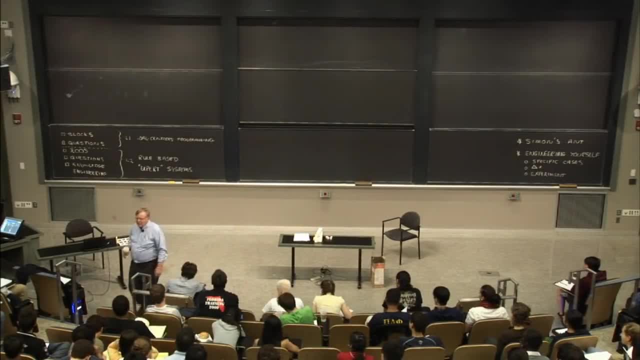 I play it for you today because I'm an engineer. I like to build stuff. I build stuff out of wood, I build stuff out of metal, I build stuff out of rocks and I especially like to write programs- I don't know. sometimes. 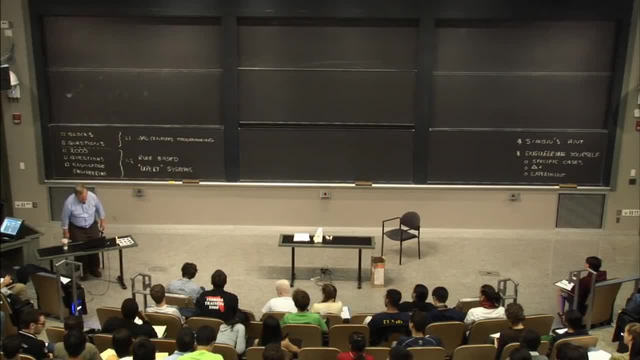 People come to me and say: I'm majoring in computer science but I don't like to write programs. I've always been mystified by that. I mean, if you want to show how tough you are, you can go bungee jumping or drive a nail through your hand or something like that. instead. 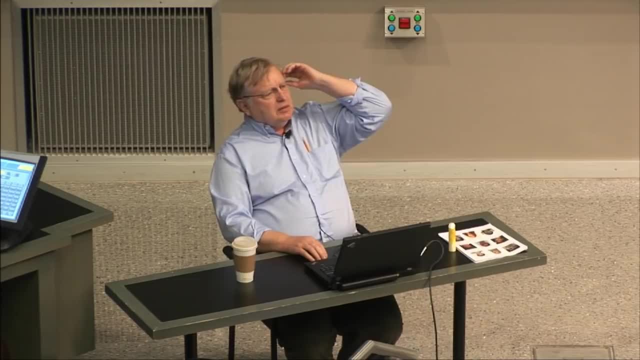 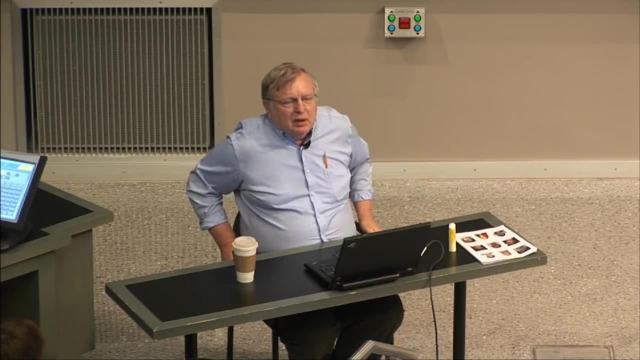 But I've written quite a few programs for demonstrating stuff in this subject. They're all written in Java, principally because I can therefore make them available to you and to the rest of the world. I can make them available to the rest of the world by way of Web Start. 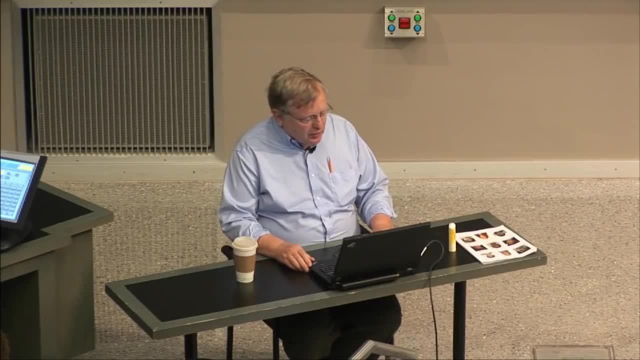 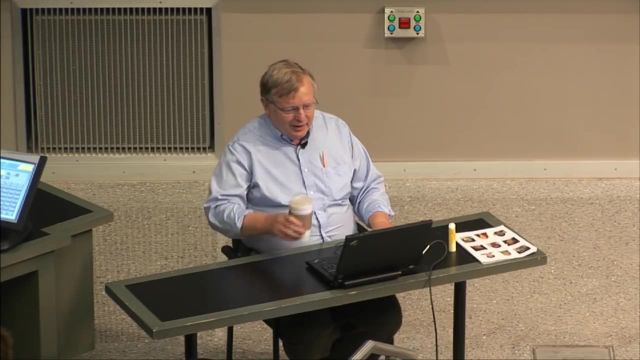 A few weeks ago I was monkeying around with the system and broke the version on the server, and within 15 minutes I got an email from somebody in the depths of Anatolia complaining about it and asking me to bring it back up. 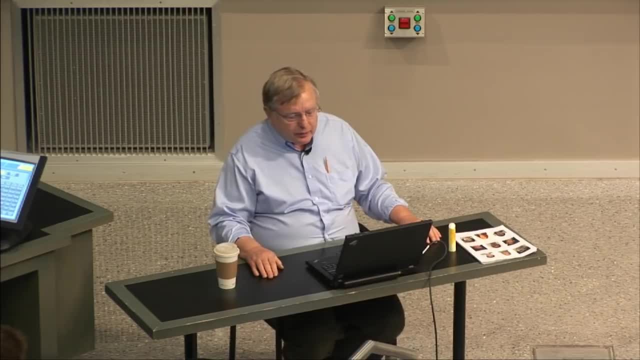 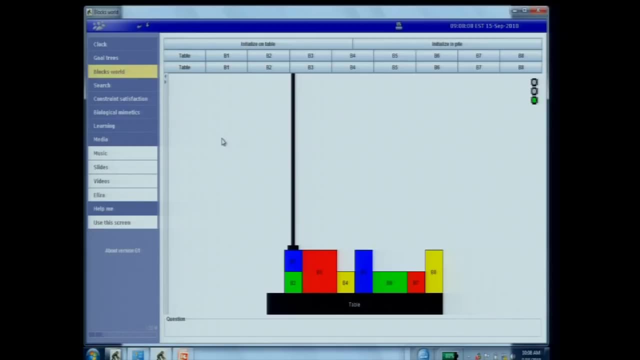 This particular program is patterned after an early AI classic And it was the business end of a program written in Java, And it was the business end of a program written in Java, written by Terry Winograd, who became and is a professor of. 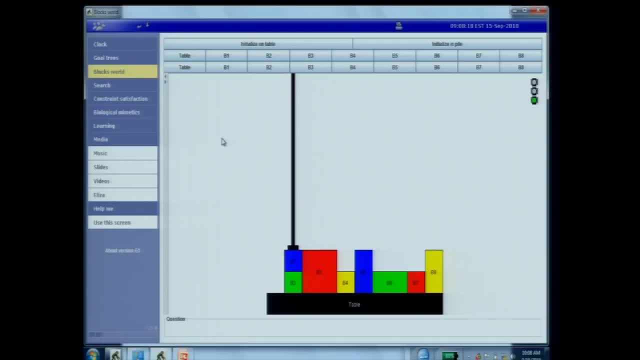 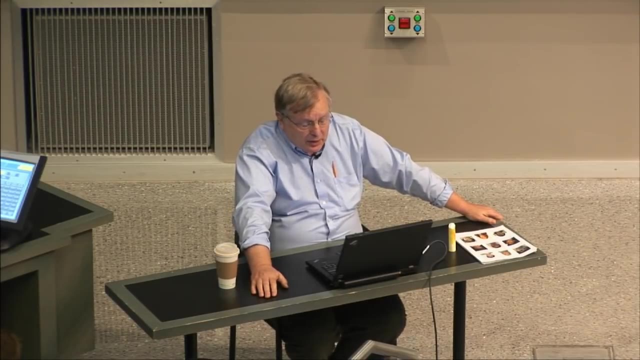 computer science at Stanford University, which is on the West Coast. for these reasons, on the strength of his work on the natural language front end of this program. But the natural language part is not what makes it of interest for us today. It's more the other kinds of stuff. 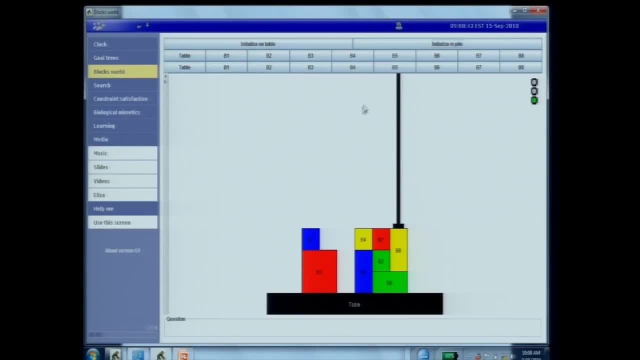 Let's pile these things up. Now I'm going to ask to do something. maybe put B2 on top of B7. Not bad. How about B6 on B3?? This program's kind of clever. Let me do one more. 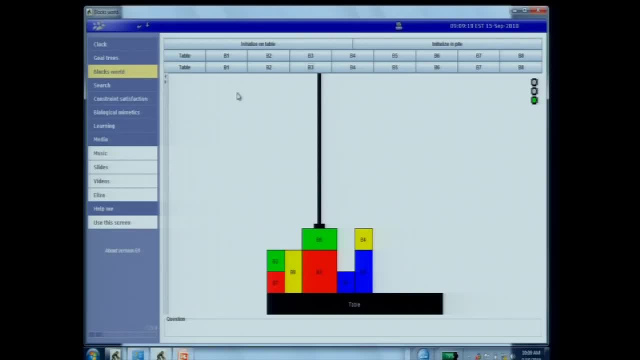 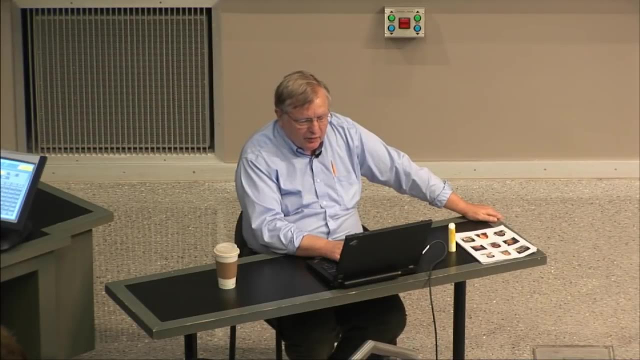 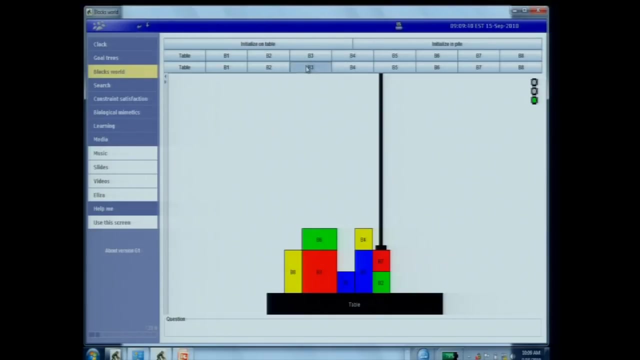 Let's put B7 on B2.. OK, now let's see. Maybe B5 on B2? Well, B4 on B3 first, maybe. No, I must have clicked the wrong button. OK, let's put B4 on B1.. 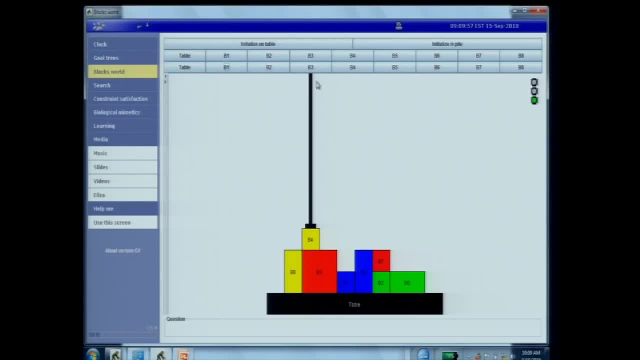 Ah, My mouse keeps getting out of control. Now let's put B1 on B2.. This is an example I'm actually going to work out on the board. Oh, I see My touchpad accidentally got activated. B1 on B2.. 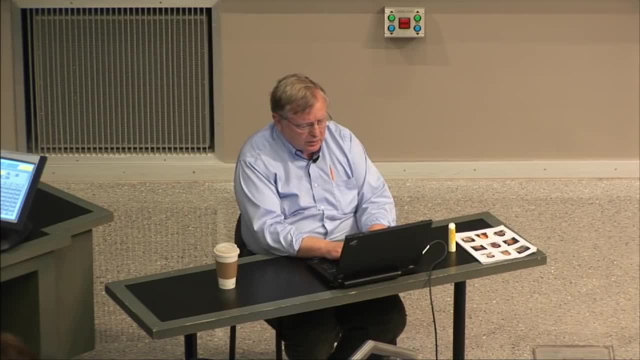 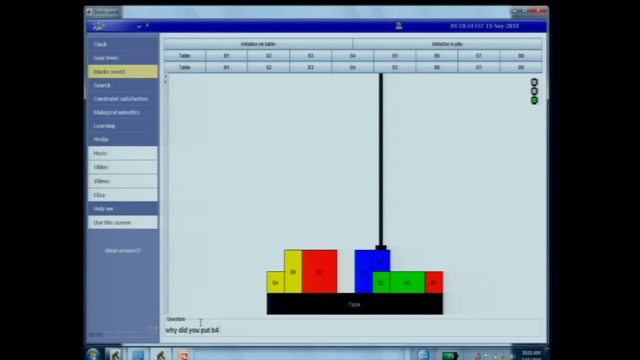 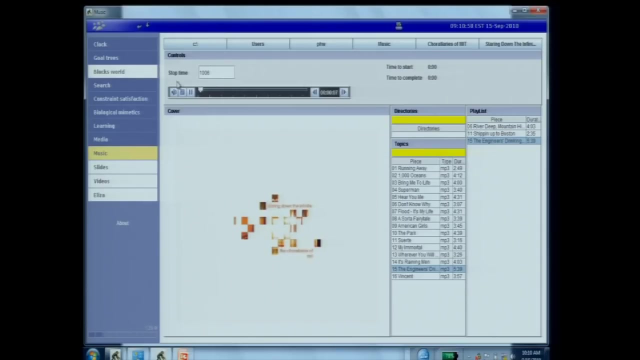 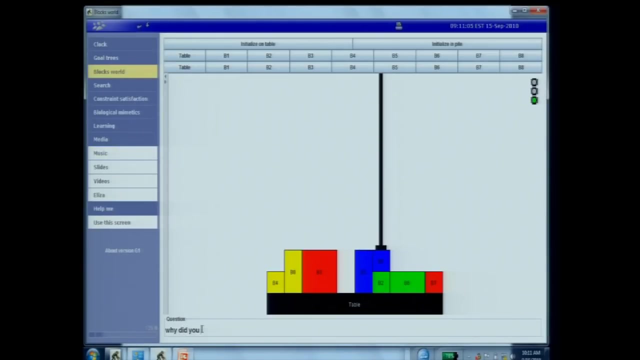 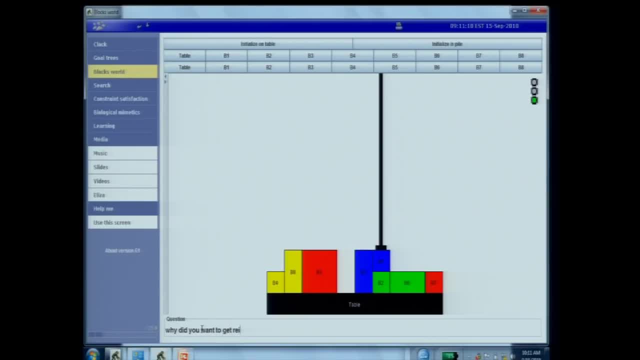 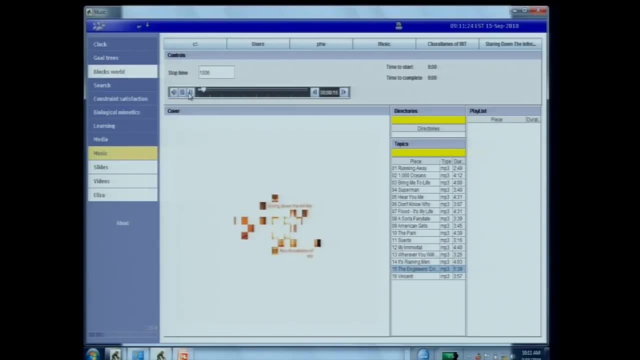 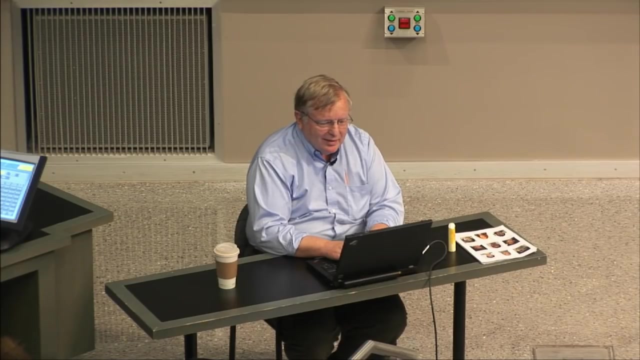 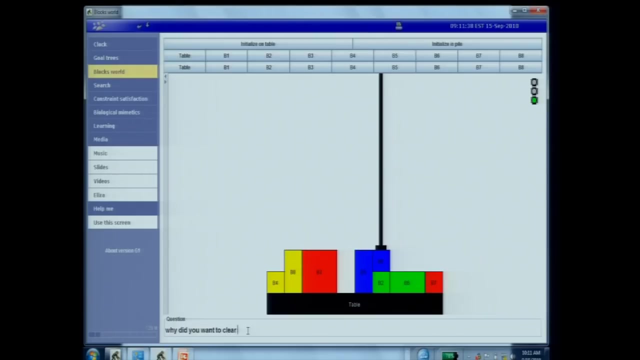 Why did you want to get rid of B4?? OK, I want to clear the top, Thank you, Thank you. So what happens when you use software? you write yourself: Why, Why, Why did you want to clear the top of B2?? 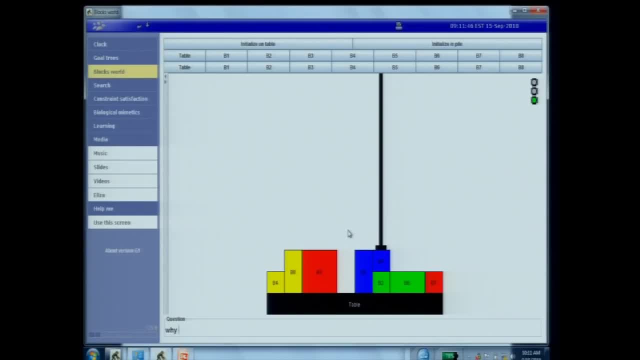 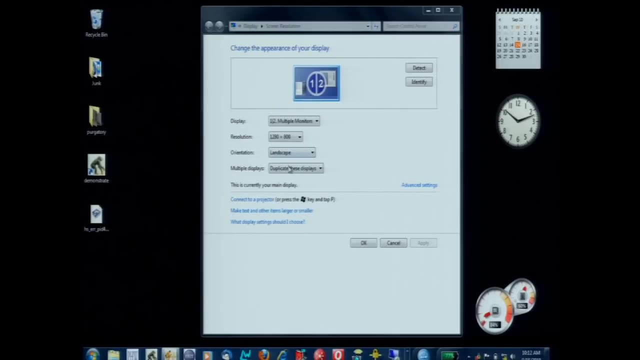 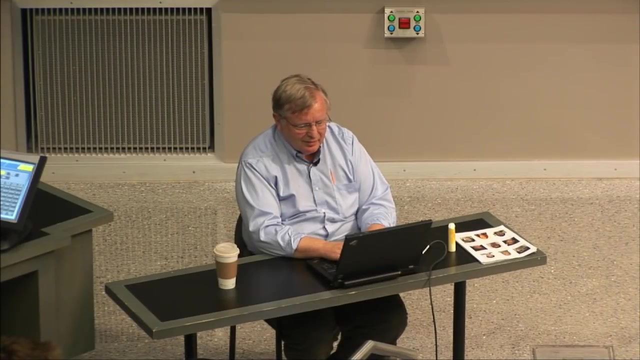 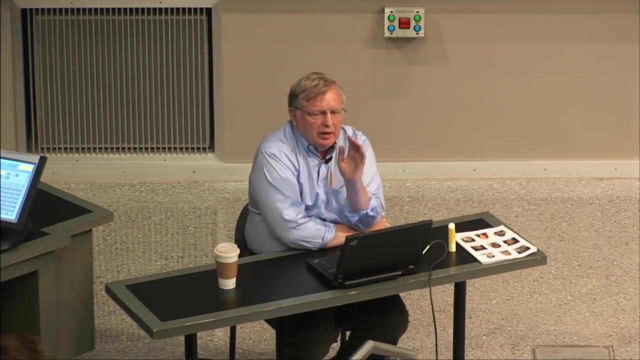 Did I do that? Why did you clear the top of B1?? OK, It's haunting me, Oh, it's haunting me. yeah, It's. the drinking song is easily offended, I guess. But I won't, uh, I won't develop that scenario again. 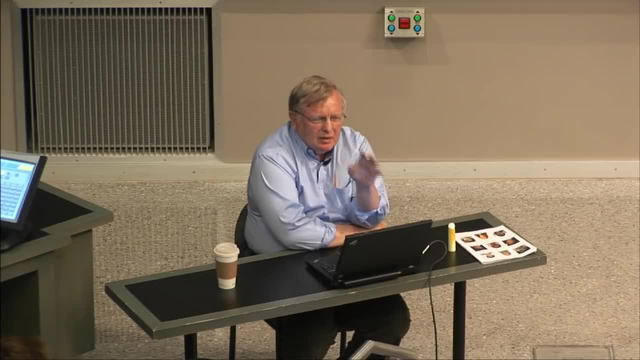 Uh, what I wanted to show you is that this program looks like it's kind of smart and it somehow can answer questions about its own behavior. Have you ever written a program that's answered questions about its own behavior? Probably not, Would you? would you like to learn how to do that? 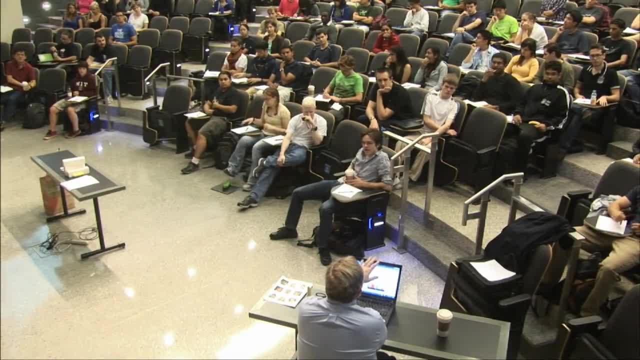 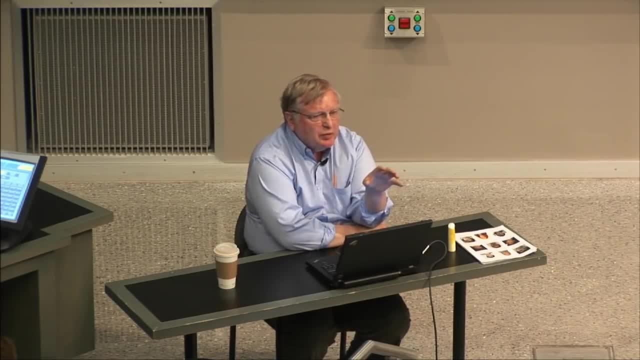 OK, So by the end of the hour, you'll be able to write this program and many more like it that know how to answer questions about their own behavior. There have been tens of thousands of such programs written, but only by people who know. 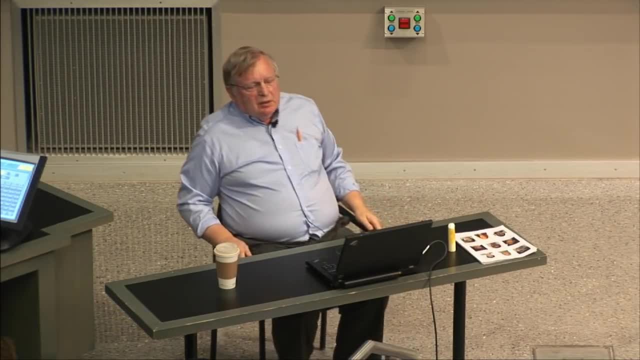 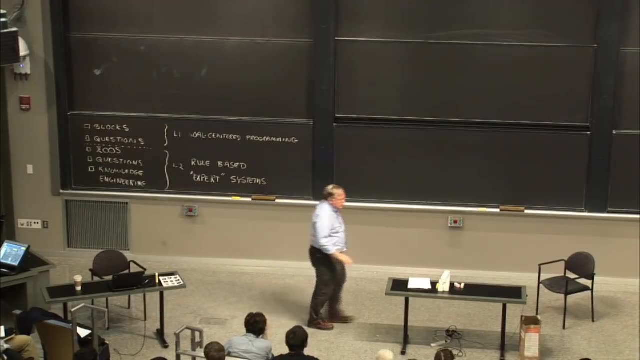 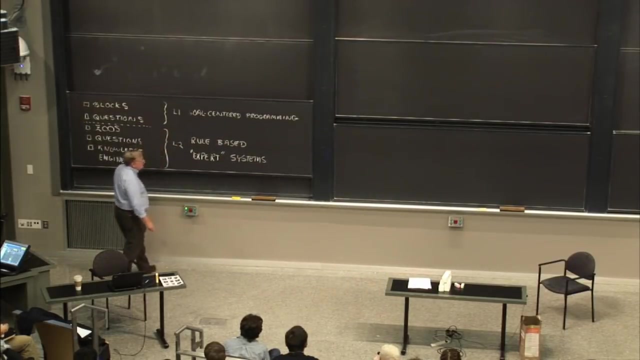 the stuff I'm going to tell you about right now. OK, So what I want to do is I want to start by taking this program apart on the board and talking to you about the modules, the subroutines that it contains. So here it is. 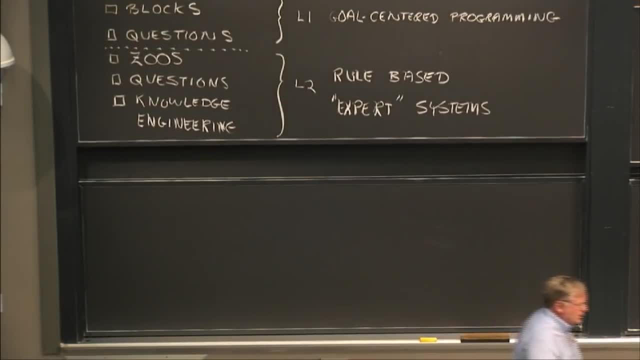 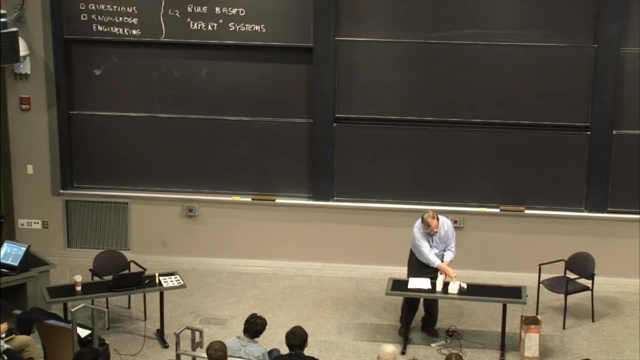 The first thing we need to think about here are some blocks. What hap? what has to happen if I'm going to put the bottom block on the larger block? Well, first of all I have to find space for it, Then I have to grasp the lower block. 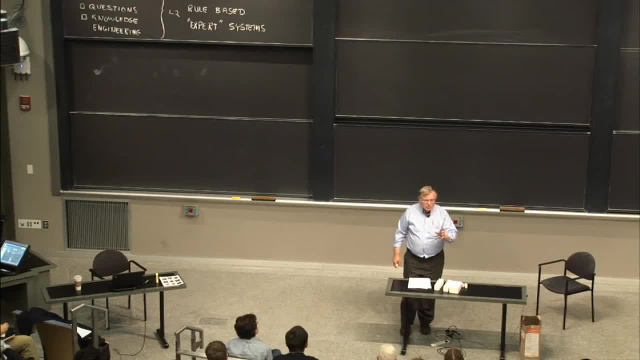 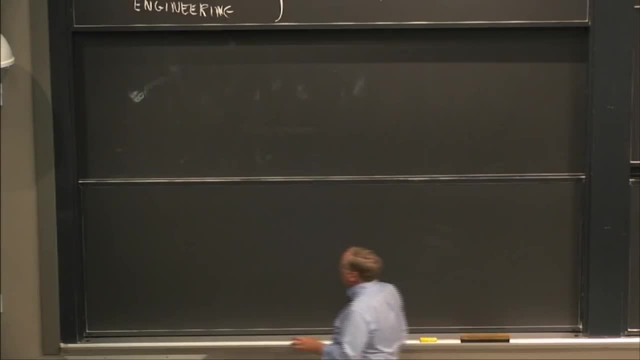 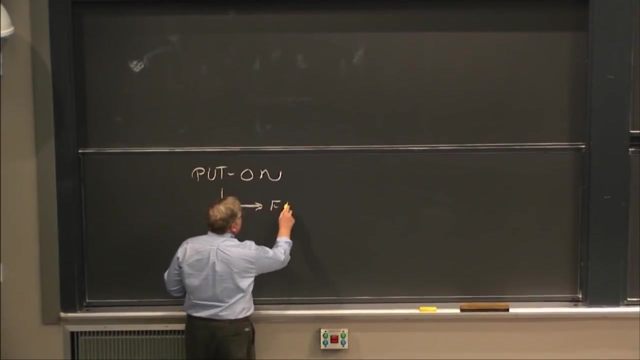 Then I have to move it, Then I have to ungrasp it. So those are four things I need to do in order to achieve what I want to do. So therefore, I know that the put-on method has four pieces. It has to find space on the target block. 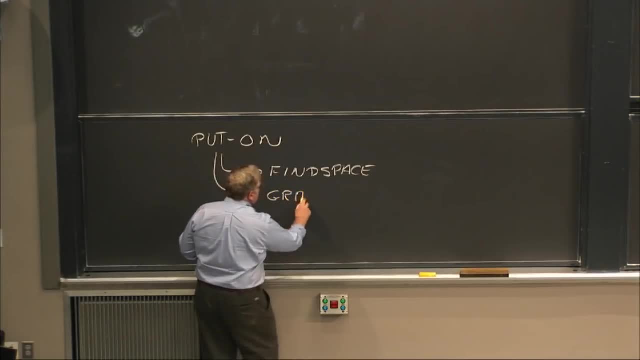 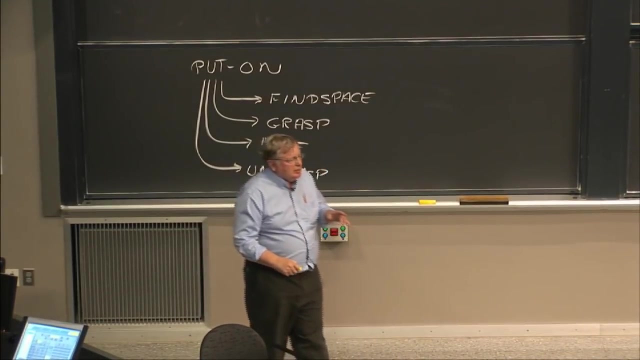 It has to grasp the block that has been commanded to move, Then it has to move And then it has to ungrasp. But taking hints from some of the questions that it did answer- before I got haunted by the music, taking our cue from that, we know that in order to grasp something, 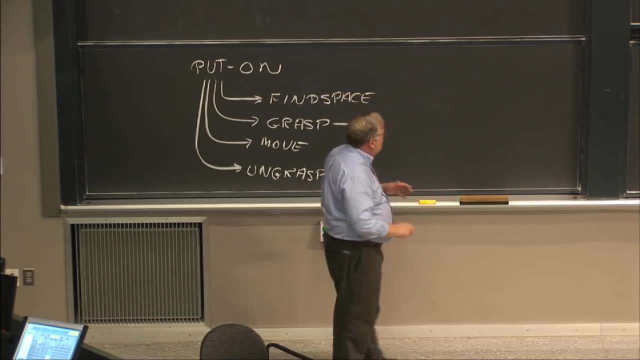 in this particular world, you can't have anything on top of it, So grasp, therefore, may call clear top in order to get stuff off from the target object, And that's it. It may happen in an iterative loop, because there may be. 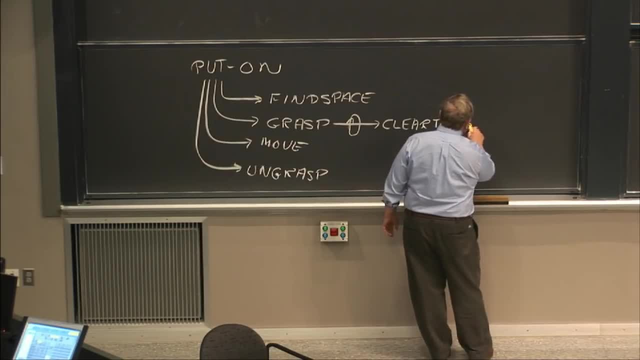 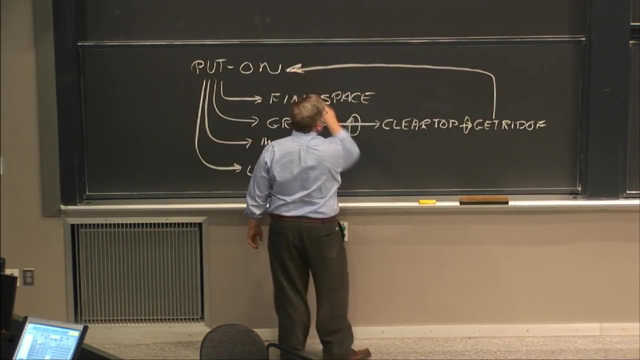 several things on top. And how do you get rid of stuff? Well, by calling getRidOf, And that may go around the loop several times. And then the way you get rid of stuff is by calling putOn. So that gives us recursion. 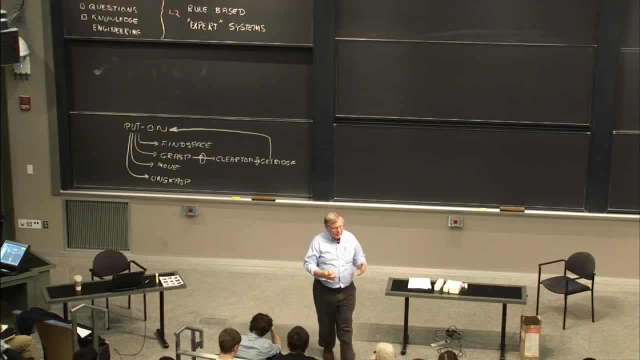 And it's from the recursion that we get a lot of the apparent complexity of the program's behavior when it solves a problem. Now, in order to find space, you also have to call getRidOf, So that's where I meant to put this other iterative loop not. 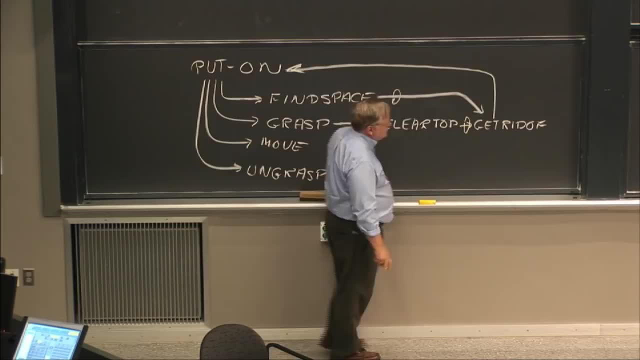 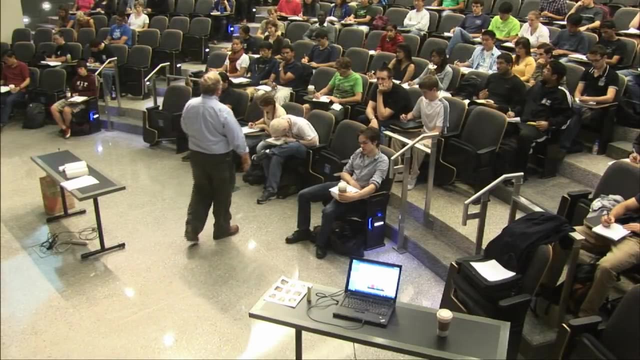 down here. Clear top has got the iterative loop inside of it. So that's the structure of the program. It's extremely simple, And you might say to me: well, how can you get such apparently complex-looking behavior out of such a simple? 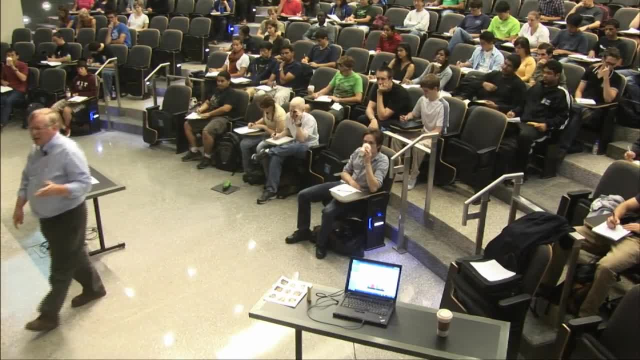 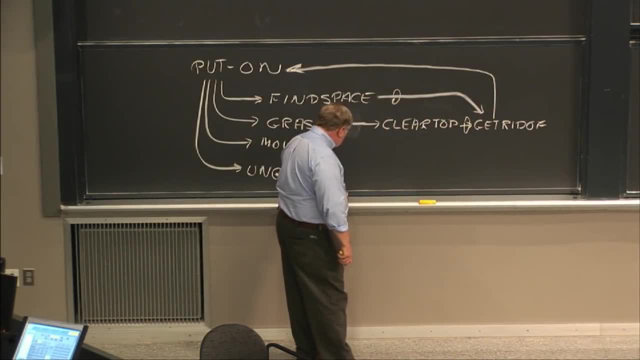 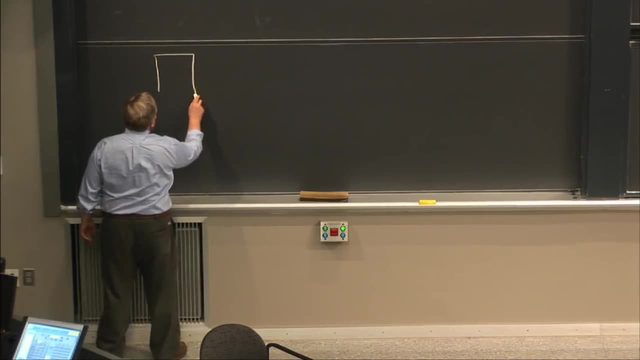 program a legitimate question. But before we tackle that one head on, I'd like to do a simulation of this program. I want a very simple Blocks problem, And it's the one I almost showed you, but it goes like this. Here's b1.. 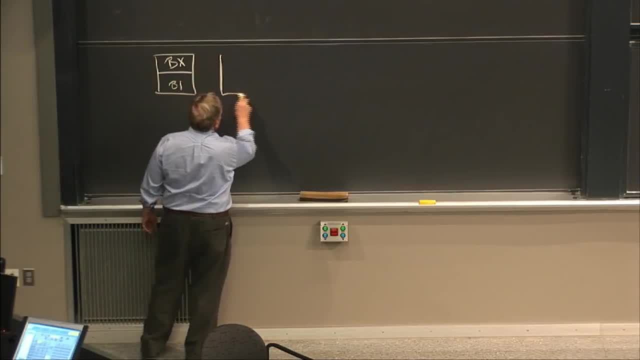 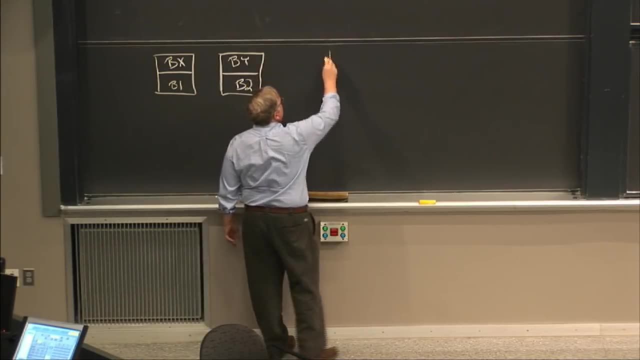 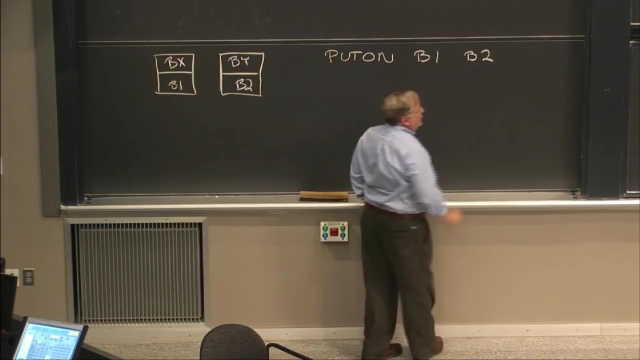 We'll call this bx, because I'd forgotten its name. Here's by And here's b2.. And the task is to put b1 on b2.. B1 on B2. And according to our system diagram, that results in four. 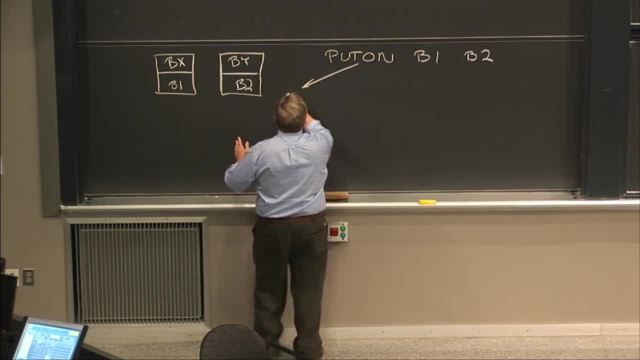 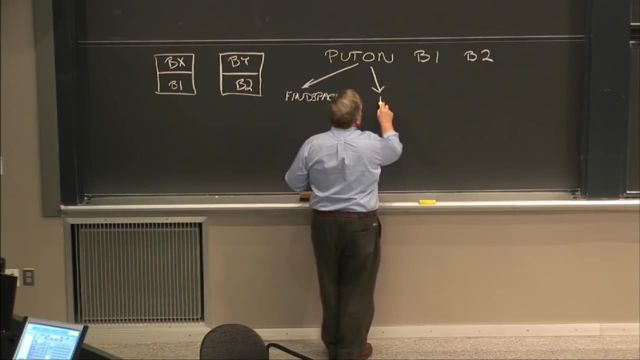 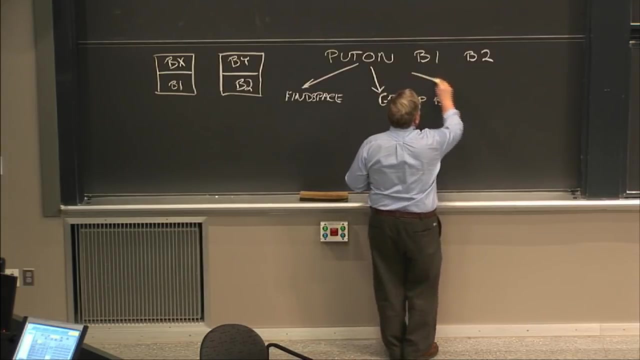 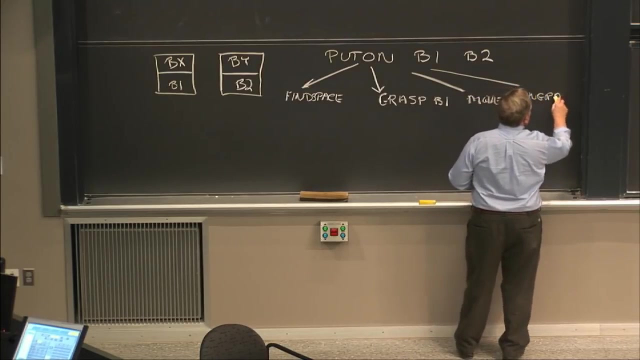 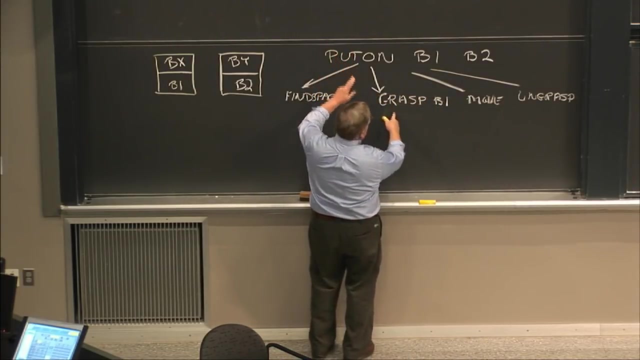 calls to subroutines. We have to find space, We have to grasp B1. We have to move And then we ungrasp. Now, the way we grasp something is the first thing we have to do is clear off its top. 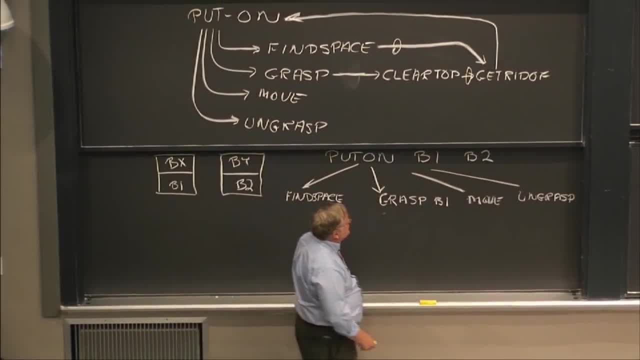 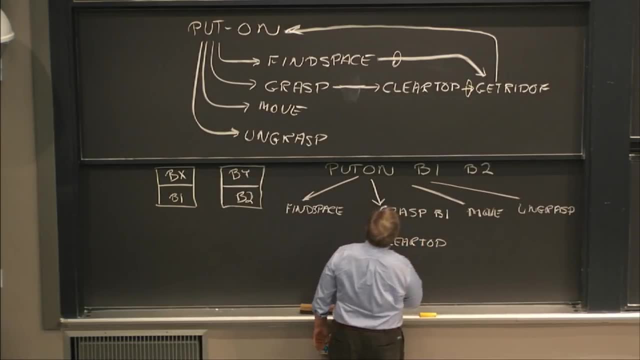 So grasp calls clear top and clear top in turn calls get rid of. And let me see, Let me keep track of these. This is clearing the top of B1, and this is getting rid of Bx. And the way we get rid of Bx is: 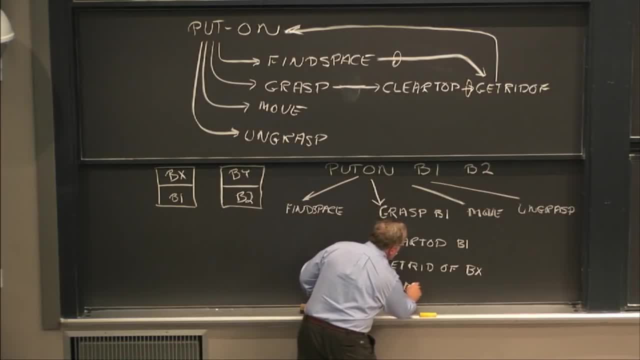 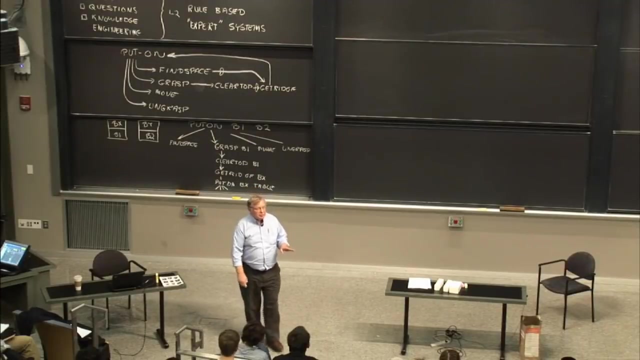 by putting Bx on the table And then that in turn causes calls to another find space, another grasp, another move and another ungrasp. So that's a little trace of the program as it works on this simple problem. 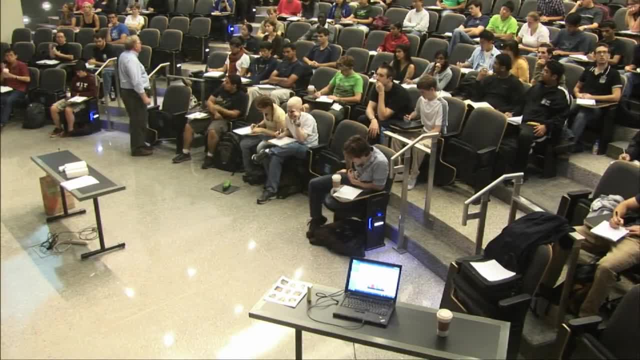 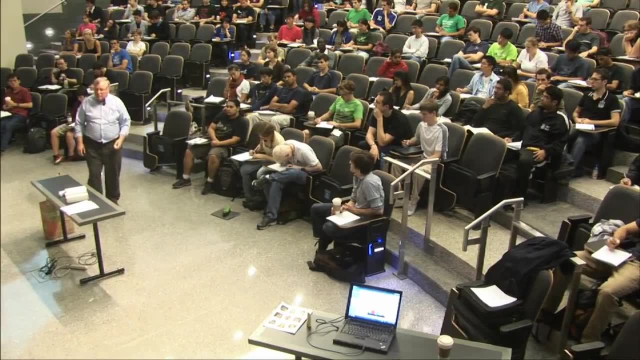 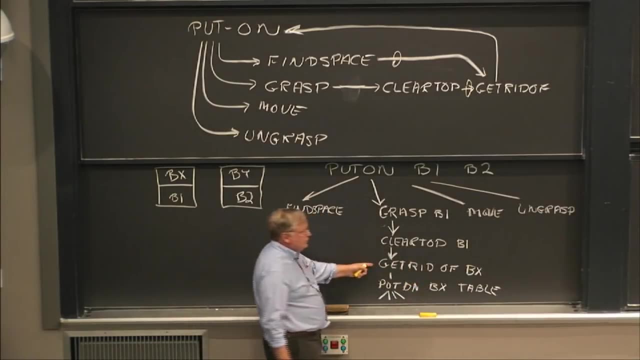 So how does it go about answering the questions that I demonstrated to you a moment ago? It must do that by using this trace. So how, for example, does it answer the question: why did you get rid of Bx Manasa? what do you think? 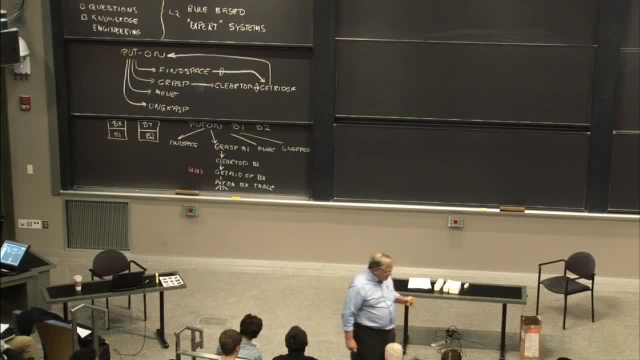 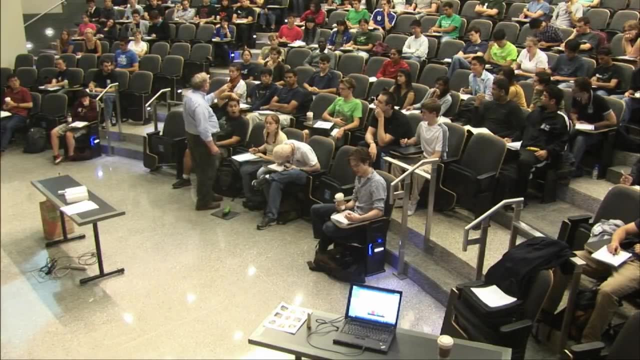 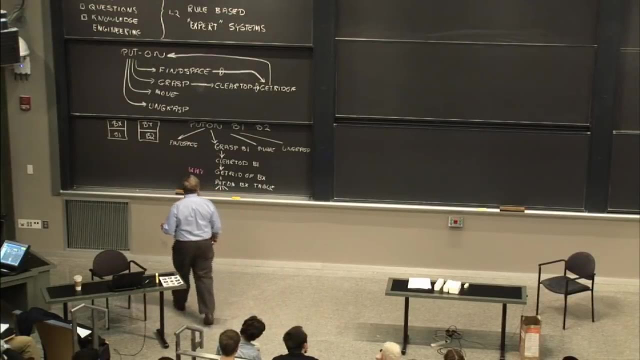 How can it answer that question? So The previous: It goes up one level and reports what it sees. So it says and said: in the demonstration I got rid of Bx because I was trying to clear the top of B1.. 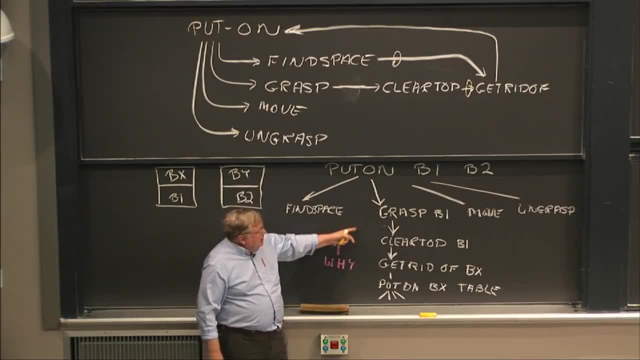 So if I were to say why did you clear the top of B1,? it would say because I was trying to grasp it. If I were to say why did you grasp B1,, it would say because I was putting B1 on B2.. 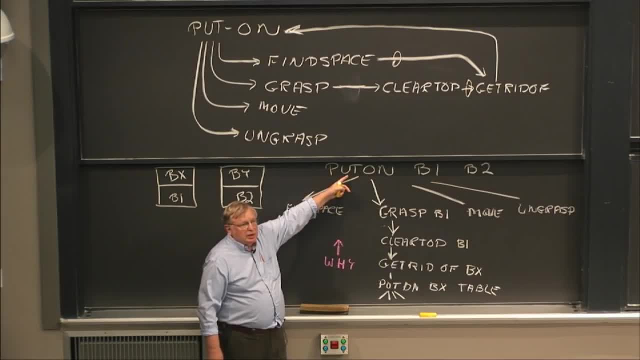 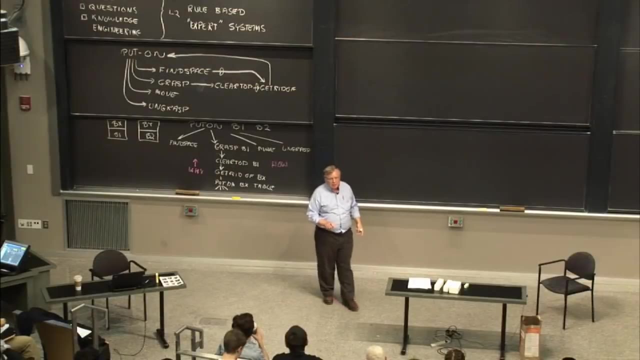 If I say why did you put B1 on B2, it would say: slavishly, because you told me to. OK, so that's how it deals with. why questions? How about? how questions? Timothy, what do you think about that one? 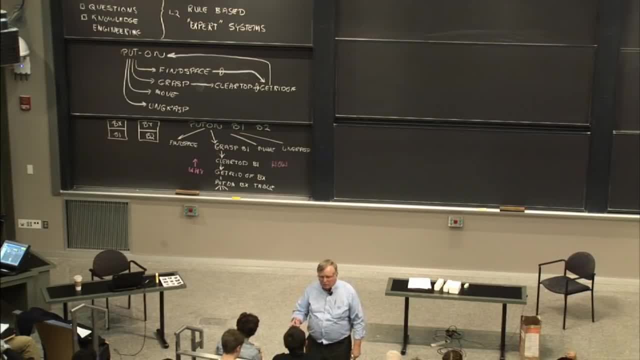 How would it go about answering a question about how you did something? Do you have a thought? Yeah, I would think about what I was trying to accomplish. Yeah, but how would the program do that? We know that answering why questions makes it go up one. 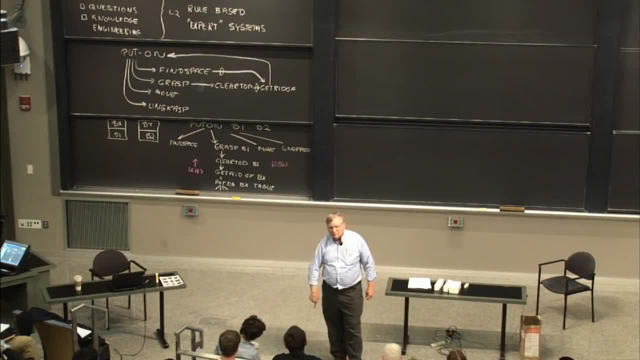 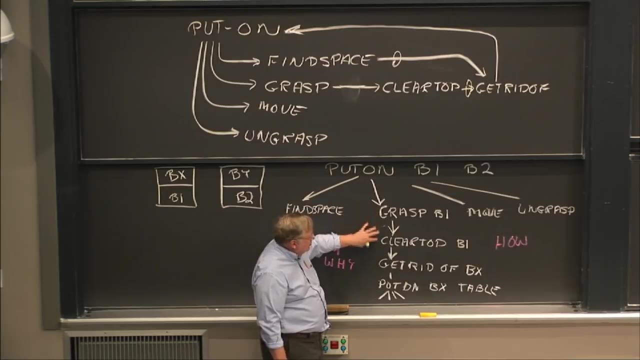 level. How does it answer a? how, question, Sebastian, you go down one level. So if you start off all the way up here with a put-on, it will say, oh well, I did these four things. If you say, why did you grasp B1, it will say because I. 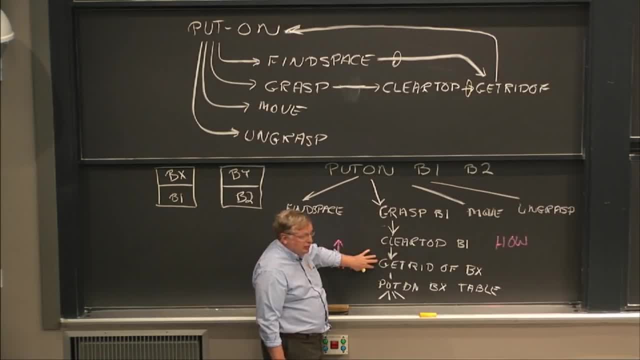 was trying to clear its top. Why did you clear its top? Because I was trying to get rid of it. Why were you trying to get rid of it? Because I was trying to put it on the table. So that's how it answers. how questions? by going down in. 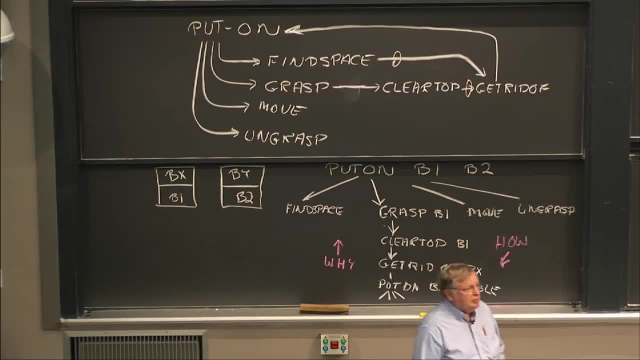 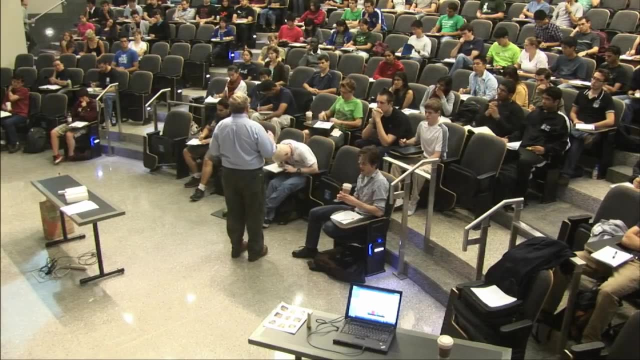 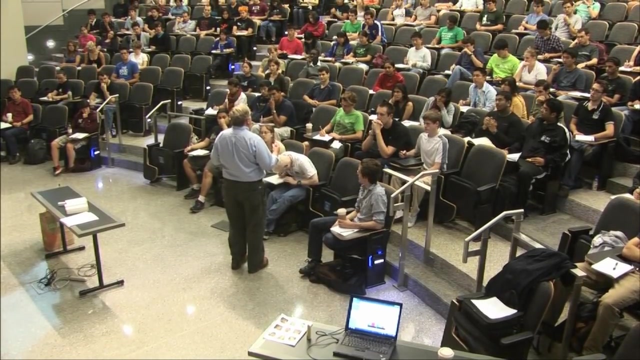 this tree, in this trace of program action, so as to see how things are put together. What are these things that are being put together? What's the word I've been avoiding, so as to bring this to a crescendo? What are these objectives, these things it wants to do? 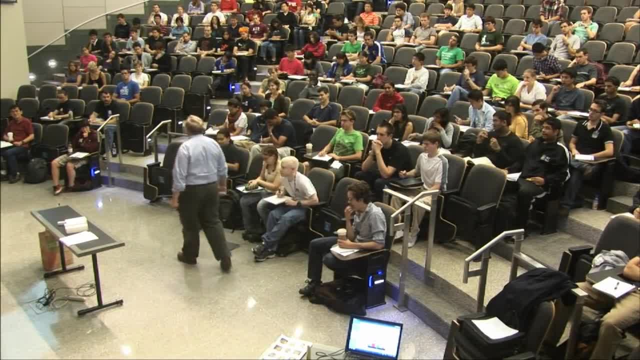 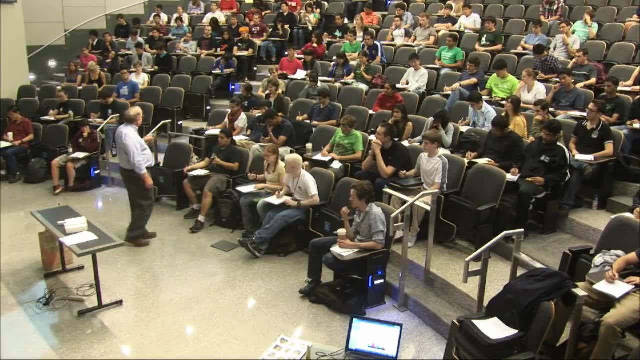 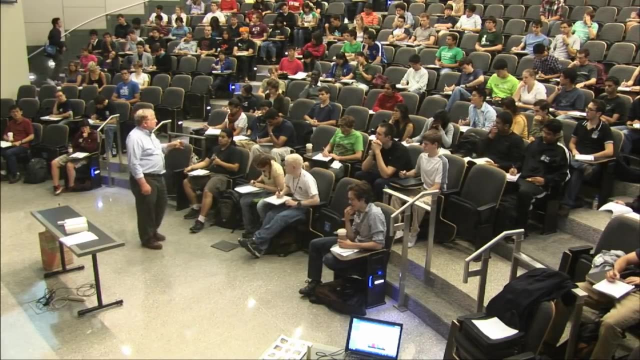 They're goals. So this thing is leaving a trace, which is a goal tree. Does that sound familiar? Three days ago, we talked about goal trees in connection with integration, So this thing is building a goal tree, also known as an AND-OR tree. 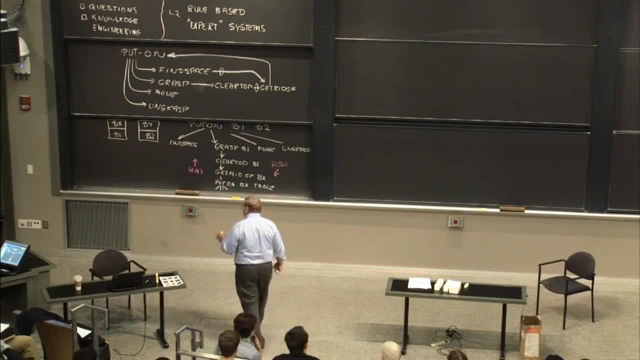 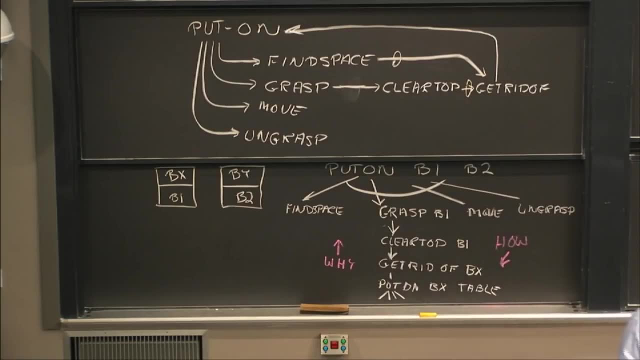 So this must be an AND tree. And if this is an AND tree, are there any AND nodes? Sure, there's one right there. So do you think, then, that you can answer questions about your own behavior as long as you build an AND-OR tree? 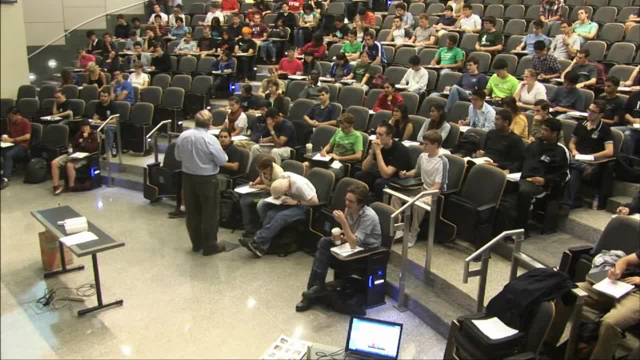 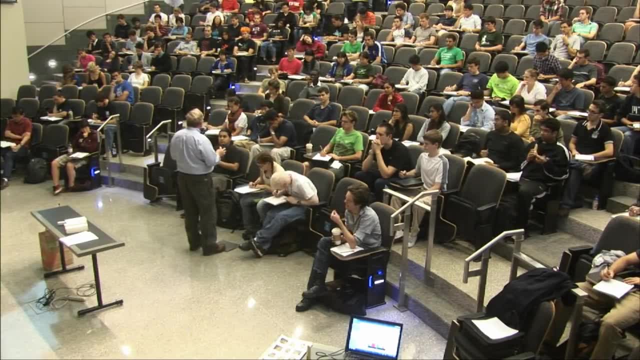 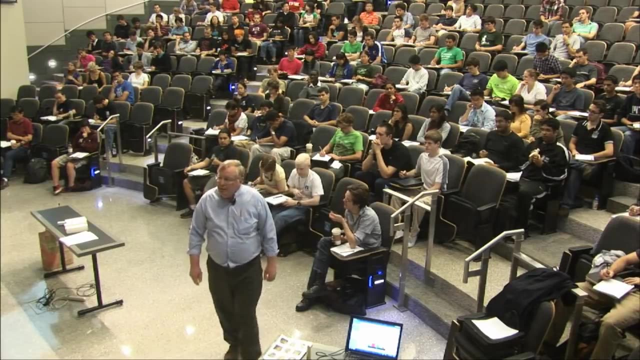 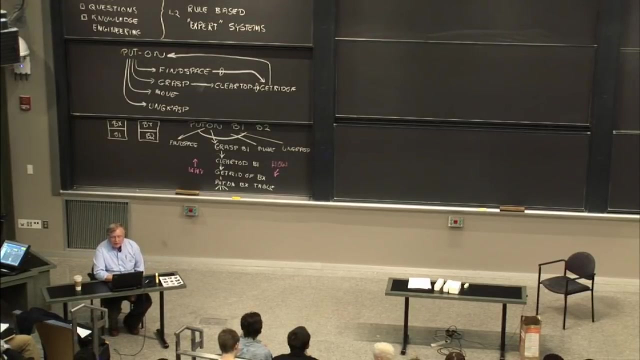 Sure. Does this mean that the integration program could answer questions about its own behavior? Sure, because they both build goal trees, And whenever you've got a goal tree you can answer certain kinds of questions about your own behavior. So let me see if, in fact, it really does build itself a goal. 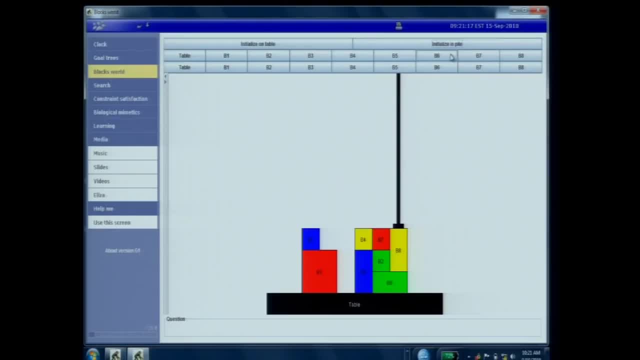 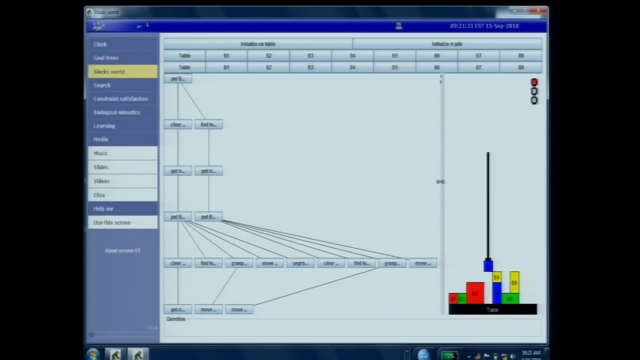 tree as it solves problems. So this time we'll be talking about an AND-OR tree. This time we'll put B6 on B3.. This time we'll watch it develop its goal tree. So, in contrast to the simple example, I was working on the 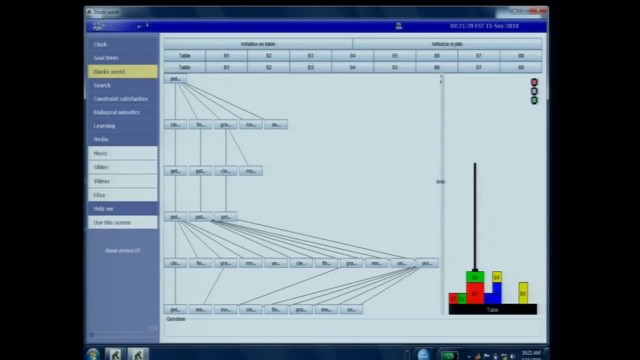 board. this gets to be a pretty complicated goal tree, But I can still answer questions about behavior, For example, I could say: why did you build this? Why did you build this? Why did you put B6 on B3, as you told me to? 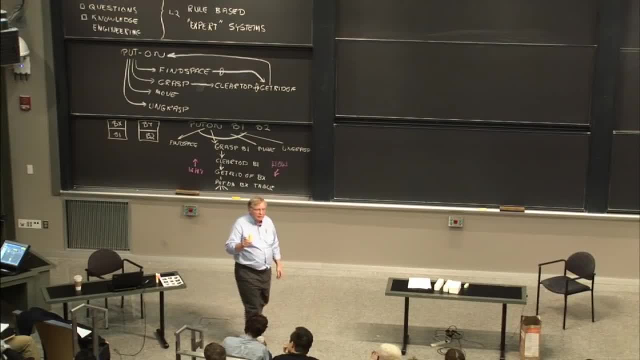 So the complexity of the behavior is largely a consequence not of the complexity of the program in this particular case, but the building of this giant goal tree is a consequence of the complexity of the problem, And this brings us rather early on to one of the gold. 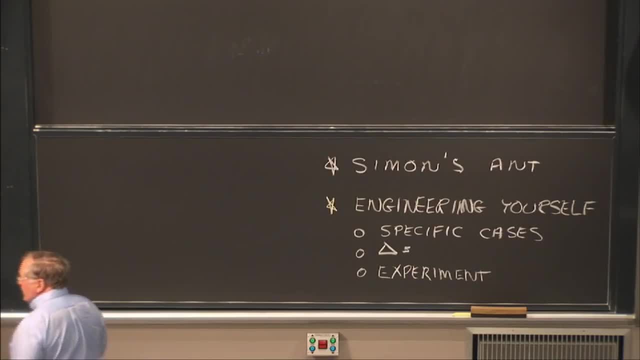 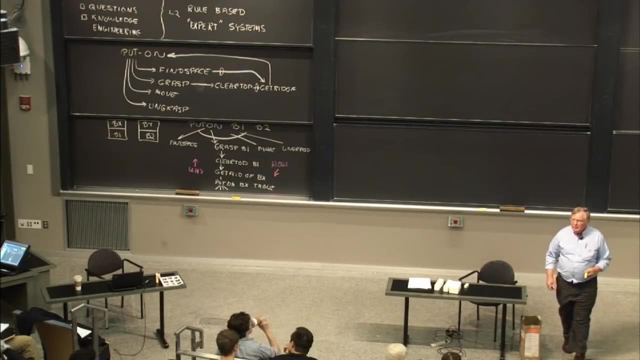 star ideas of today. And this gold star idea goes back to a problem that we've solved And it goes back to a lecture given in the late 60s by Herb Simon, who was the first Nobel Laureate in the pseudo Nobel Prize for Economics. 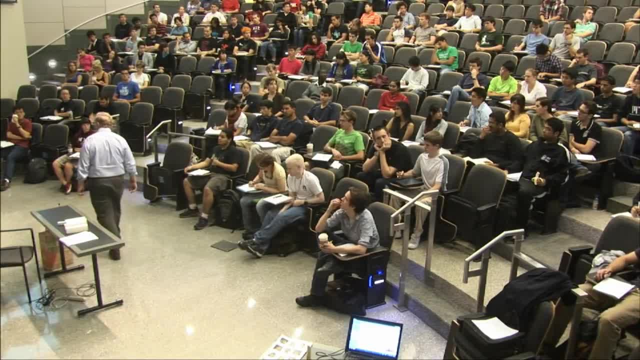 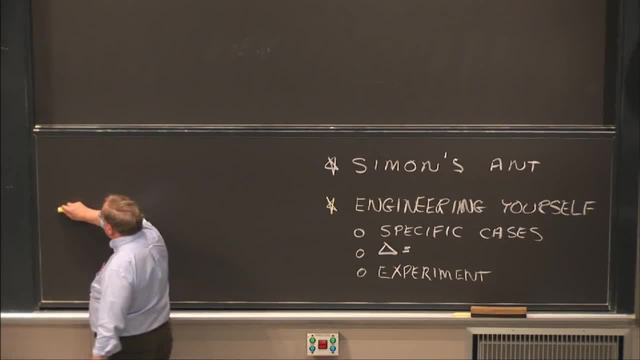 Is that right, Bob? Was he the first? Yeah, he was the first winner of the Nobel Prize- pseudo Nobel Prize- in economics, And in this lecture, which was titled Science is the Artificial, he said: imagine that you're looking on a beach. 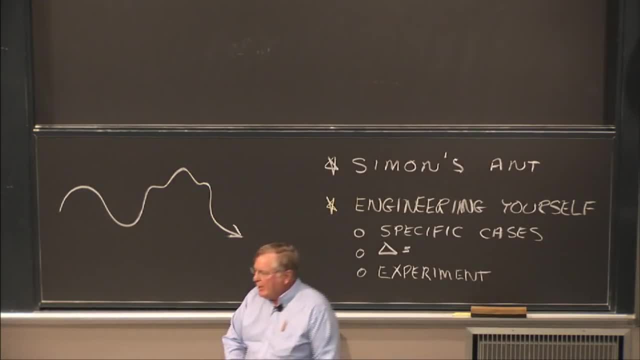 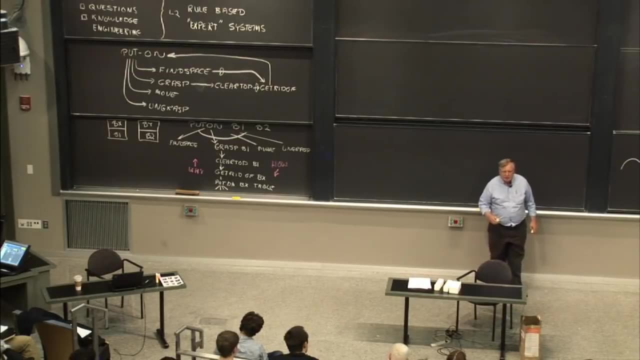 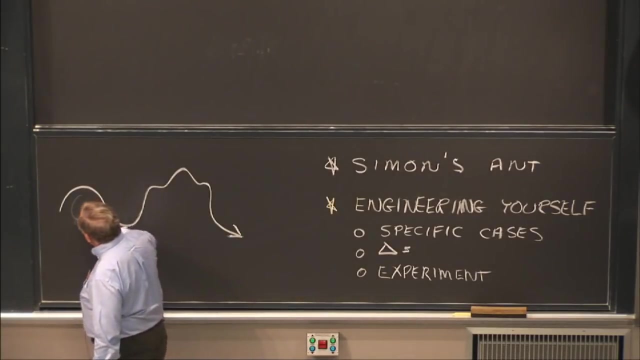 at the path of an ant And he said: well, you know, The path of the ant looks extremely complicated And you're tempted to think the ant is some kind of genius or a monster brain ant. But in fact, when you take a closer look, what you discover? 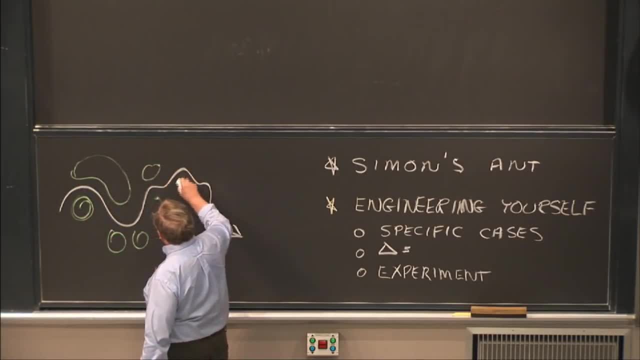 is that there are a bunch of pebbles on the beach And all the ant is doing is avoiding those pebbles on its way home. So the complexity of the behavior, said Simon, is a consequence of the complexity of the environment. 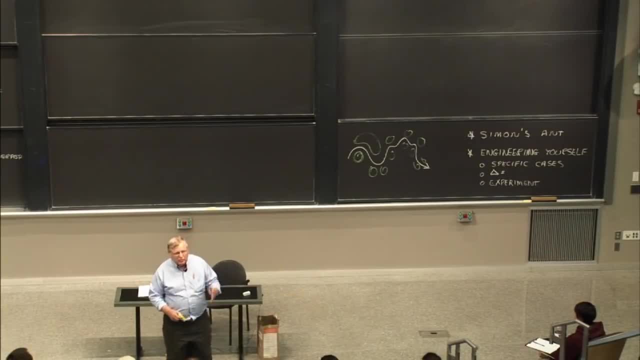 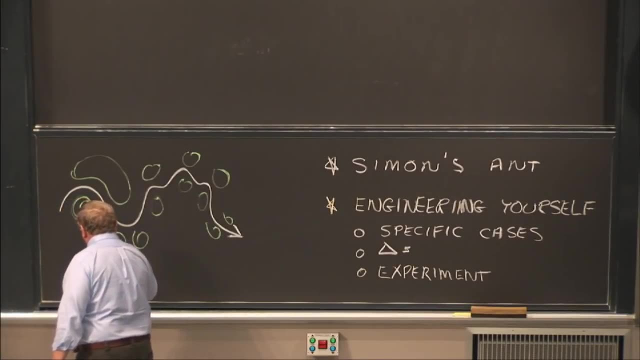 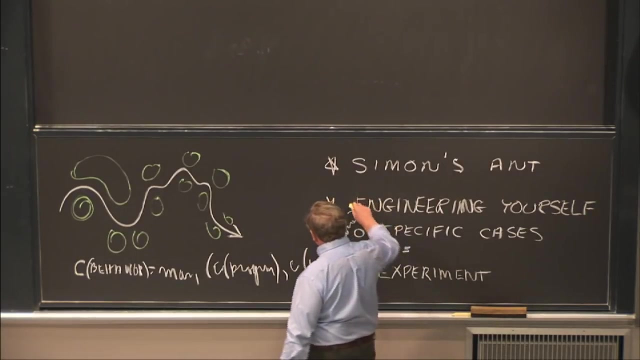 Not the complexity of the program. So that's the metaphor of Simon's ant, And what it says is that the complexity of the behavior is the max of the complexity of the program and the complexity of the environment. So that's something we'll see many times during the rest of 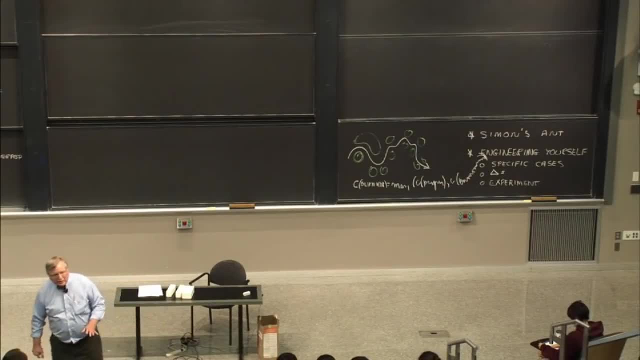 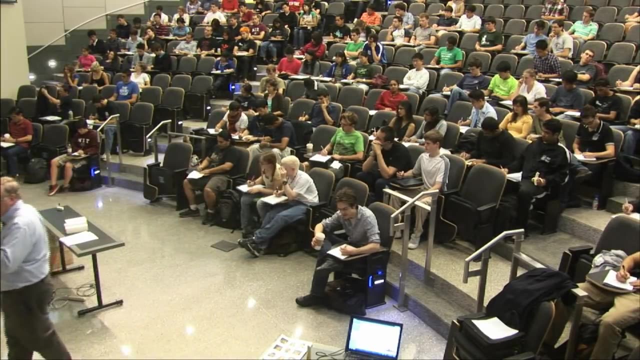 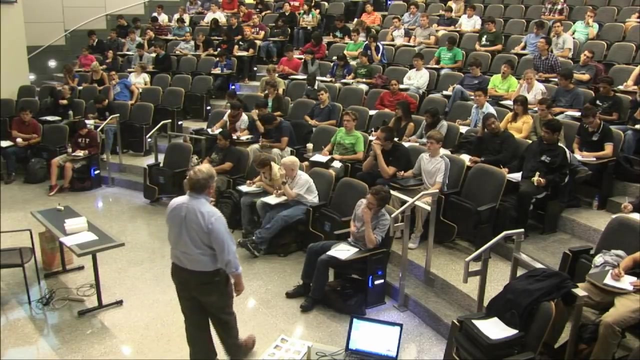 the semester. Complex behavior, simple program. You think it's going to be complicated. It turns out to be simple, Because the problem has the complexity, not the program. So that brings us to check box three in today's talk, And there's a little bit of a seam here, because now I want 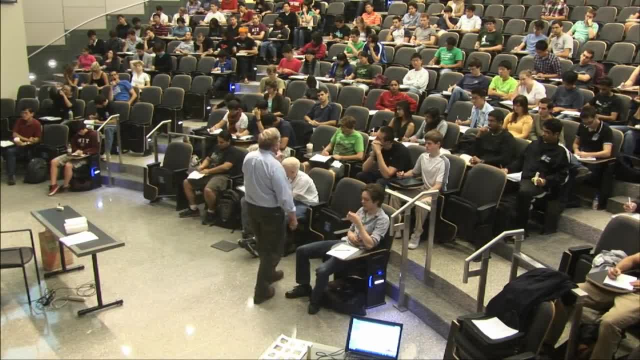 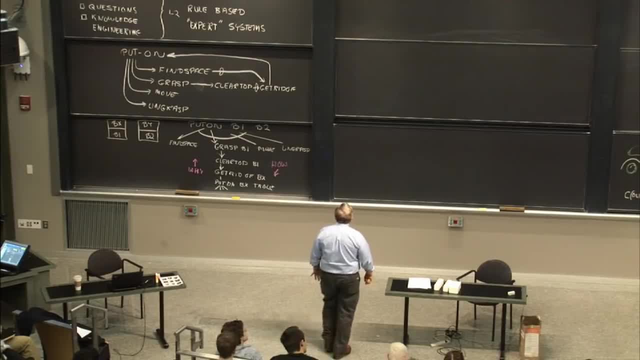 to stop talking about goal-centered programming and start talking about rule-based expert systems. Rule-based expert systems were developed in a burst of enthusiasm about the prospects for commercial applications of artificial intelligence in the mid-1980s. At that time, it was supposed lengthy articles were written. 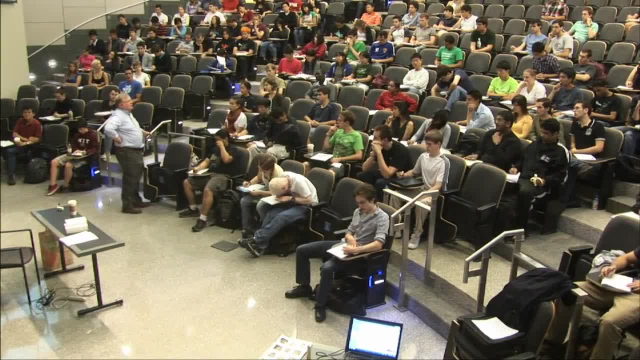 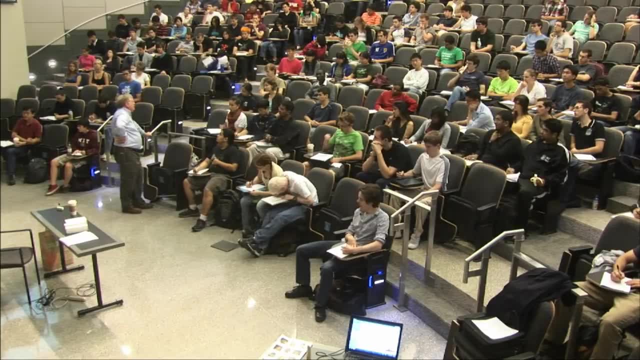 that you could account for useful aspects of human intelligence By writing all the knowledge that you need. you could use all the knowledge that you need, All the knowledge in the form of simple rules. So if this is true, then that's true. 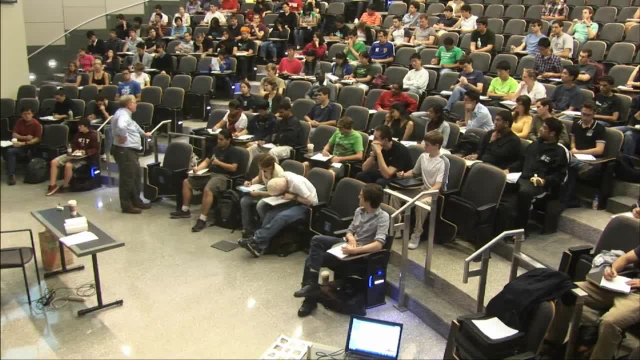 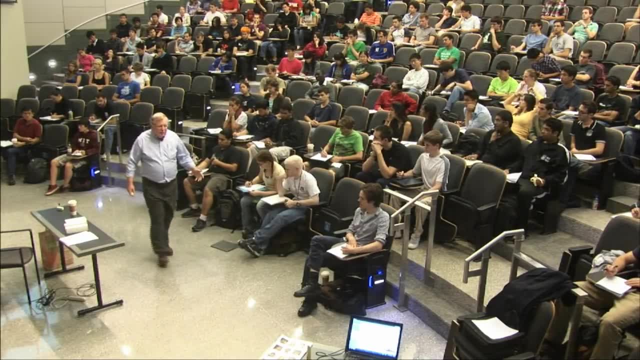 If you want to achieve this, then do that, But all the knowledge had to be encapsulated in the form of simple rules. So what might you want to do with this? All sorts of things. Thousands of these systems were written, as I indicated before. 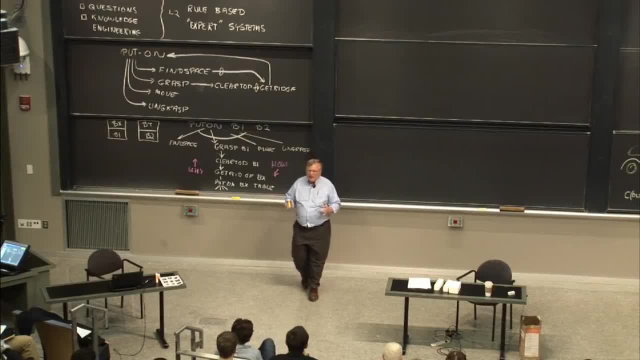 But here's an example. I'm going to work out an example having to do with identification, And this example is called. This example is patterned off of a classic program, strangely also written at Stanford, called Mycin. It was developed to diagnose bacterial. 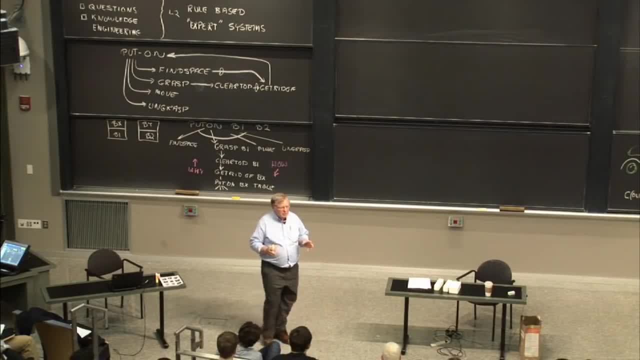 infections of the blood. So you come in, you've got some horrible disease and the doctor gets curious about what antibiotic would be perfect for your disease and starts asking you a lot of questions. So I'm not going to deal with that, because that world has. 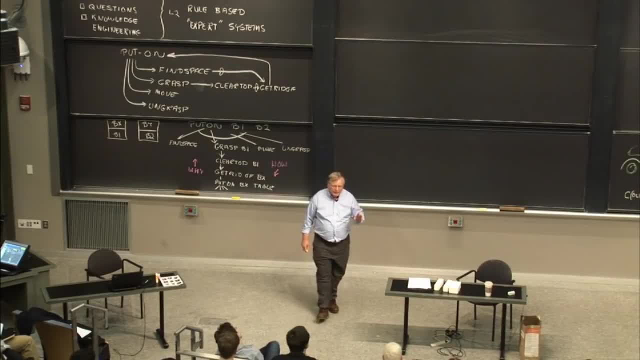 has all kinds of unpronounceable terms like bacteroides and anaerobic and stuff like that. So it's completely analogous to talk about identifying animals in a little zoo, sort of a small town type of zoo. So I'm going to suggest that we write down on a piece of: 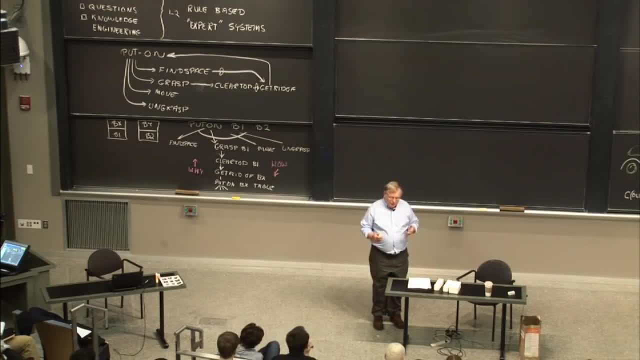 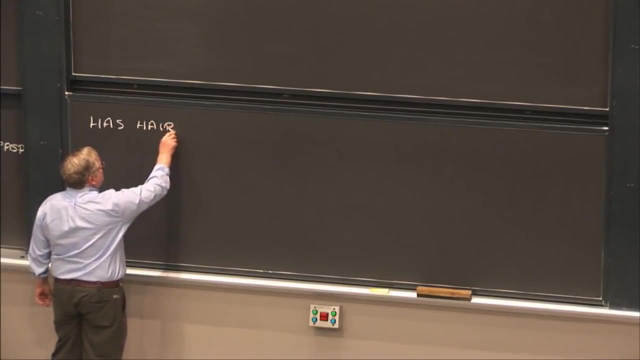 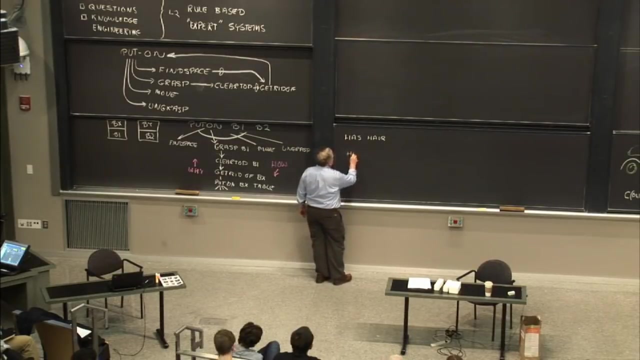 paper all the things we can observe about an animal, and then we'll try to figure out what the animal is. So I don't know What can we start with? Has hair. Then there are some characteristics of the following form: Has claws. 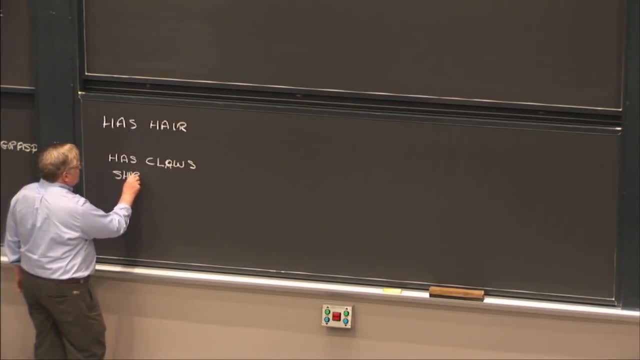 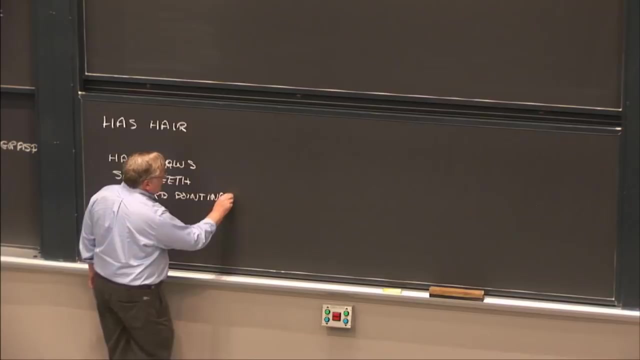 Sharp teeth And forward-pointing eyes, And these are all characteristics of carnivores. We happen to have forward-pointing eyes too, but that's more because we used to swing around in trees a lot and we needed the stereo vision and we don't have the. 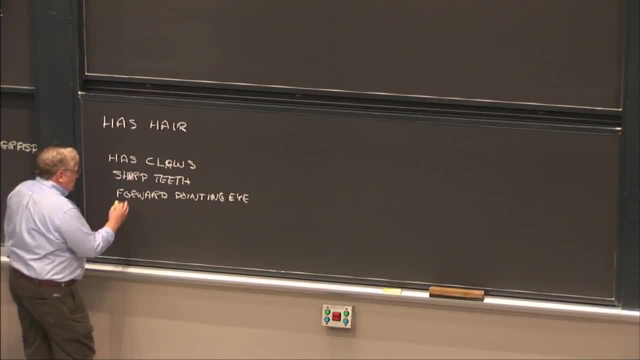 claws and the sharp teeth to go, But anyhow, those are typically characteristics of carnivores, as is eating meat, And this particular little animal we're looking at has also got spots, and it's very fast. What is it? Oh well, everybody says it's a cheetah. 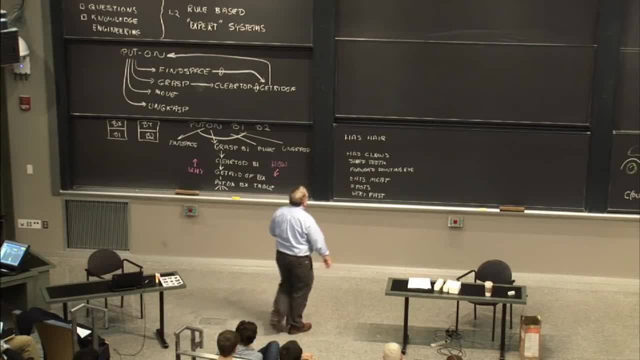 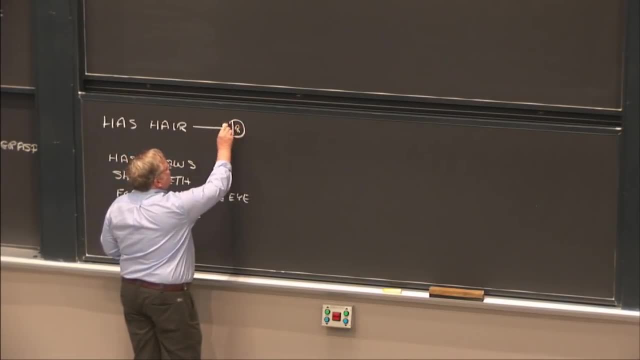 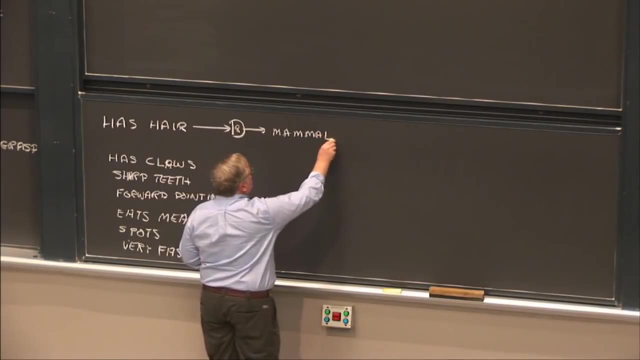 Let's see how a program would figure that out. Well, a program might say: let's see If it has hair. then rule one says that that means it must be a mammal. We can imagine another rule that says: if you have sharp. 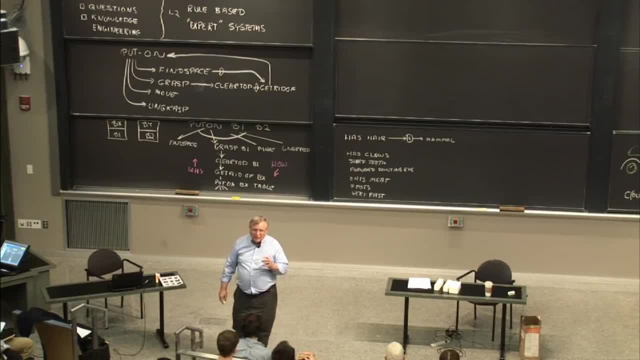 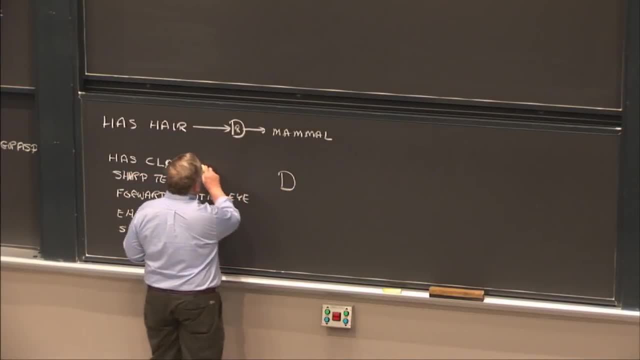 claws, sharp teeth and forward-pointing eyes. then you're a carnivore, And I'm using sort of hard-to-understand rules, but I'm using some hardware notation here. That's an AND gate right, So that means that we have to have all of these. 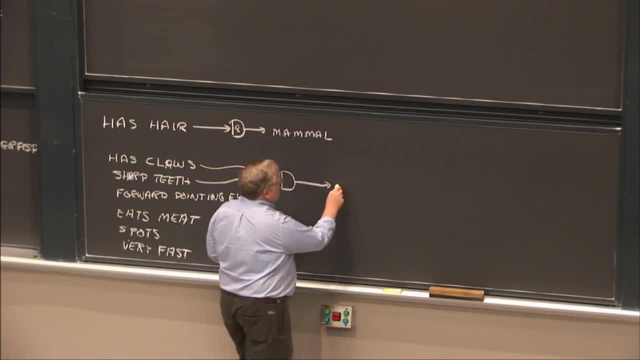 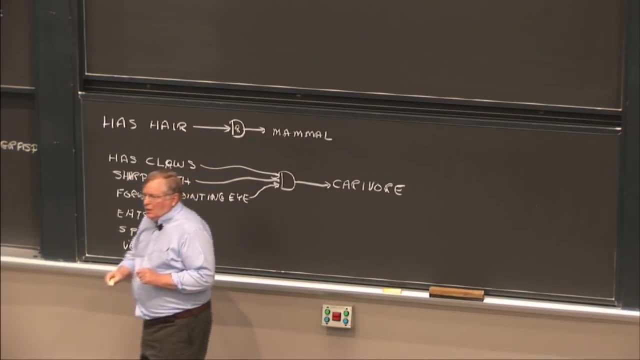 characteristics before we will conclude that the animal is a carnivore. Now this animal has been also observed to eat meat, So that means that we've got extra evidence that the animal is carnivorous. And now, because the animal is a mammal, there are a lot of animals that are carnivorous. They can't eat meat. They can't eat meat. There are animals that eat meat. That's a whole lot of animals, But that's not carnivorous. All right, let's go over here. If the animal was carnivorous, if we could just see the animal. 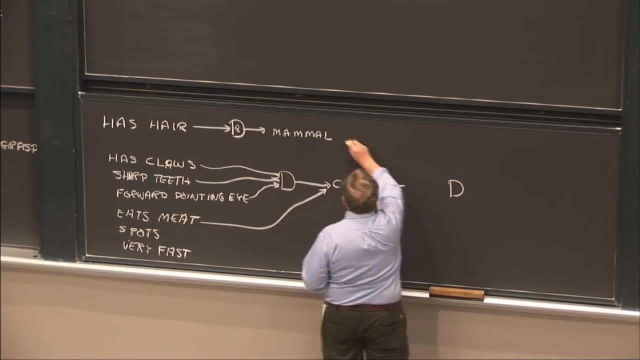 eating meat. what is that carnivore? If the animal was carnivore, they would eat. a use of meat is a mammal and a carnivore and it has spots and it's very fast. then the animal is a cheetah. 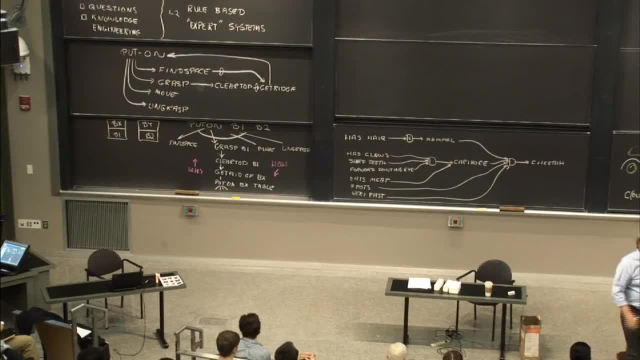 I hope all of our African students agree that that must be a cheetah. It's a small zoo. I mean, if it's a big zoo, who knows what it is? It's probably got some unpronounceable name. There are other possibilities. 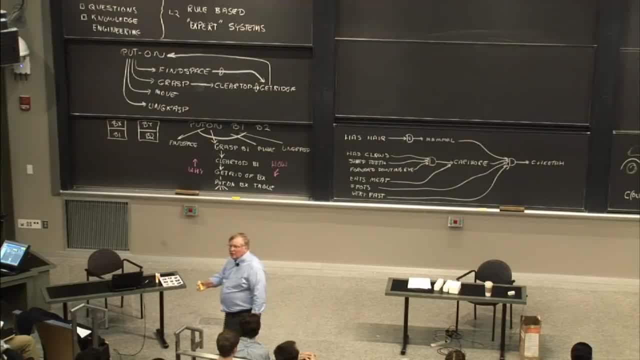 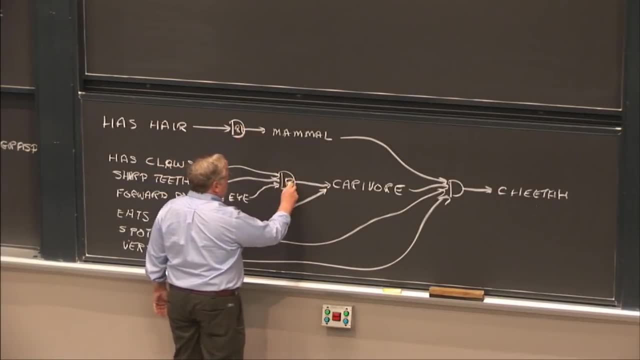 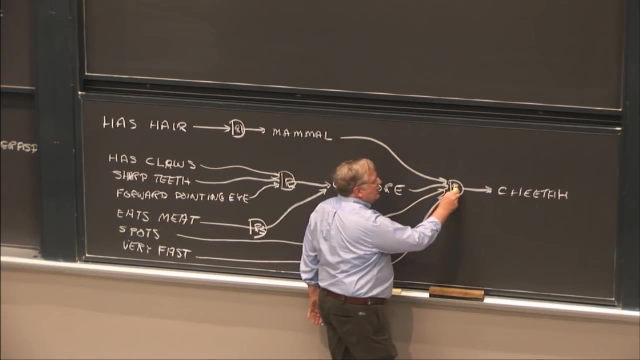 But for our small zoo that will do So. we have now written down, in the form of these AND gates, several rules: R1,, R2, and there needs to be an AND gate here, that's R3, and an R4,, all of which indicated: 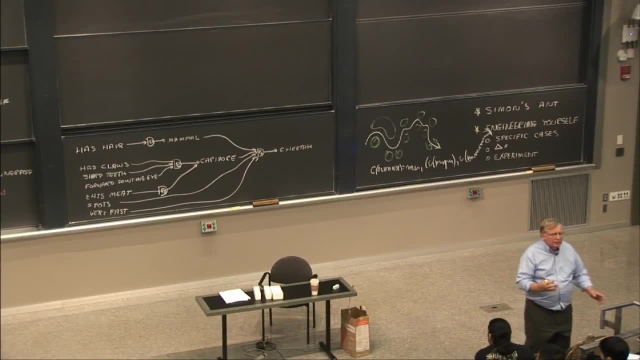 this animal is a cheetah. So we built ourself a little rule-based expert system that can recognize exactly one animal. But you can imagine, You can imagine filling out this system with other rules so you can recognize giraffes and penguins and all the other. 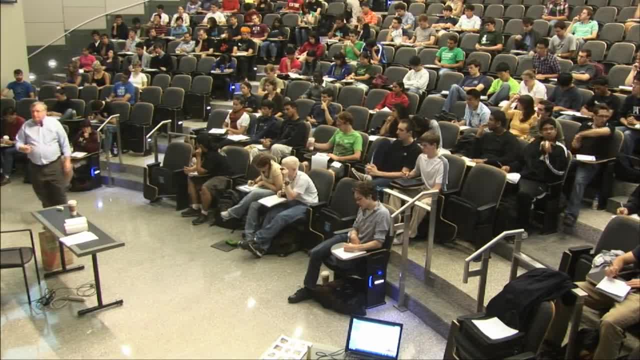 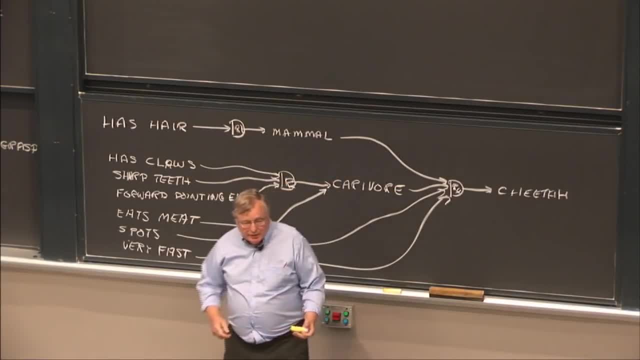 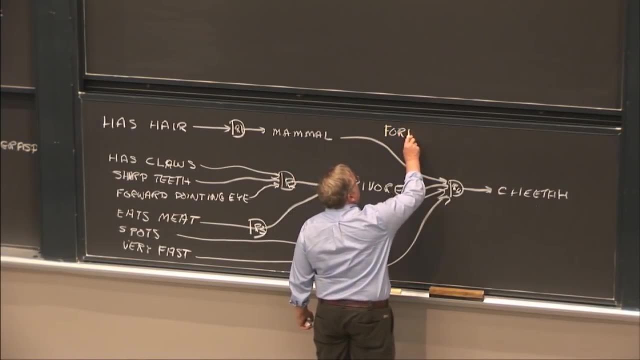 sorts of things to find a small zoo. So when you have a system like this that works as I've indicated, then what we're going to call that, we're going to give that a special name And we're going to call that a forward chaining. 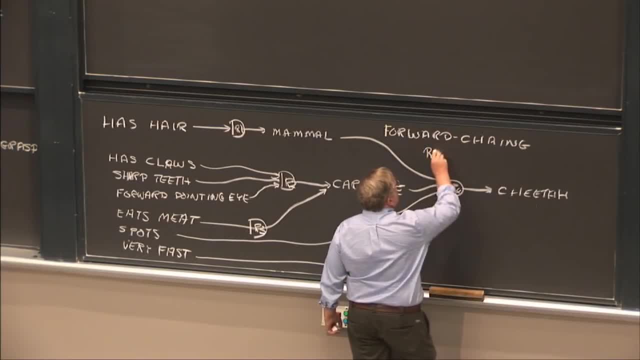 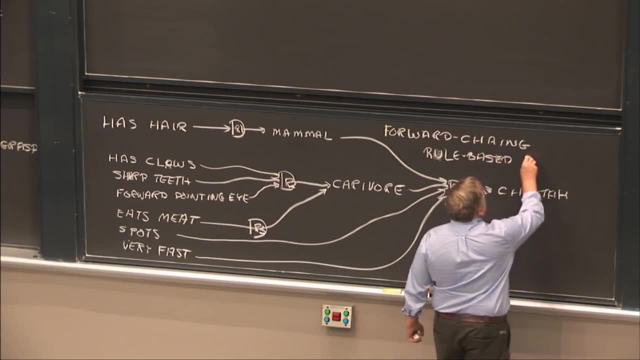 And we're going to call that a rule-based because it uses rules. expert system- And we're going to put expert in parentheses because when these things were developed for marketing reasons, they call them expert systems instead of novice systems. So we're going to call them expert systems instead of. 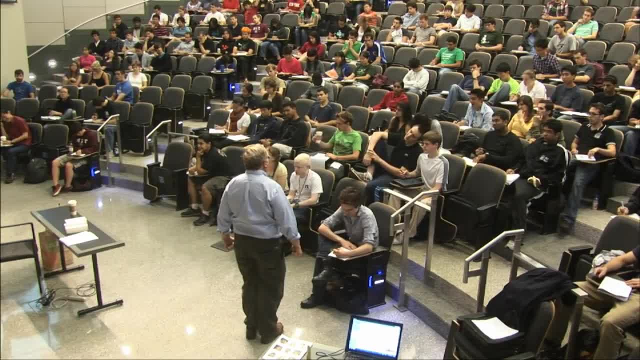 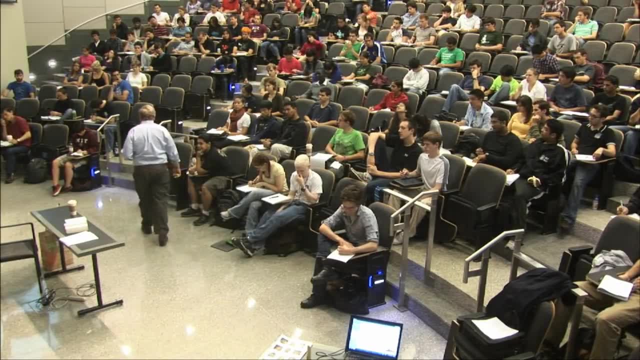 novice systems. But are they really experts in a human sense? Not really, because they have these knee-jerk rules. They're not equipped with anything you might want to call common sense. They don't have an ability to deal with previous cases like 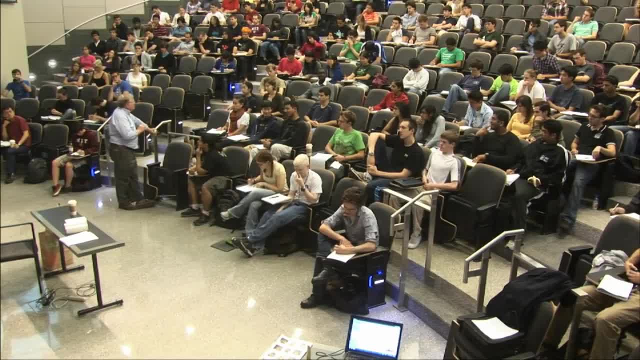 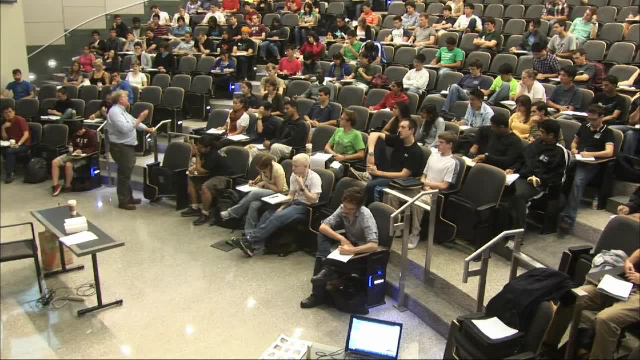 we do when we go to medical school. So they really ought to be called rule-based novice systems, because they reason like novices on the basis of rules. But the tradition is to call them rule-based expert systems, And this one works forward. 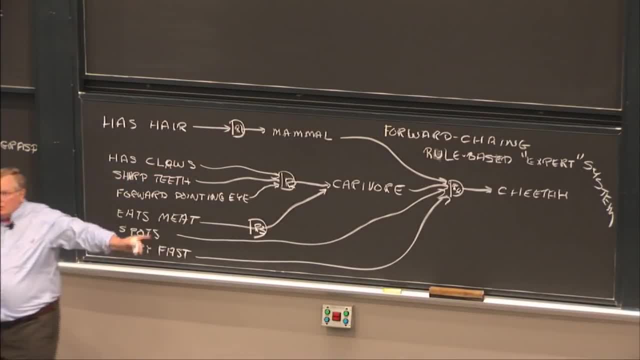 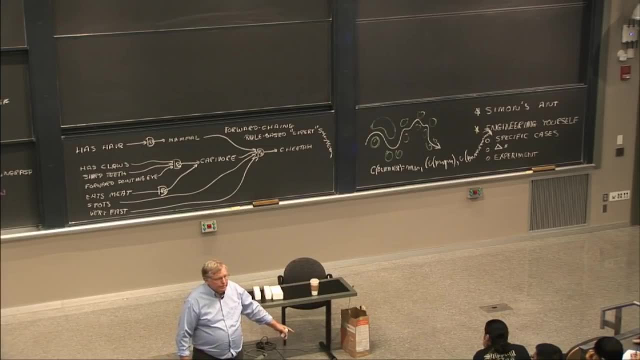 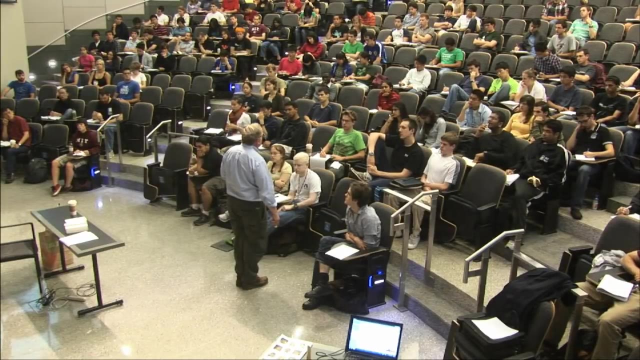 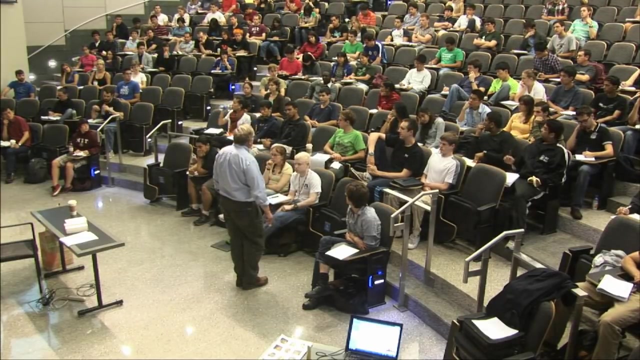 So it's a system that is able to go from the facts we give it to the conclusion off on the right. That's why it's a forward chaining system. Can this system answer questions about its own behavior? Waswell, what do you think? 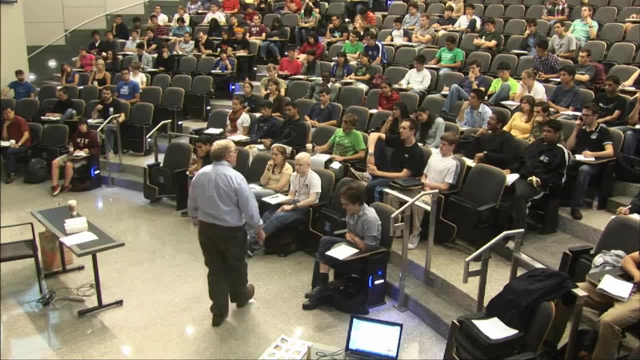 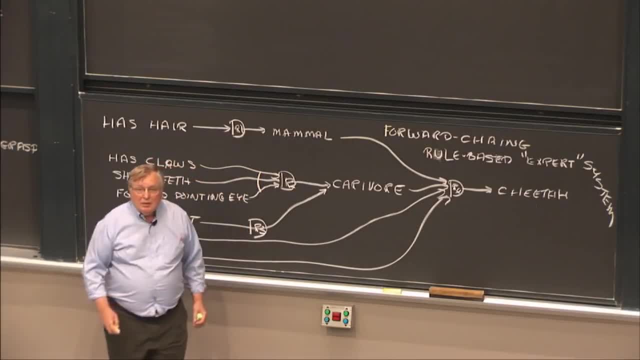 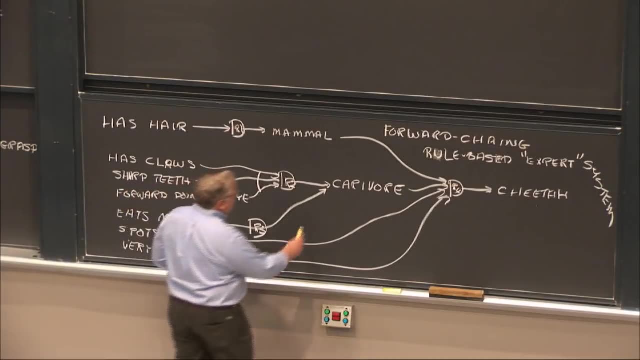 Why This is, in fact, building a gold tree, Because each of these rules that require several things to be true is creating an AND node, And each of these situations here where you have multiple reasons for believing the thing is a carnivore. that's. 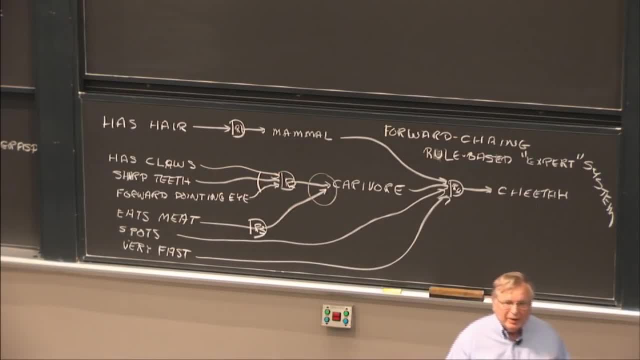 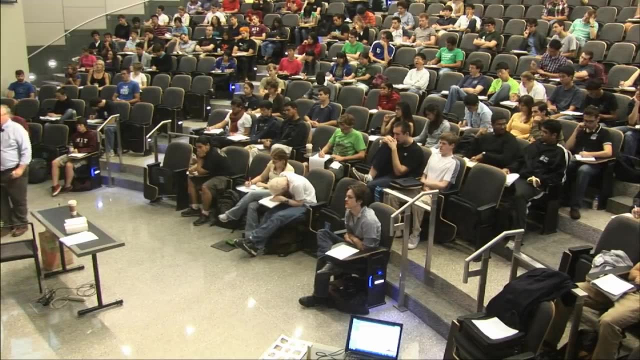 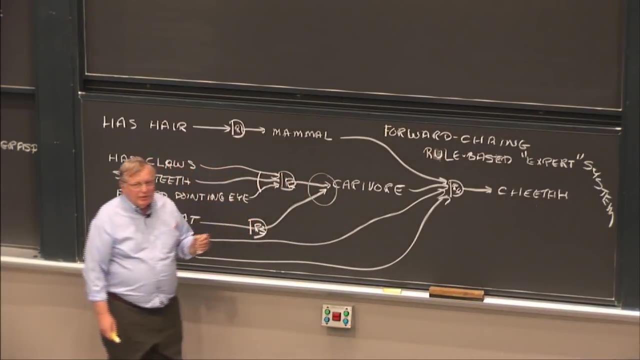 creating an OR node, And we already know that you can answer questions about your own behavior if you leave behind a trace of a gold tree. So look at this. if I say to it, why were you interested in the animal's claws? Because I was trying to see if it was a carnivore. 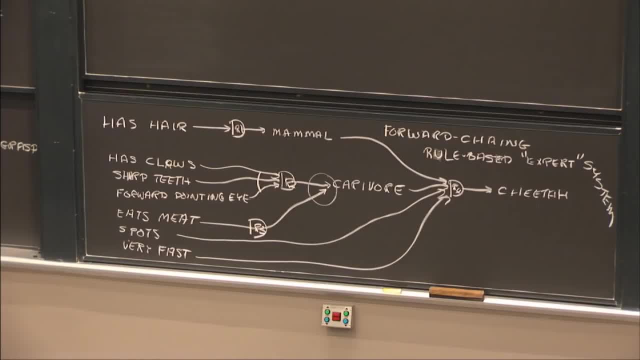 How did you know that the animal is a mammal? Because it has hair. Why did you think it was a cheetah? Because it's a mammal. a carnivore has spots, and very fast. So by working forward and backward in this. 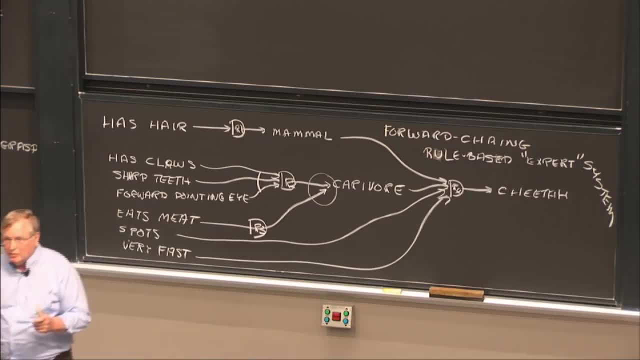 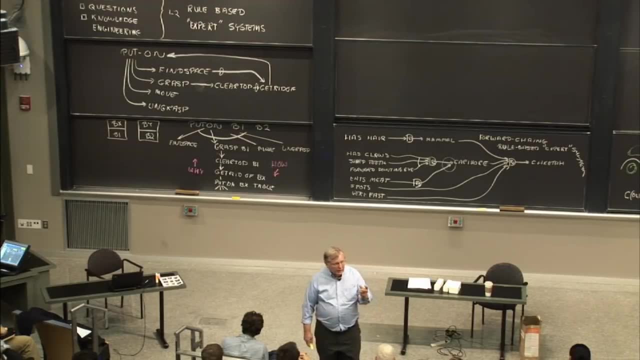 gold tree. this too can answer questions about its own behavior. So now you know how, going forward, you can write programs that answer questions about their behavior. Either you write the subroutines, so that each one is wrapped around a goal, so you've got. 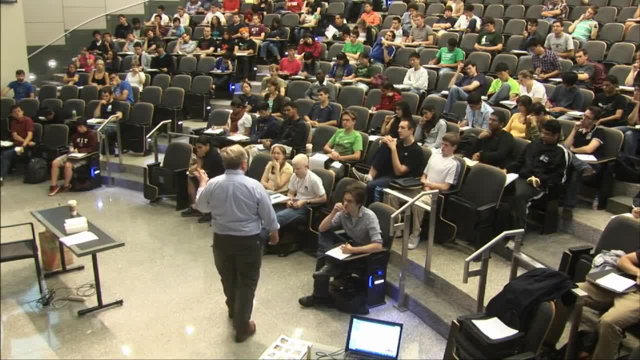 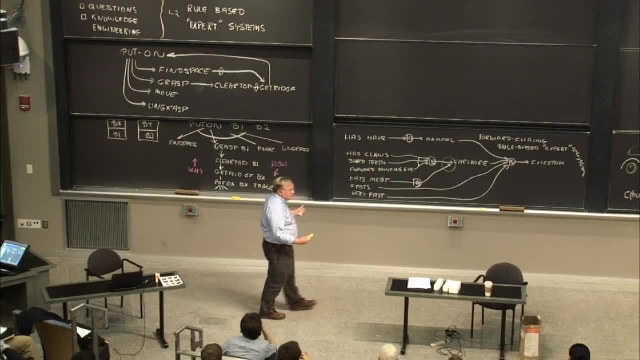 goal-centered programming, Or you build a so-called expert system using rules, in which case it's easy to make it leave behind a trace of a gold tree which makes it possible to answer questions about its own behavior, just as this Blocksboro program did. 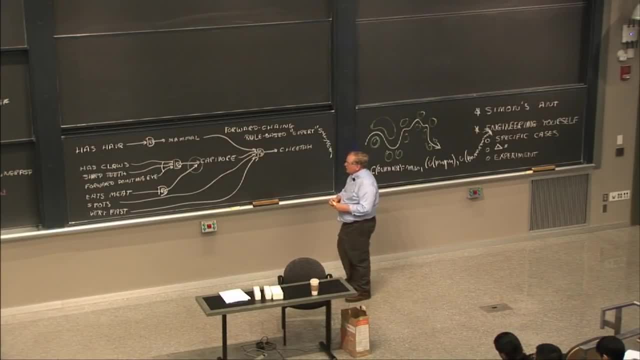 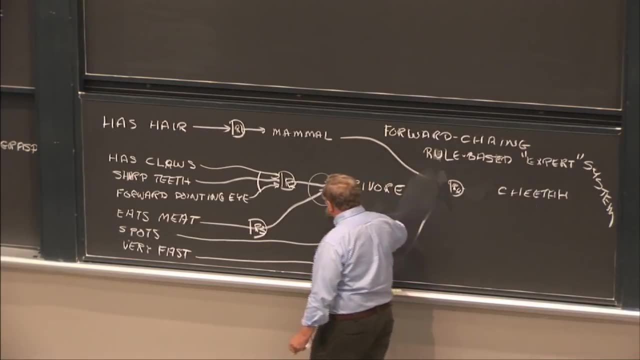 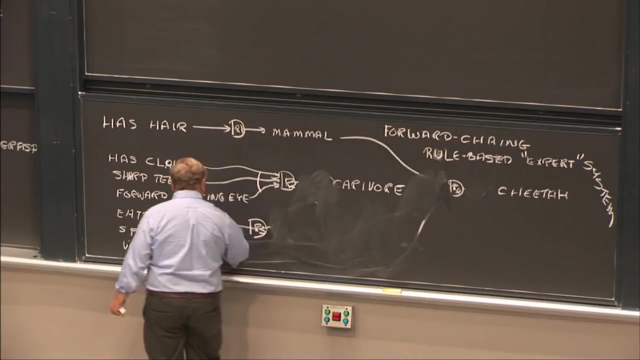 But now a little more vocabulary. I'm going to save time by erasing all of these things that I previously drew by way of connections, And I'm going to approach this zoo in a little different way. I'm going to not ask any questions about the animal. 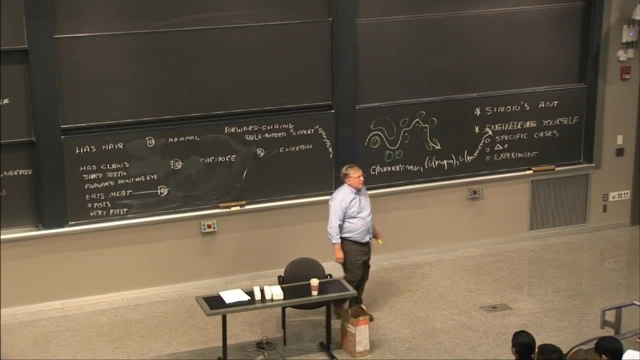 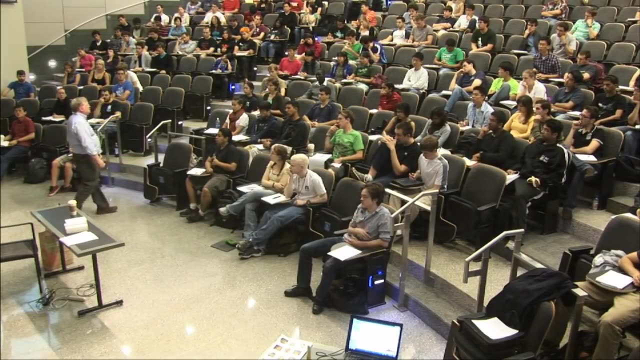 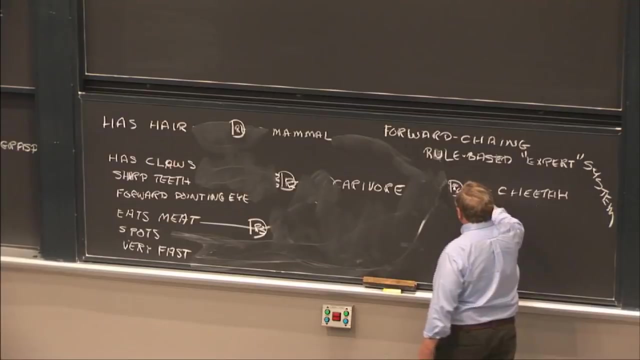 Instead, I'm going to say: mommy, is this thing? I'm looking at a cheetah, And how would mommy go about figuring it out In her head? she would say, well, I don't know. If it's going to be a cheetah, then it must be the case that 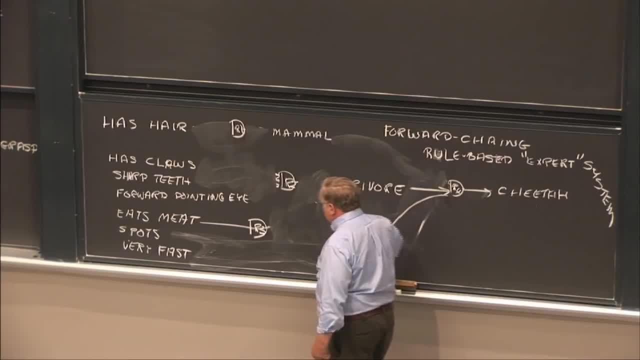 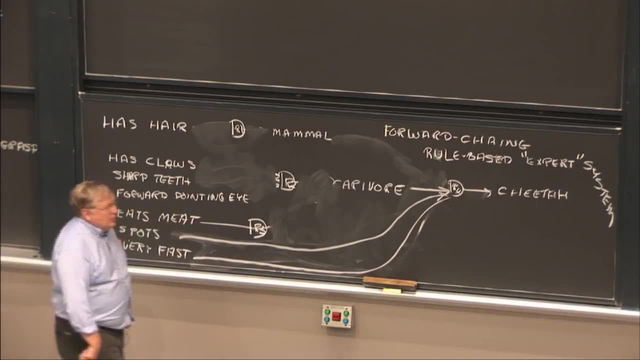 it's a carnivore And it must be the case that it has spots, And it must be the case that it's very fast. So so far, what we've established is that if it's going to be a cheetah, it has to have the four 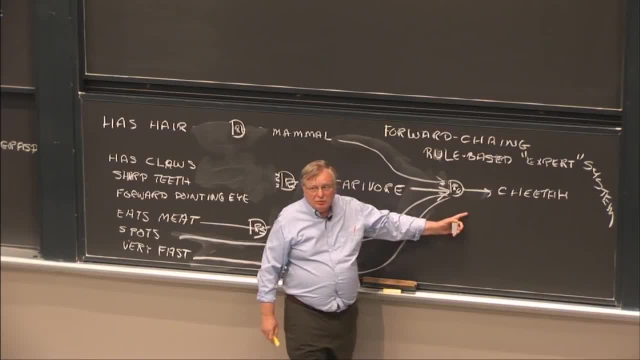 characteristics that mommy finds behind this rule R4.. So instead of working forward from facts, what I'm going to do is work backward from a hypothesis. So here the hypothesis is: this thing is a cheetah. How do I go about showing whether that's true or not? 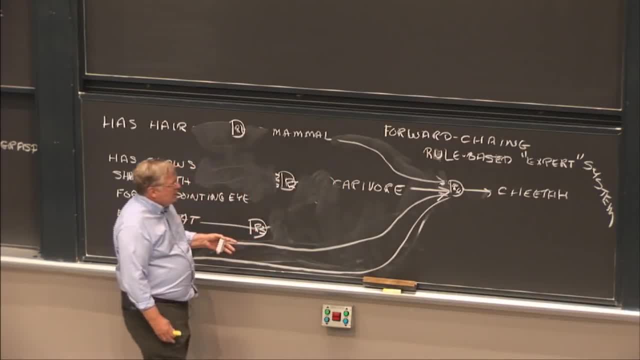 Well, I haven't done anything so far, Because all I know is: is it a cheetah? if all of these things are true, but are they true? Well, to find out if it's a mammal, I can use rule one. 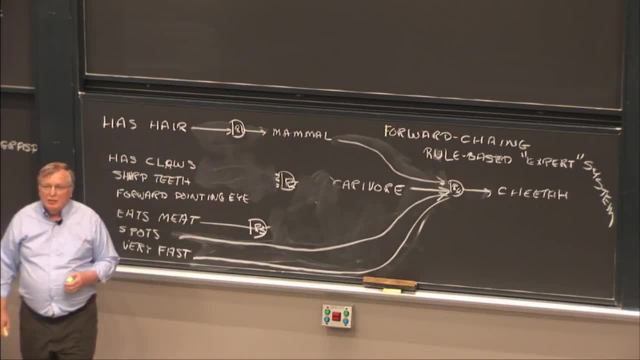 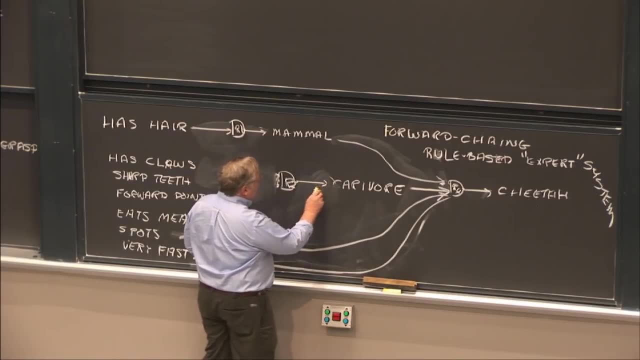 And if I know or can determine that the animal has hair, then that part of it is taken care of. And I can similarly work my way back through carnivore by saying: well, it's a carnivore if it has claws, sharp teeth. 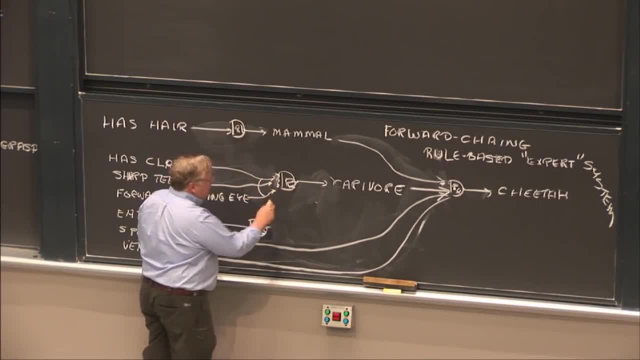 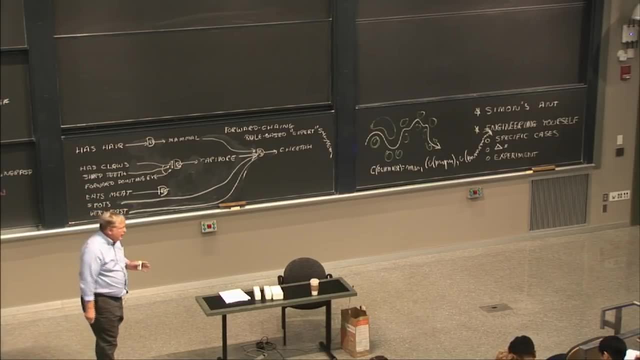 and forward-pointing eyes And in as much as the animal in question does, then I'm through. I know it's a carnivore. I don't have to go through and show that it's a carnivore another way, So I'll never actually ask questions about. 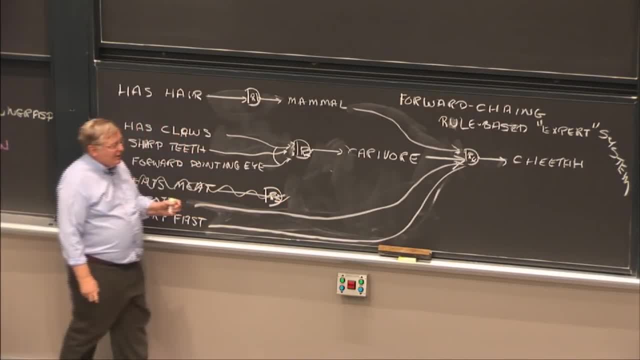 whether it eats meat. Finally, the final two conditions are met by just an inspection of the animal, That is to say it's in the database, I don't have to use any rules to determine that the animal has spots, and it's very fast. 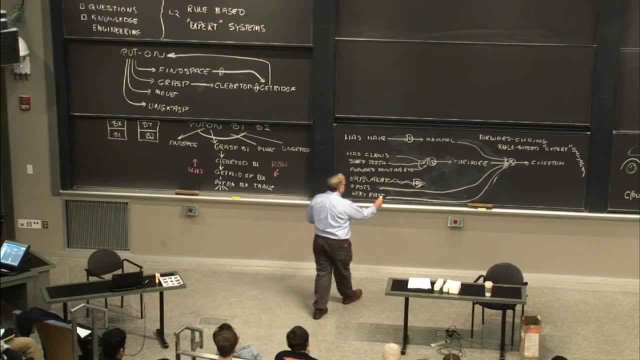 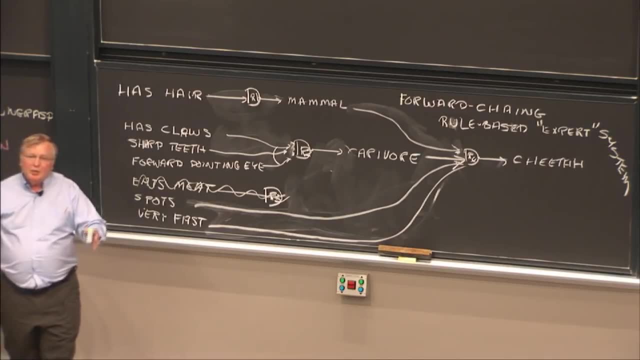 So now I've got everything in place to say that it's a cheetah, because it's a carnivore, because it has claws, sharp teeth and forward-pointing eyes, And all the rest of the stuff is similarly determined by going backwards. 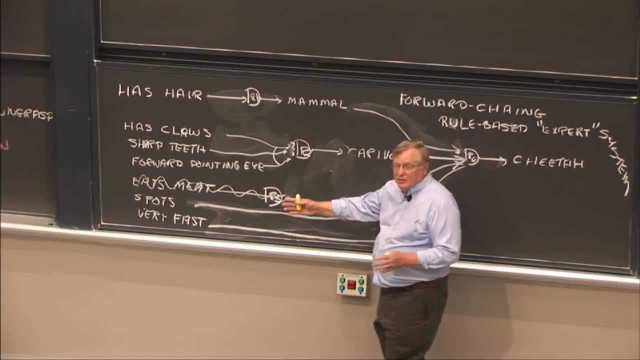 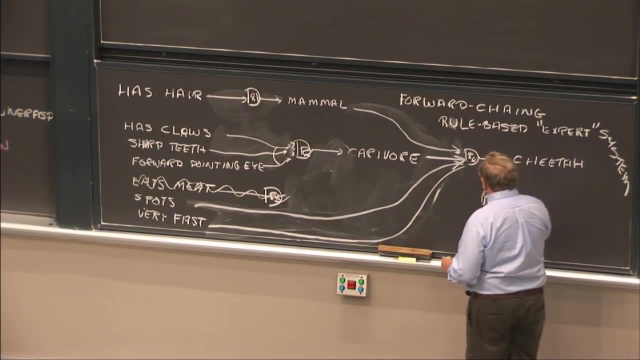 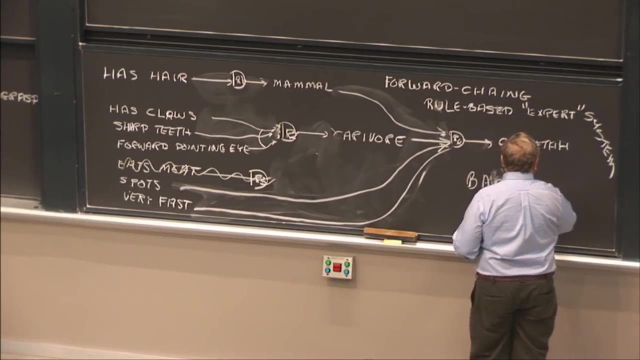 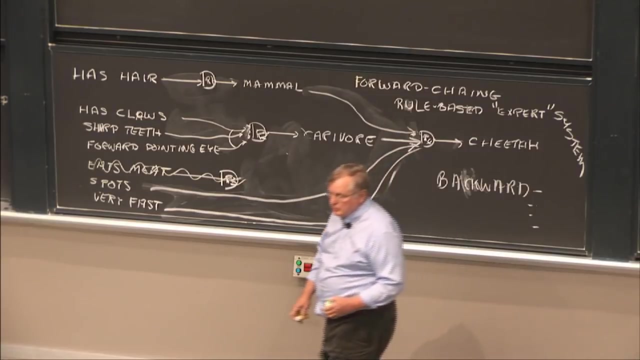 Backwards, from the hypothesis toward the facts, instead of from the facts forward to the conclusions. So building a system that works like that. I have a backward, A backward-chaining, rule-based expert system. But there's a very important characteristic of this system. 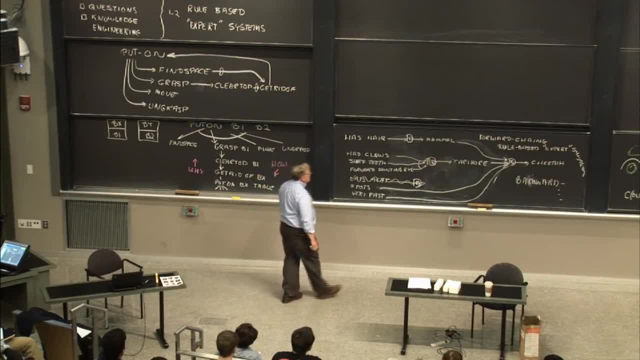 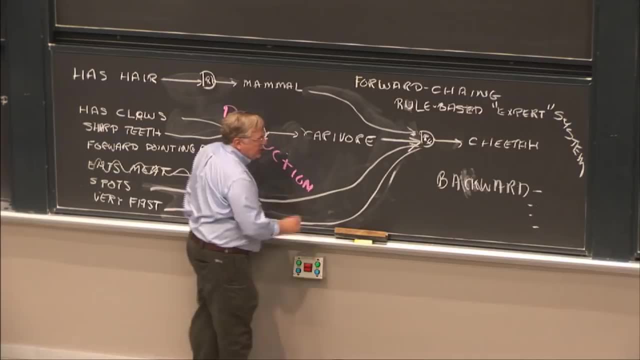 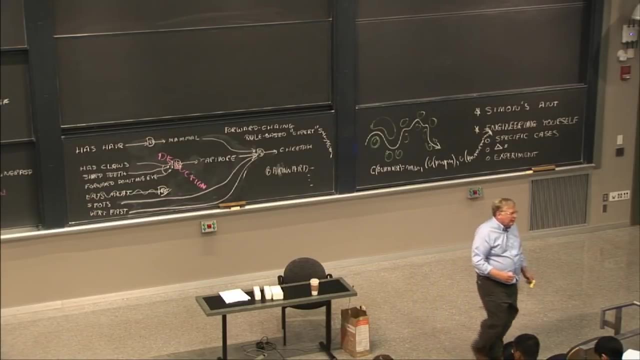 in both backward and forward mode, and that is that this thing is a deduction system. That's because it's working with facts to produce new facts, And when you have a deduction system you can never take anything away. But these rule-based systems are also used in another mode. 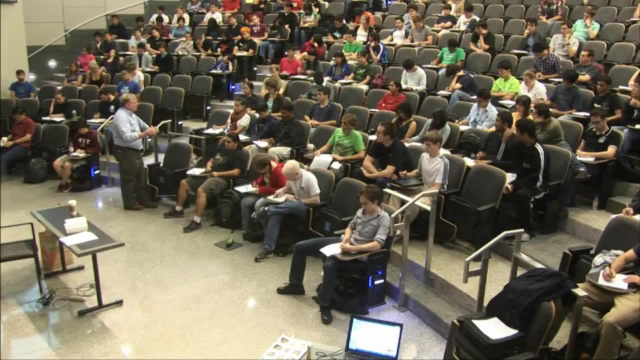 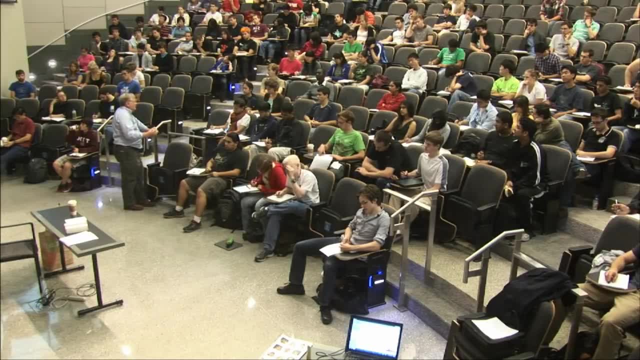 where it's possible to take something away. See, in fact world, the deduction world. you're talking about proving things, And once you prove something is true, it can't be false. If it is, you've got a contradiction in your system. 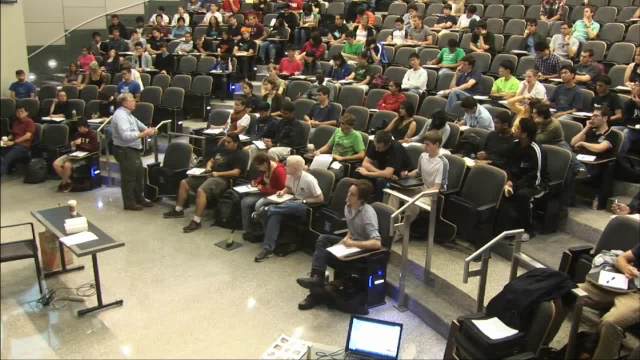 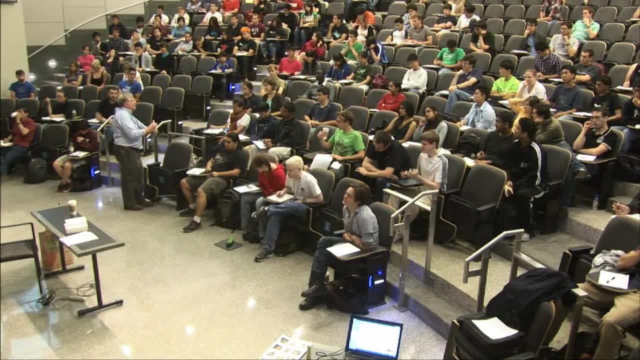 But if you think of this as a programming language, if you think of using rules as a programming language, then you can think of arranging it so that these rules are going to always add or subtract from the database. Let me show you an example of a couple of systems. 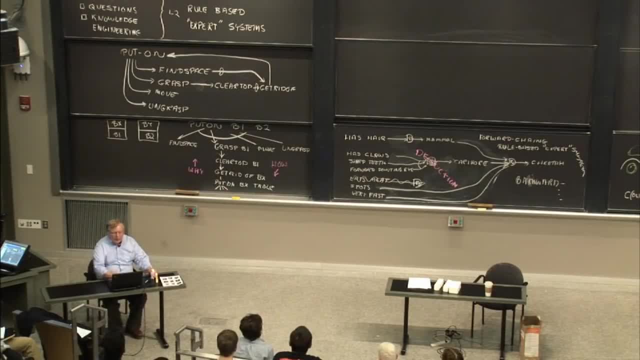 First of all, since I've talked about the Myces system, let me show you. Here's an example of a Mycene Dialogue. That's a Mycene Dialogue And you can see the appearance of words. you have to go to medical school to learn. 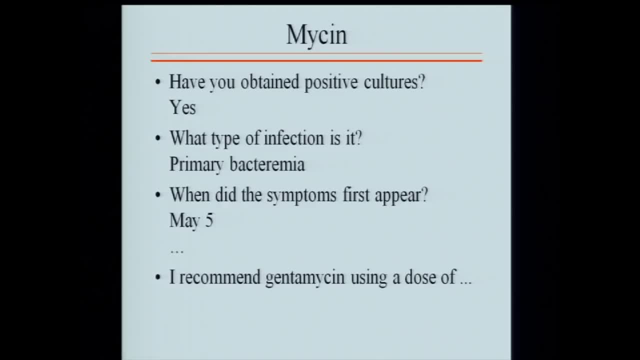 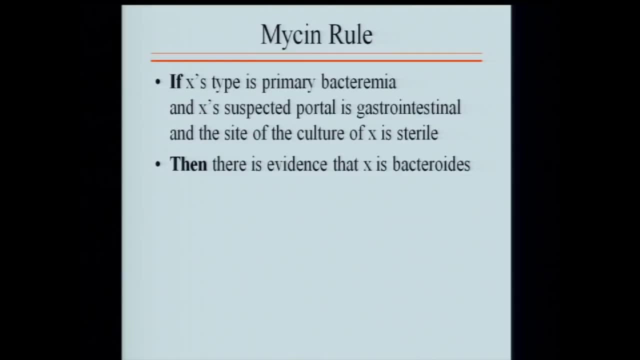 And here's a typical Mycene rule, just like the rules for doing zoo analysis, only a more complicated domain. But here's another example of a system that was written not in the 80s but just a couple of years ago, And it's called the Mycene Dialogue. 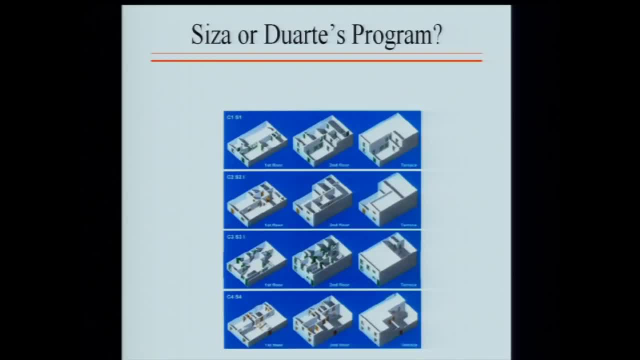 And you can see that the Mycene Dialogue is very similar to the Mycene Dialogue. It was written not in the 80s but just a couple years ago by a student in the architecture department, a PhD thesis. He was interested in the architecture of a Portuguese. 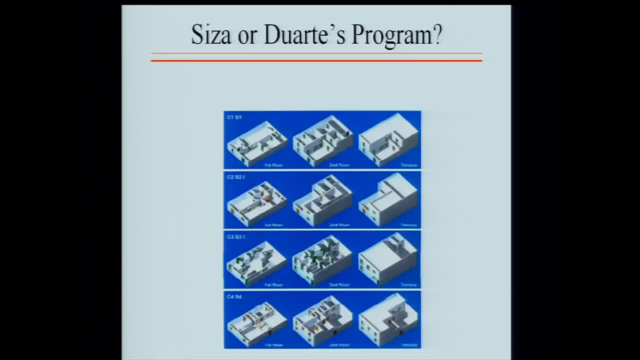 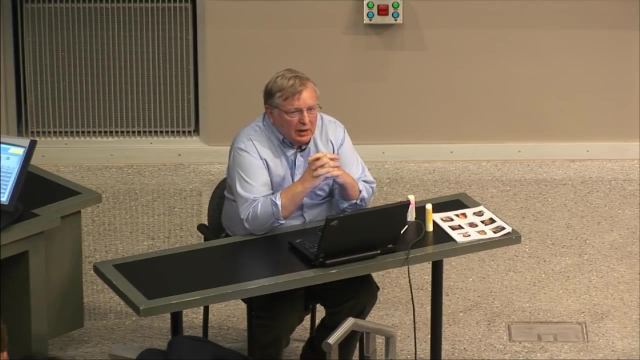 architect named Siza, And Siza has done a lot of mass housing stuff, And Siza has the idea that you ought to be able to design your own house. And so Jose Duarte, a Portuguese student and a PhD student in architecture, wrote a rule-based system that was. 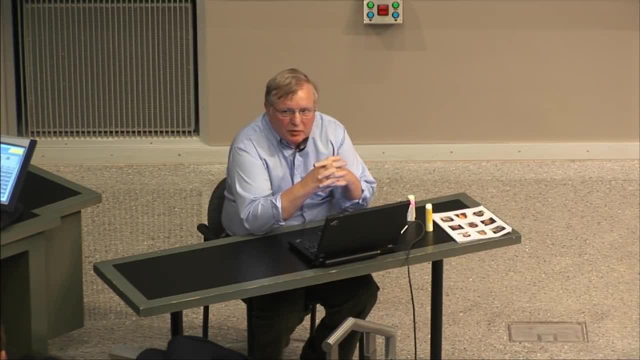 capable of designing Siza-like houses in response to the requirements and recommendations and desires of the people who were going to occupy the houses. So the most compelling part of this exercise was that Duarte took some of the designs of the program, mixed them up with. 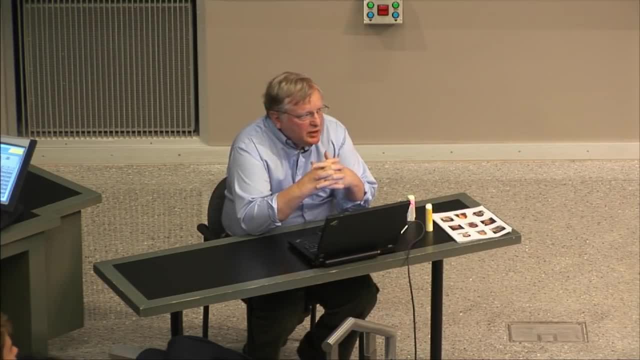 some of the designs of Siza and put them in front of Siza and said, which ones did you do? And Siza couldn't tell. So somehow the rule-based system that was built using this kind of technology was sufficient to confuse even the 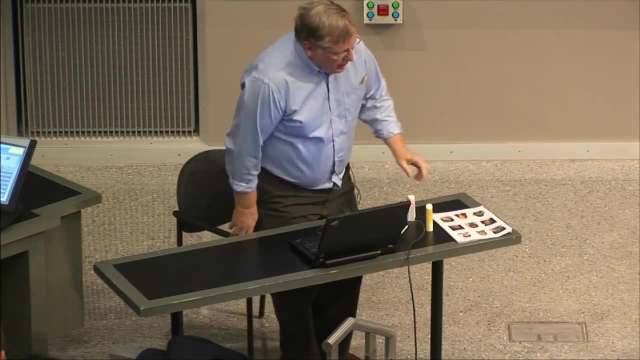 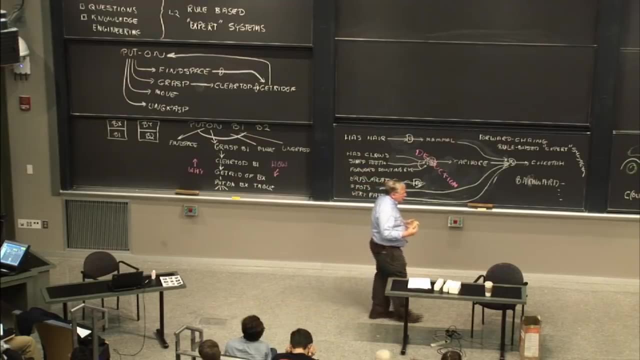 expert that they were patterned after. But this program is a little complicated. It too has its own specialized lingo, So I'm not going to talk about it in detail, but rather talk instead about an analogous problem, And that is a problem that everyone has faced at one. 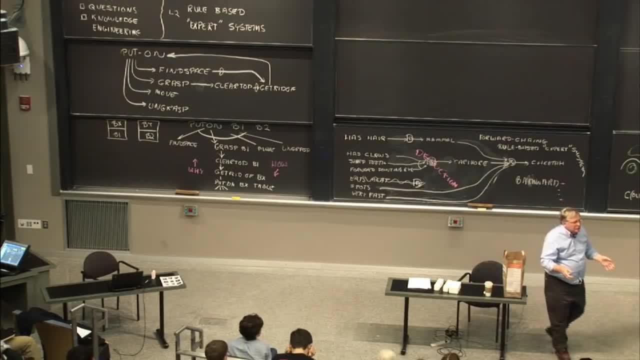 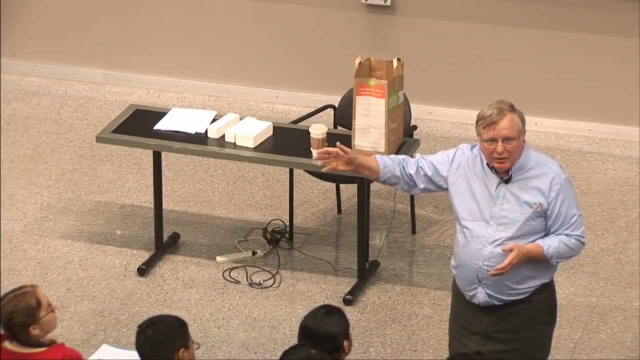 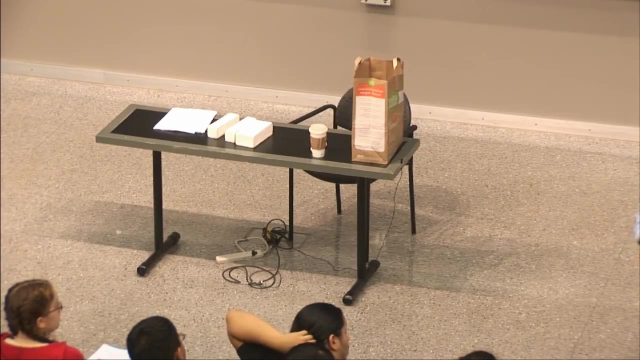 point or another, And that is the problem of putting, for example, the groceries in a bag at a grocery store. It's the same thing, right? Instead of putting rooms in a house, you're putting groceries in a bag, And there must be some rules about how to do that. 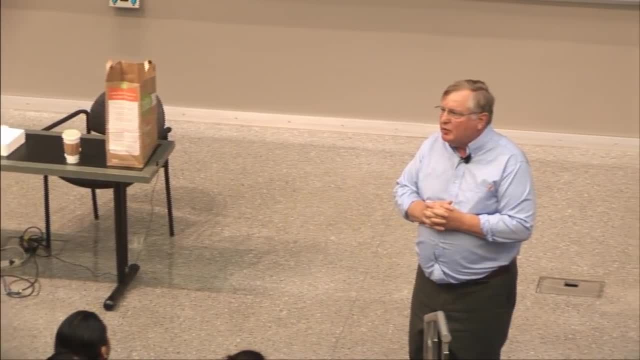 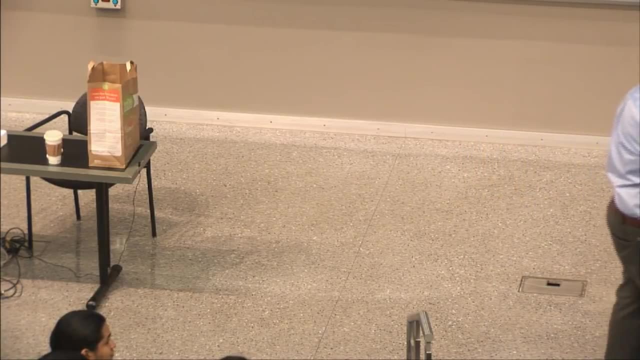 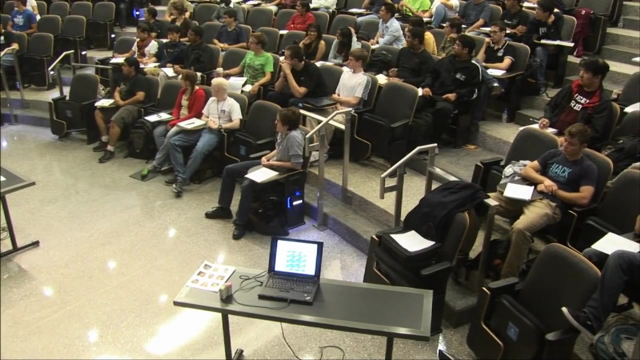 In fact, maybe some of you have been professional grocery store baggers. Ariel is a grocery professional bagger. You're a? Which one? I used to work at MarketBus. Yeah, what is your name, Lisa? OK, we've got two professional grocery store baggers. 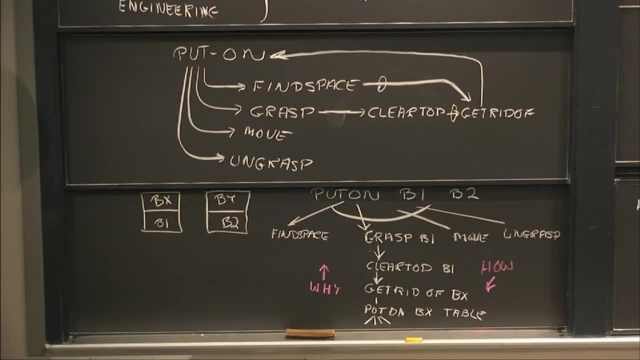 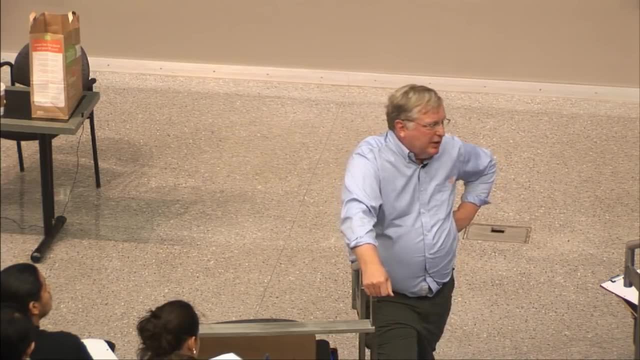 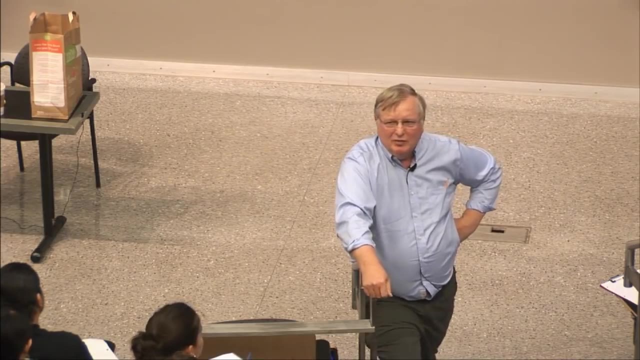 And I'm going to be now simulating a highly paid knowledge engineer desirous of building a program that knows how to bag groceries. So I'm going to visit your site, MarketBasket, and I'm going to ask Lisa now, fearful of losing her job, if she 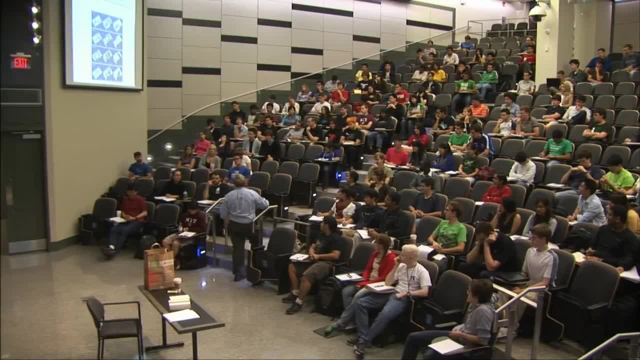 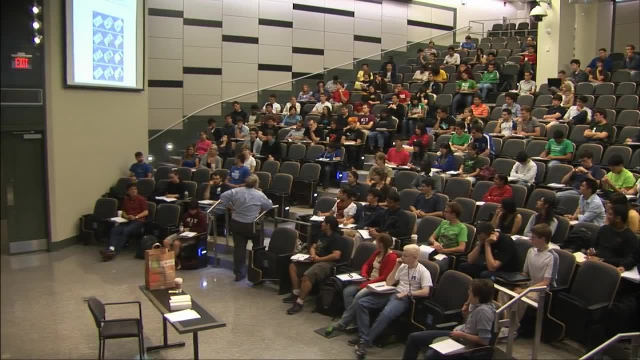 would tell me about how she bags groceries. So could you suggest a rule? Sure, Large items in the bottom, Large items in the bottom. You see, that's why I'm a highly paid knowledge engineer, because I translate what she said into an if-then rule. 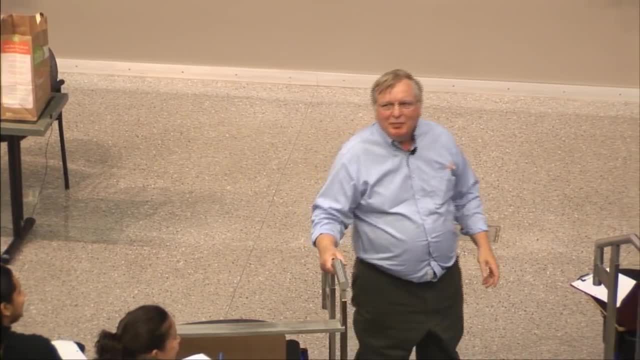 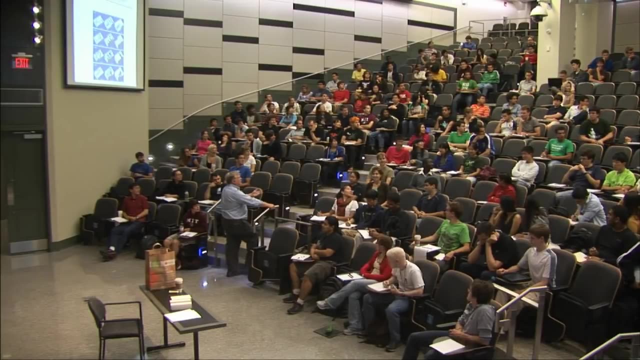 So if large, then bottom. So now I've got it. So how about you? Ariel, You got a suggestion About how to bag groceries. I mean, you can get small things on the top, Put them in the bottom. Yeah, 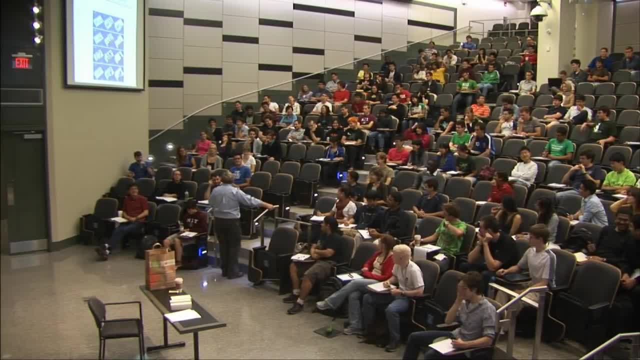 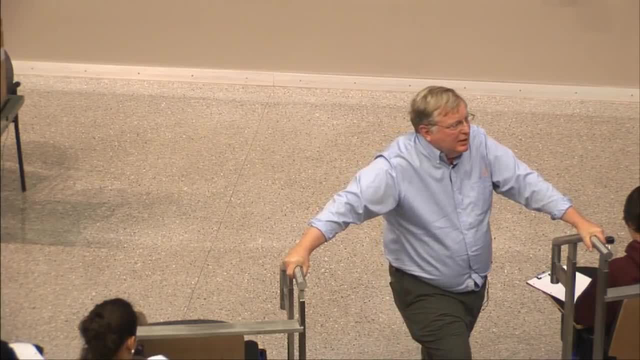 If small, then on top. Lisa, have you got anything else you can tell me? Don't put too many heavy things in the same bag. Don't put too many heavy things in the same bag. So if heavy greater than three, then no bag, or 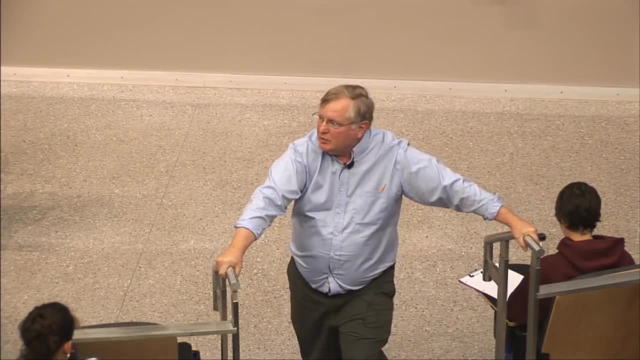 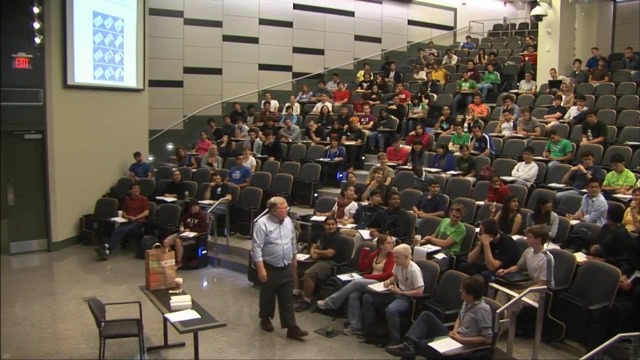 something like that. Is that all we're going to be able to do? Does anybody else want to volunteer? Scylla, have you bagged groceries in Turkey? So they don't have grocery baggers, so we have to. Everybody's a professional bagger, so yeah. 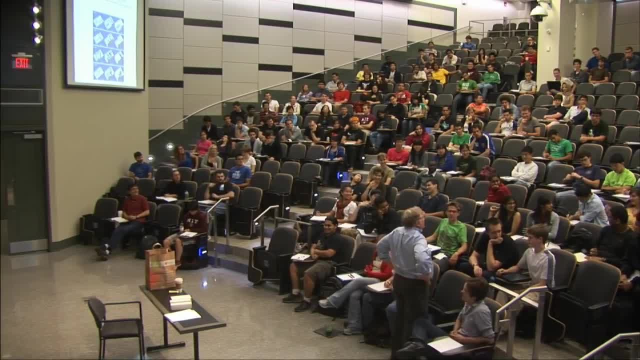 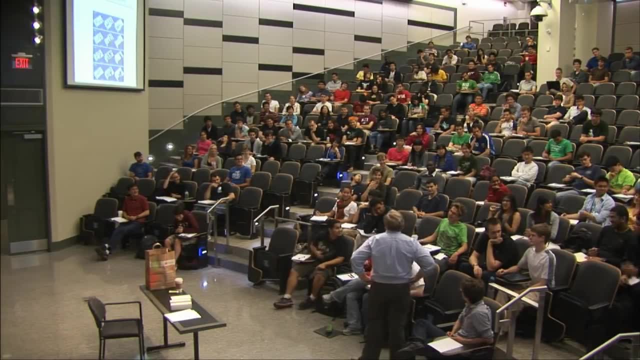 It's outsourced to them, Trust me. So no squishies on the bottom, No squishies on the bottom. If you have tomatoes, you don't want them to get squishy. Now there's a very different thing about squishies and 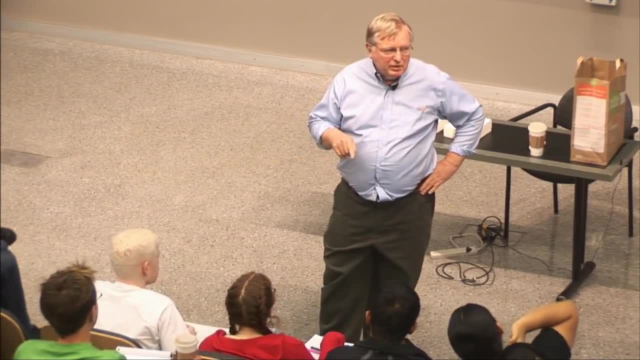 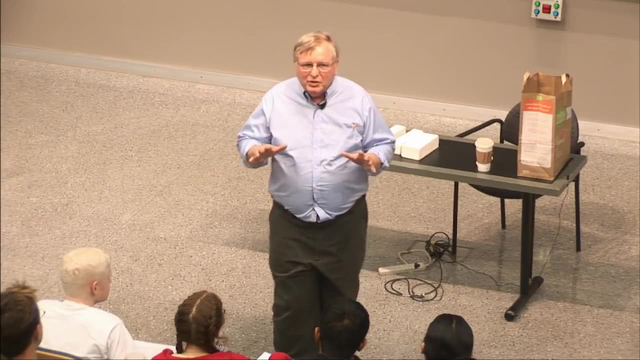 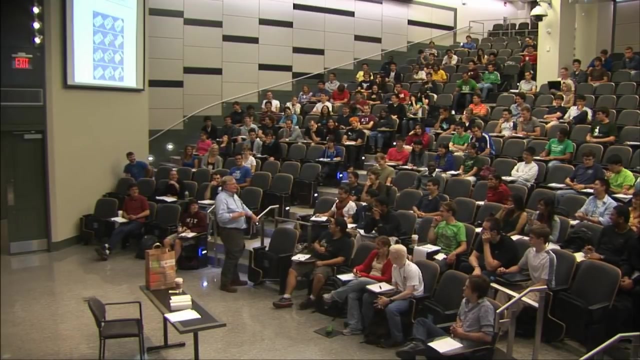 tomatoes, because tomato is specific and squishy isn't. One tendency of MIT students, of course, is that we all tend to generalize. I once knew a professor in a Sloan school who seemed real smart. Then I figured out what he did. 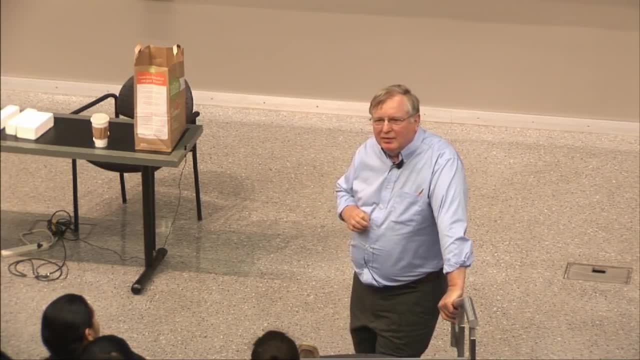 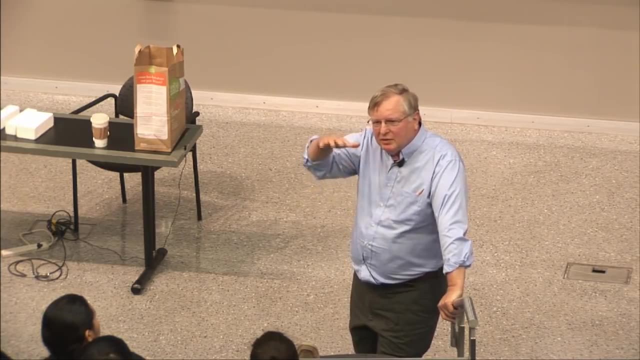 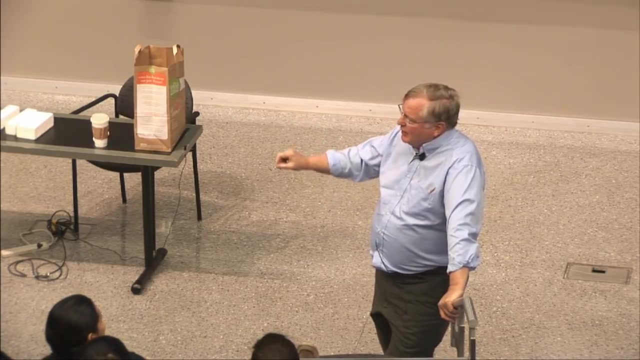 If I were to say I'm thinking about a red apple, he'd sit back and say: oh, I see you're contemplating colored fruit today. Just taking it up one level of abstraction, Man of genius. He also was able to talk for an hour after he drew a. 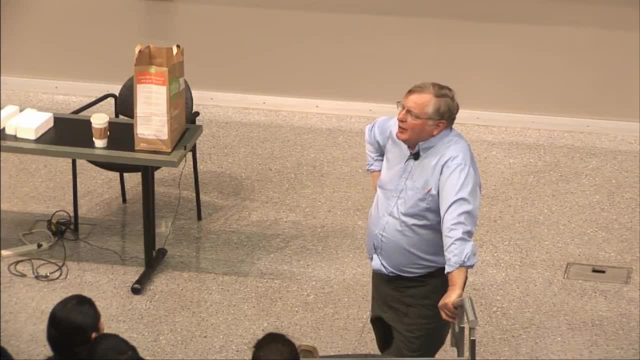 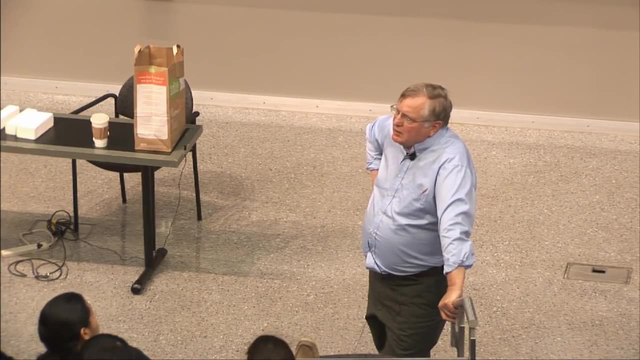 triangle on the board. Amazing people. Anyhow, where were we? Oh yes, Bagging groceries. So we're making something. We're making something. We're making some progress, but not as much as I would like, and so, in order to really make progress on tasks, 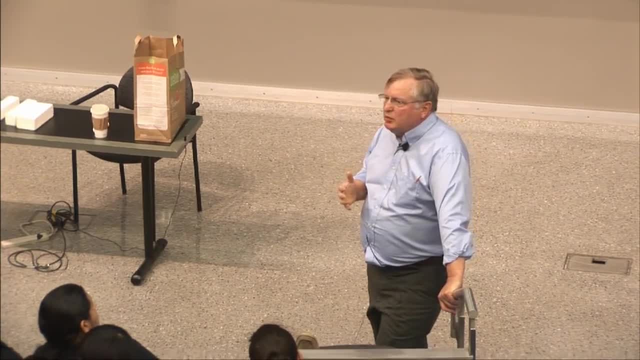 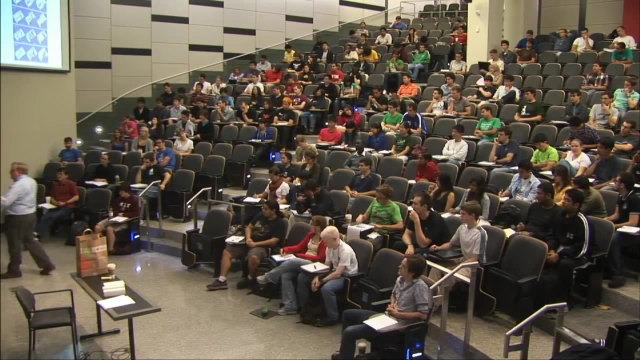 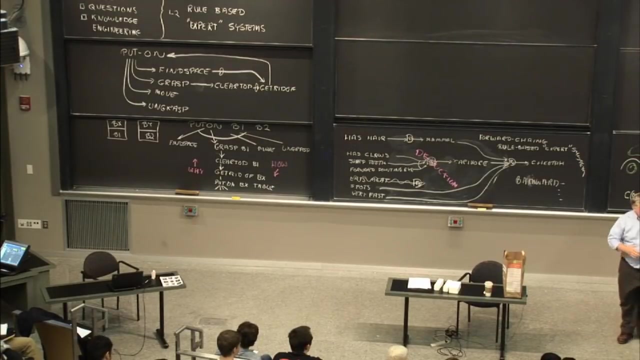 like this. you have to exercise, you have to know about some principles of knowledge engineering. So principle number one, which I've listed over here as part of a gold star idea, is deal with specific cases. So, while you're at the site, if all you do is talk to the 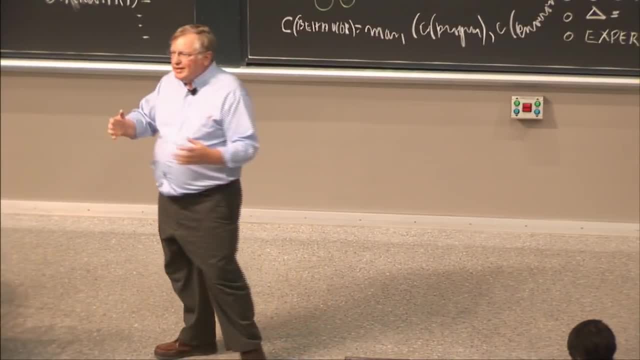 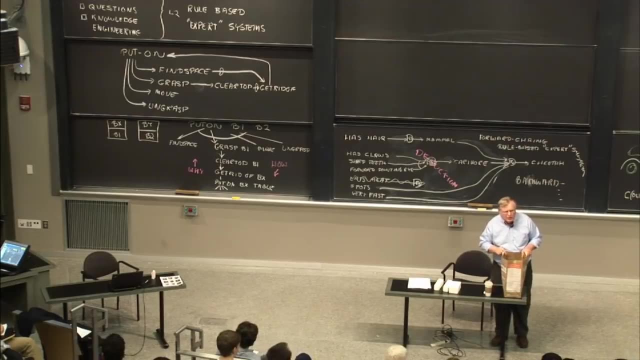 experts like Lisa and Ariel. All you're going to get is vague generalities, because they won't think of everything. So what you do is you say: well, let me watch you on the line, And then you'll see that they have to have some way of. 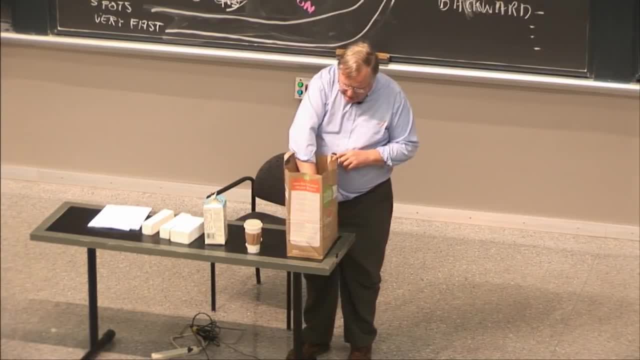 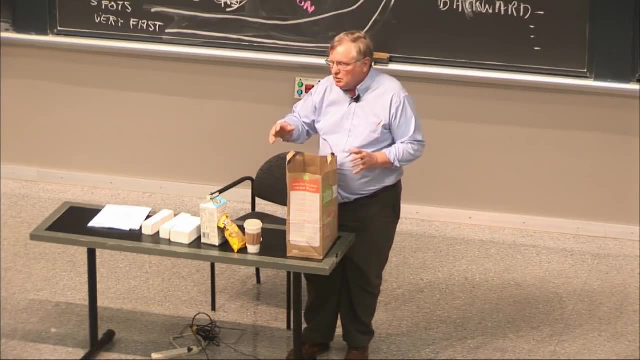 dealing with the milk, And then they will see that they have to have some way of dealing with the potato chips. Nobody mentioned potato chips, except insofar as they might be squishy- Squishy. We don't have a definition for squishy. 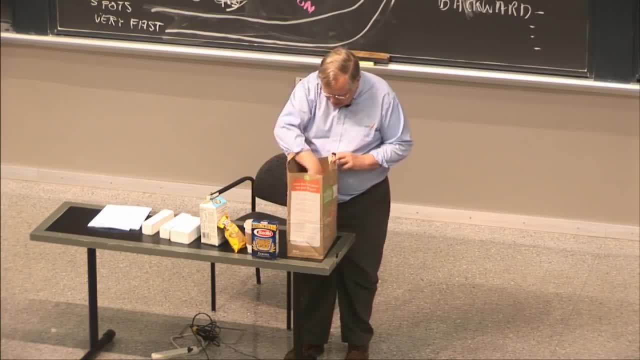 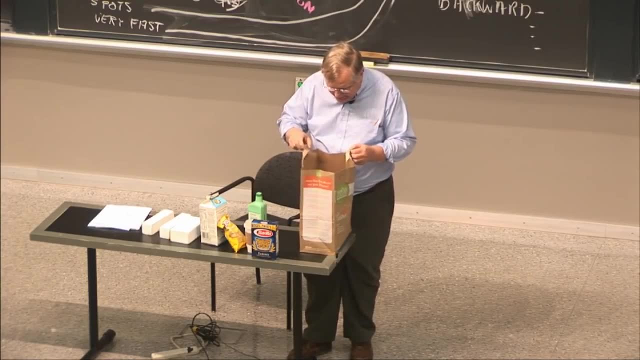 No one talked about the macaroni. and no one talked about the motor oil. This is a convenience store. Probably don't want that in the same bag with the meat. And then no one talked about canned stuff. Here's a can of olives. 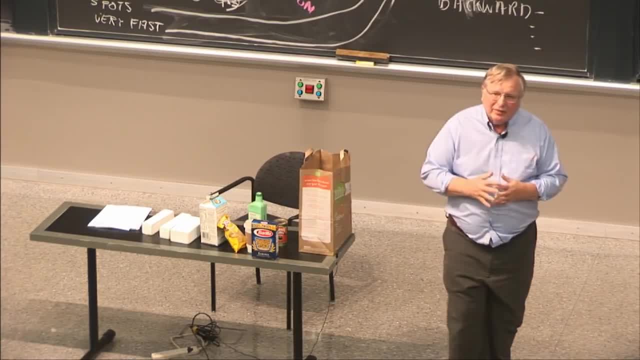 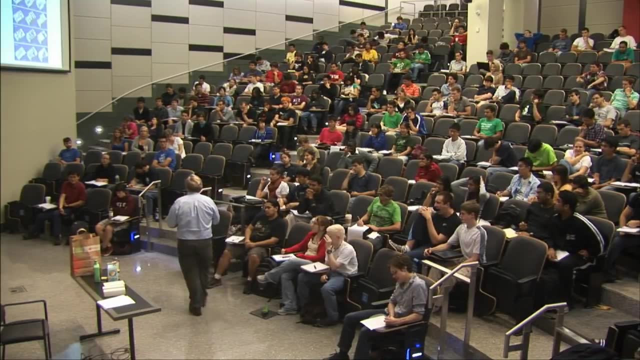 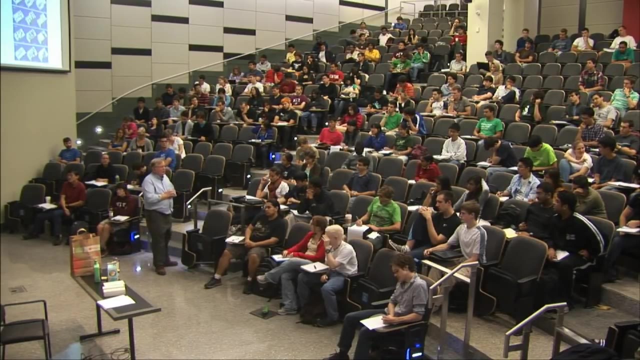 So by looking at specific cases, you will elicit from people knowledge that they otherwise would not have thought to give you Knowledge engineering rule number one And within a very few minutes you'll have all three knowledge engineering rules And be prepared to be a highly paid knowledge engineer. 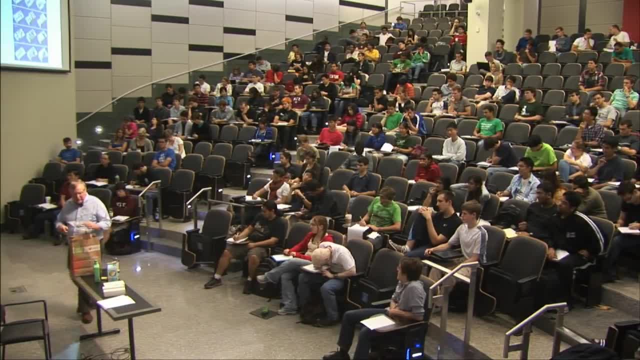 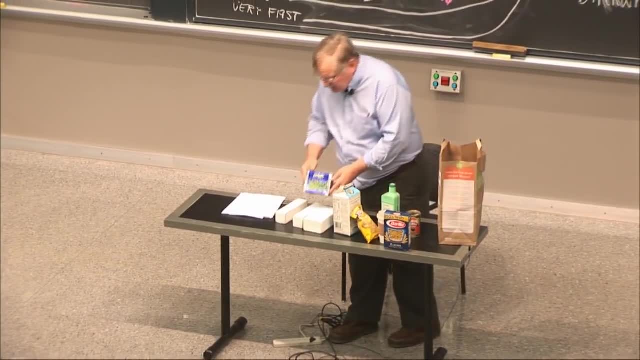 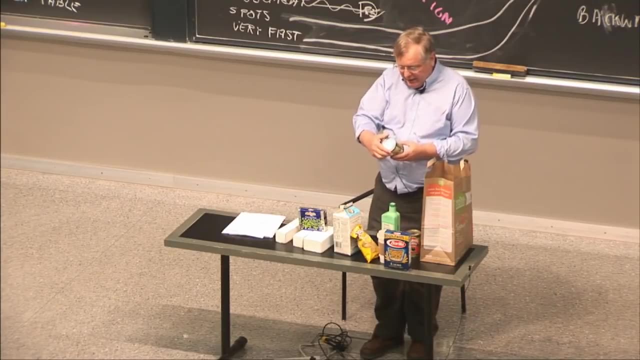 Let's call these heuristics. Heuristic number one: specific cases. Heuristic number two is: ask questions about things that appear to be the same but are actually handled differently. So there's some bird's eye frozen peas And here some fresh cut sweet peas. 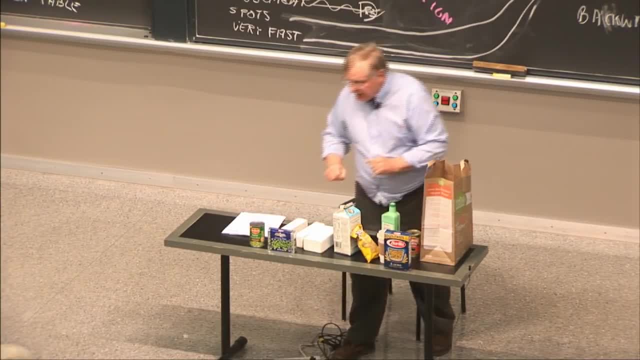 And to me it's a little bit of a challenge. It's a little bit of a challenge. It's a little bit of a challenge. A person who's never touched a grocery bag in my life. Maybe I'm from Mars. I can't tell the difference. 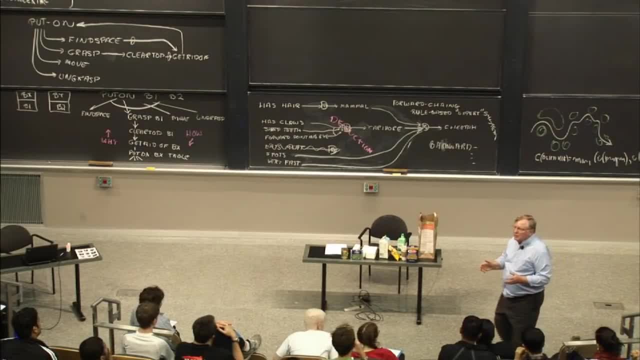 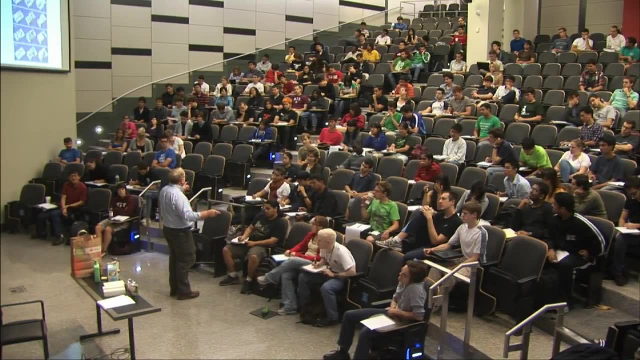 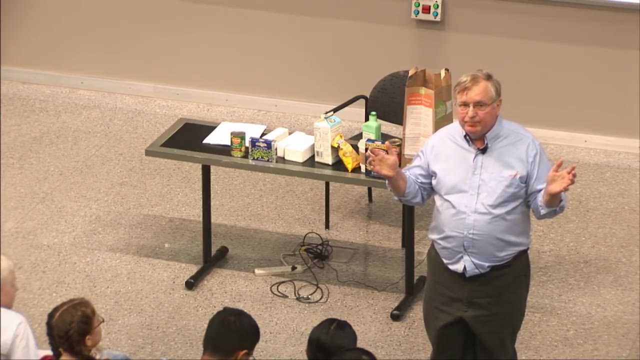 They're both peas, But I observe that the experts are handling these objects differently. So I say: why did you handle those peas differently from those peas? And what do they say? One's canned and one's frozen. So what happens? Bingo. 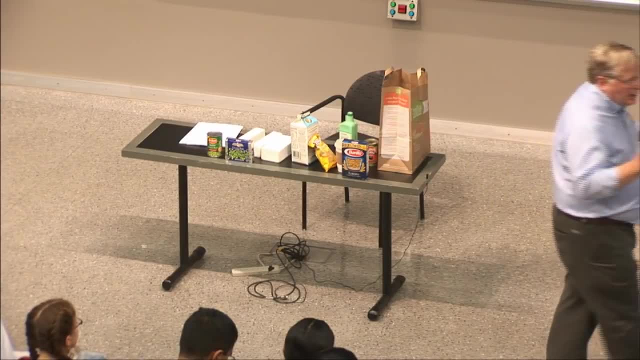 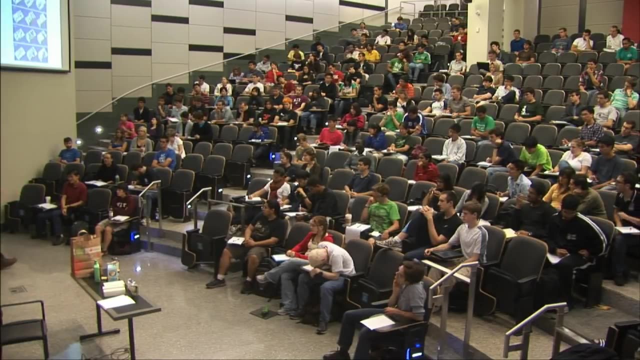 I've got some new words in my vocabulary And those new vocabulary words are going to give me power over the domain, because I can now use those words in my rules And I can write rules like: if frozen, then put them all. 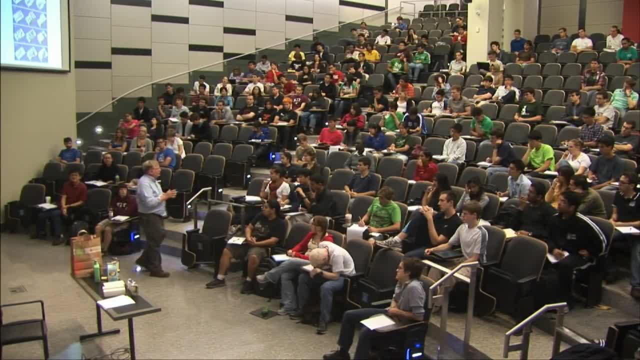 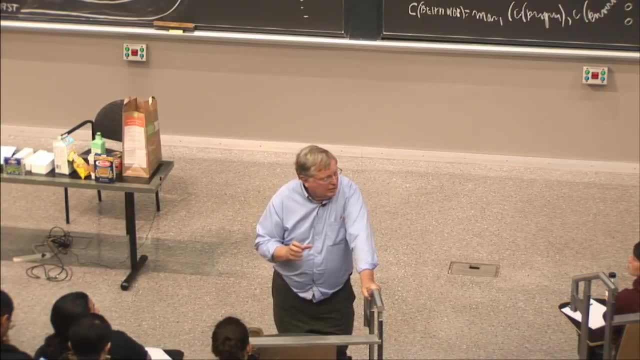 together in a little plastic bag. Actually, that's too complicated, But that's what we end up doing, right? Why do we put them all together in a little plastic bag? What's that? Well, there are two explanations. The MIT explanation. 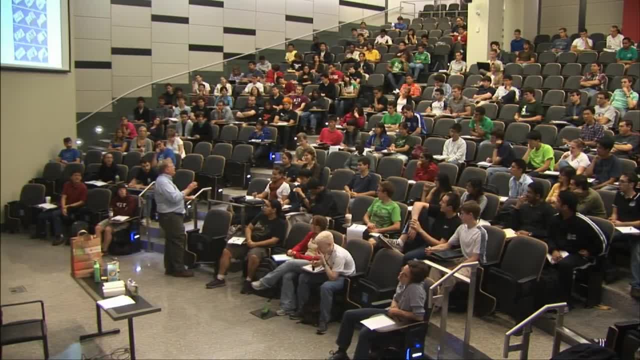 Ah, there's the MIT explanation. We know that That temperature flow is equal to the fourth power of the temperature difference and the surface area and all that kind of stuff. We want to get them all together in a ball sphere. The normal explanation is that they're going to melt anyway. 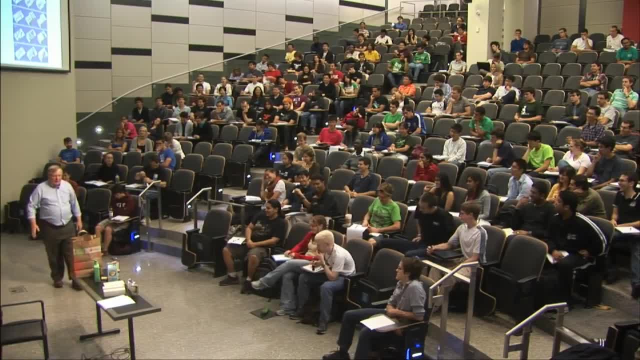 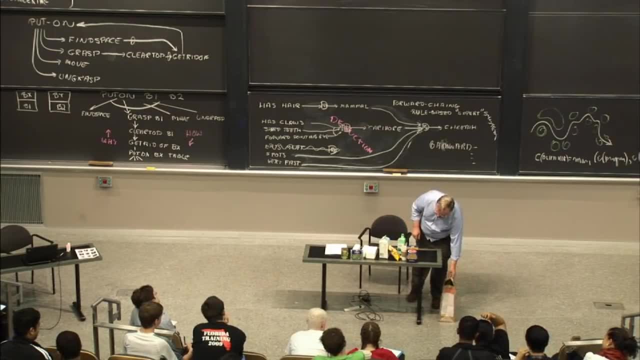 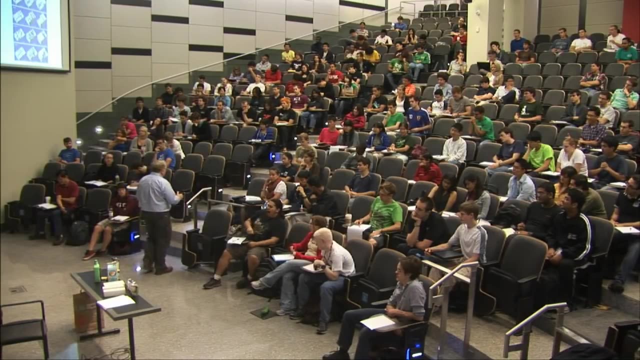 so they might as well not get everything else wet, All right. So that's heuristic number two. And actually there's heuristic number three that I just want to relate to you for the first time, Because I have been dealing with it a lot. 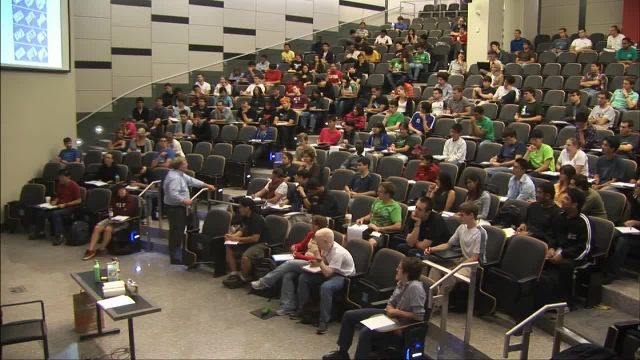 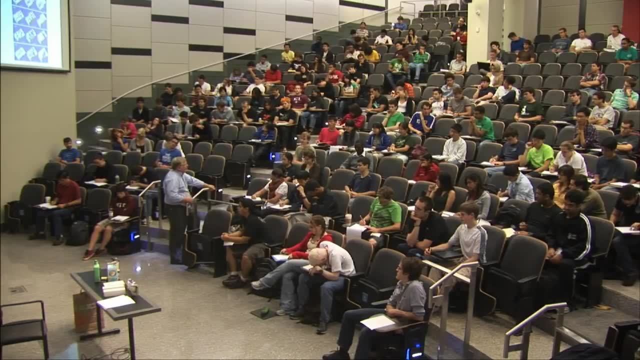 over this past summer. Heuristic number three is: you build a system and you see when it cracks. And when it cracks is when you don't have one of the rules you need in order to execute, in order to get the program to execute as you want it to execute. 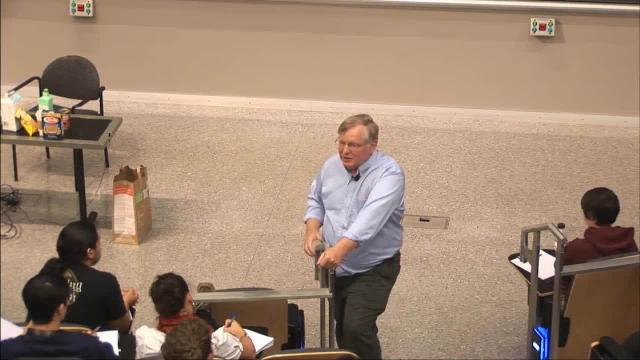 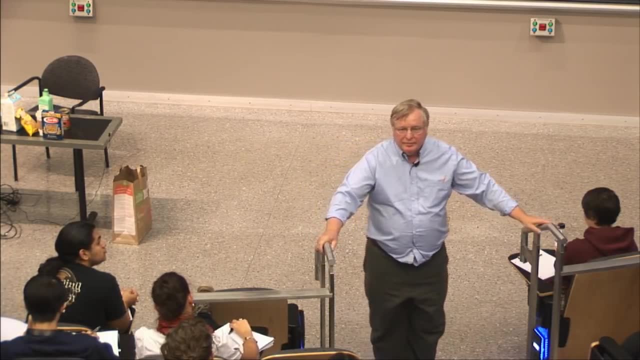 So if I were to write a grocery store bagging program and have it bag some groceries eventually, it would either make a mistake or come to a grinding halt And bingo. I know that there's a heuristic rule, Isn't that what happens when you do a problem set and you 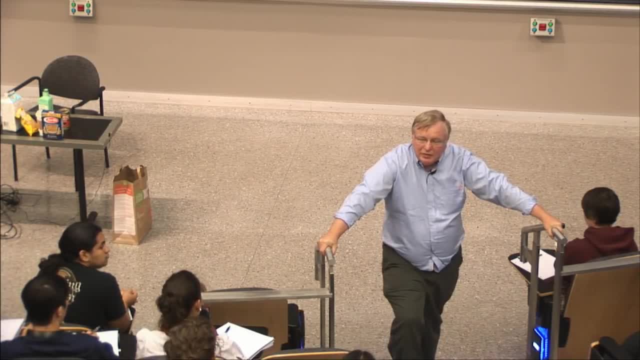 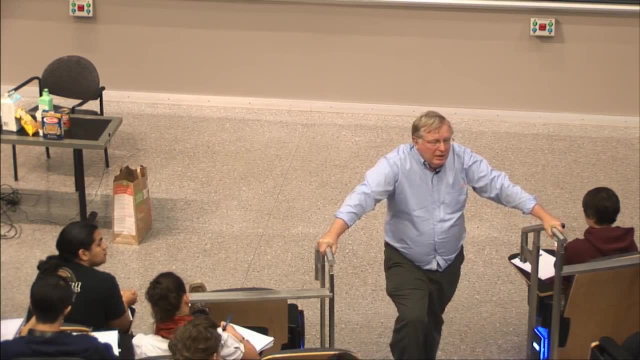 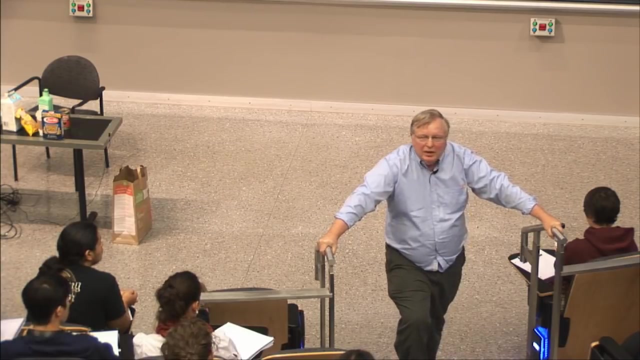 hit an impasse. You're performing an experiment on yourself and you're discovering that you don't have the whole program. In fact, I've listed this as a gold star idea- having to do with engineering yourself, because all of these things that you can do for knowledge, engineering, are things you can. 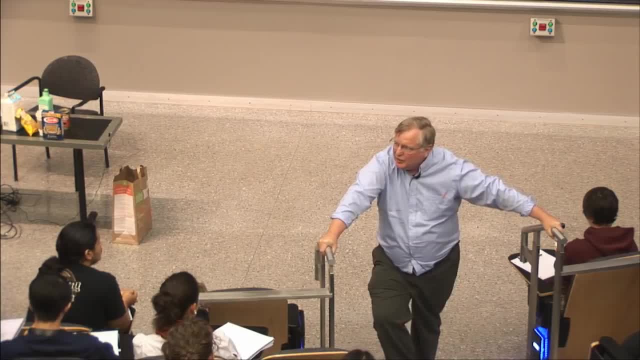 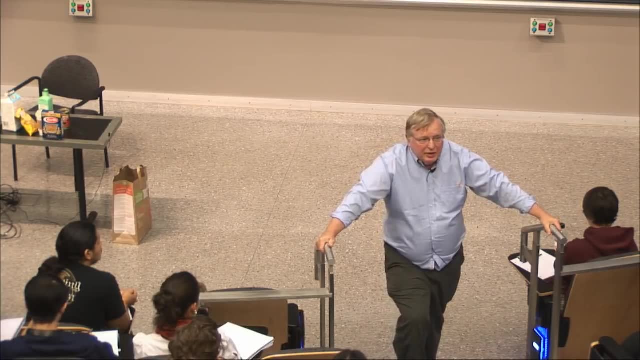 do when you learn a new subject yourself, Because essentially you're making yourself into an expert system. when you're learning circuit theory or electromagnetism or something like that Or something of that sort, You're saying to yourself: well, let's look at some. 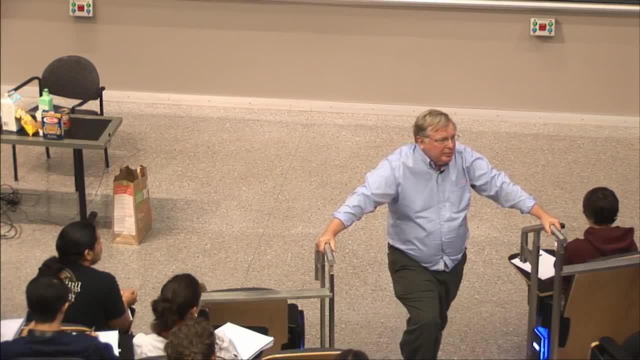 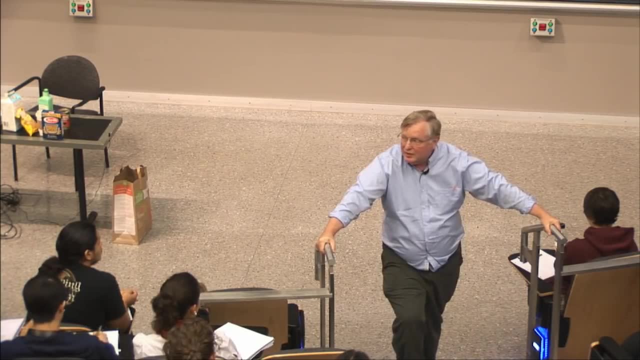 specific cases. Well, what are the vocabulary items here that tell me why this problem is different from that problem? Oh, this is a cylinder instead of a sphere. Or you're working a problem set and discover you can't work the problem and you need to get another chunk of. 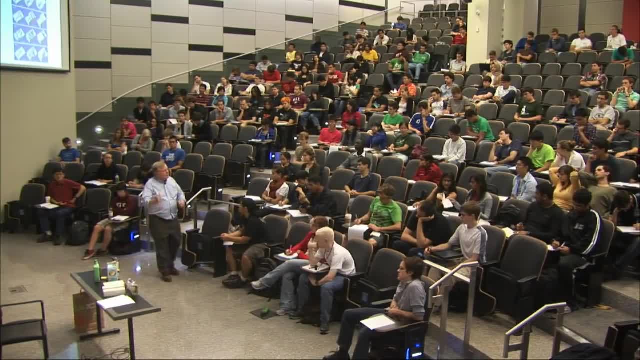 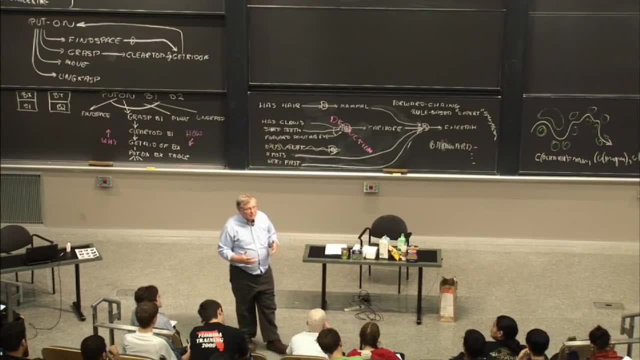 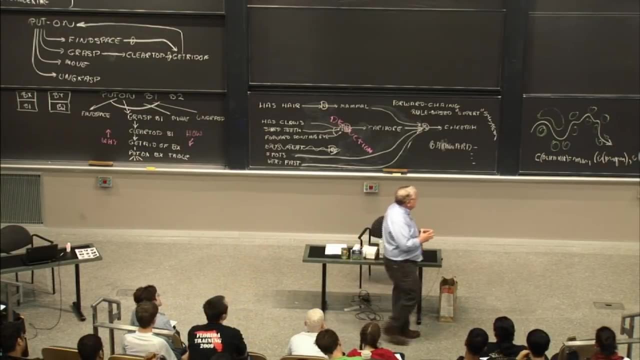 knowledge that makes it possible for you to do it. So this sort of thing, what you think of primarily as mechanism, heuristics for doing knowledge, engineering, are also mechanisms for making yourself smarter. So that concludes what I want to talk with you about today. 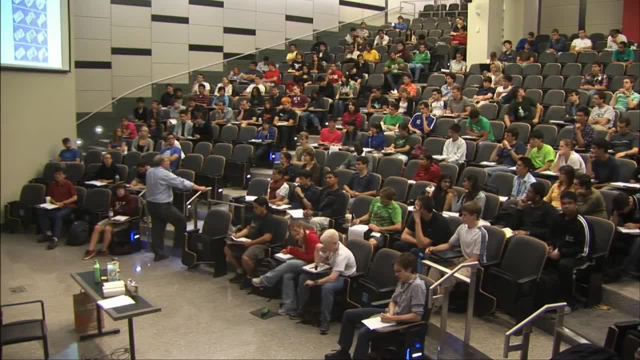 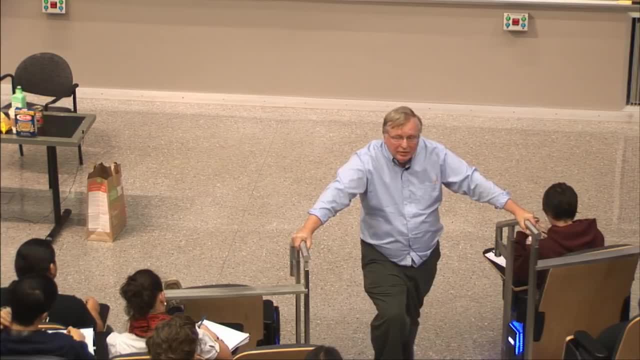 But the bottom line is that if you build a rule-based expert system, it can answer questions about its own behavior. If you build a program that's centered on goals, it can answer questions about its own behavior. If you build an integration program, it can answer. 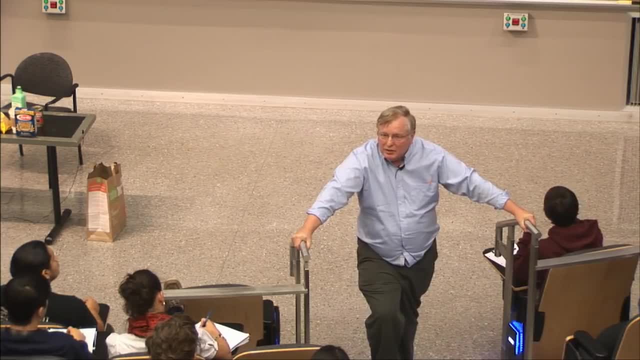 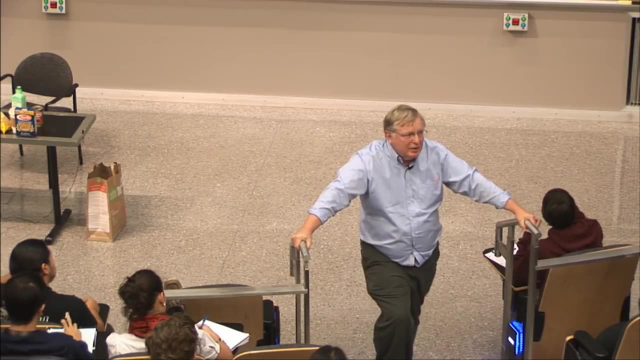 questions about its own behavior. And if you want to build one of these systems and you want to these systems and you need to extract knowledge from an expert, you need to approach it with these kinds of heuristics, because the expert won't think what to tell you. 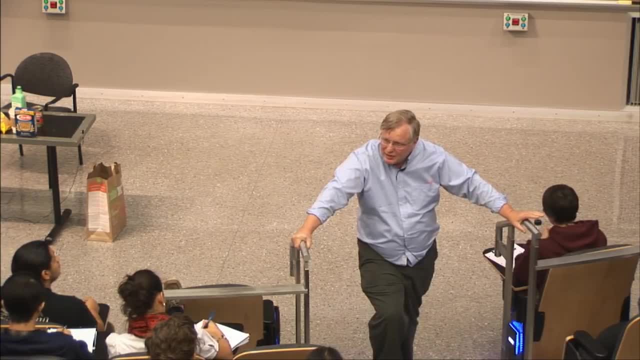 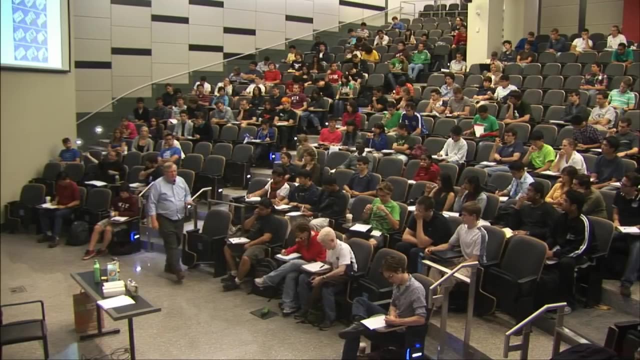 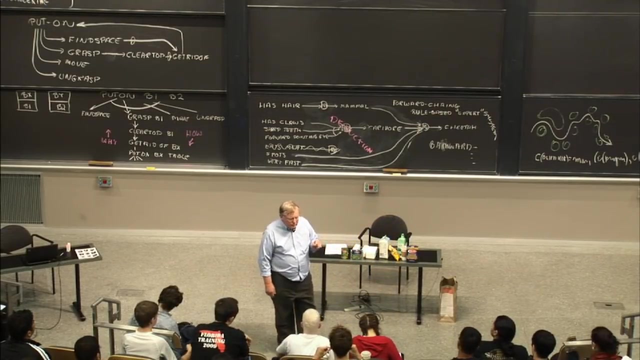 unless you elicit that information by specific cases, by asking questions about differences and by ultimately doing some experiments to see where your program is correct. So that really concludes what I had to say, except I want to ask the question: is this all we need to know about human? 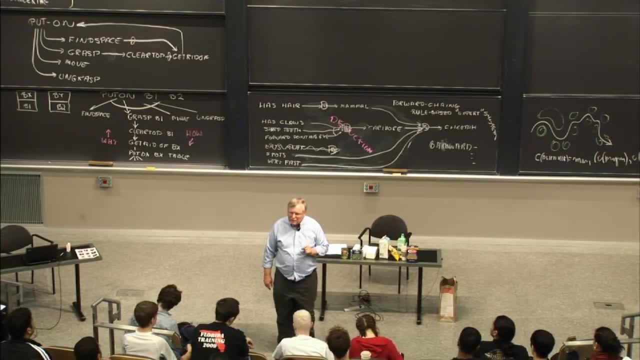 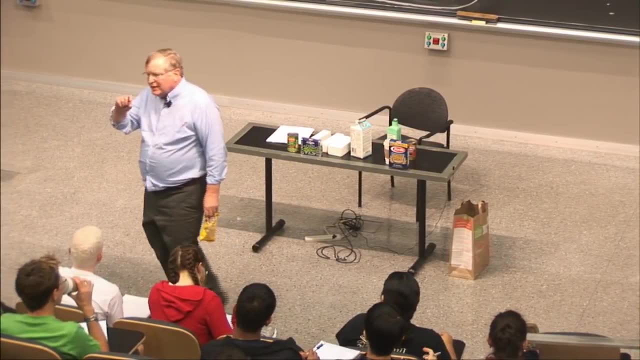 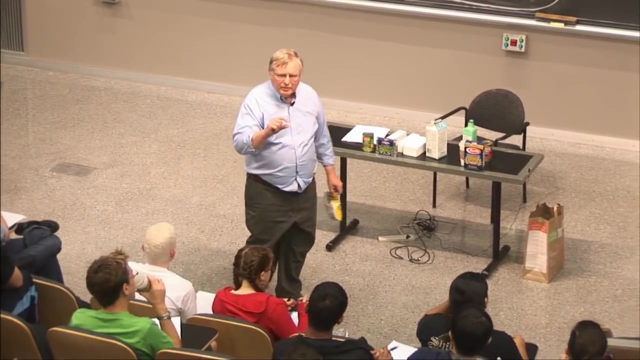 intelligence Can these things be? are these things really smart? And the traditional answer is no. they're not really smart because their intelligence is a sort of thin veneer And when you try to get underneath it, they tend to- as written, they tend to crack. 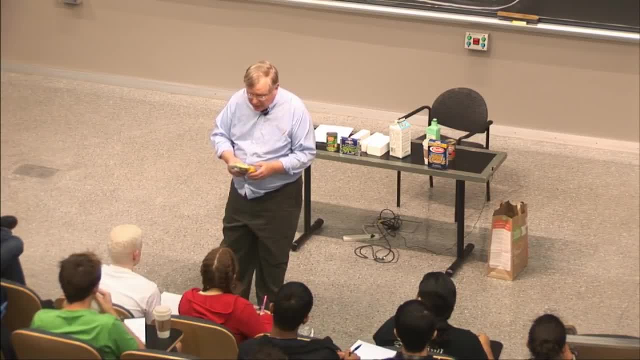 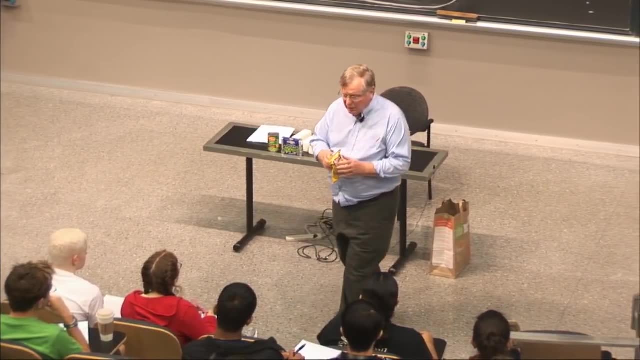 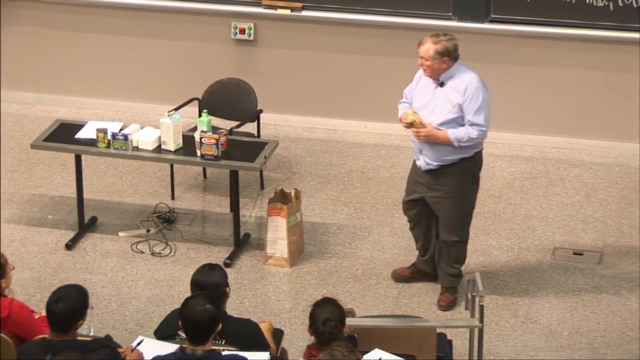 For example, we talked about a rule, or we could talk about a rule that knows that you should put the potato chips on the top of the bag, But a program that knows that would have no idea why you would want to put the potato chips on top of the bag. 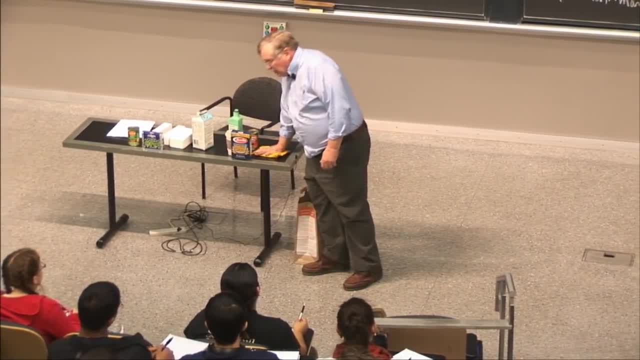 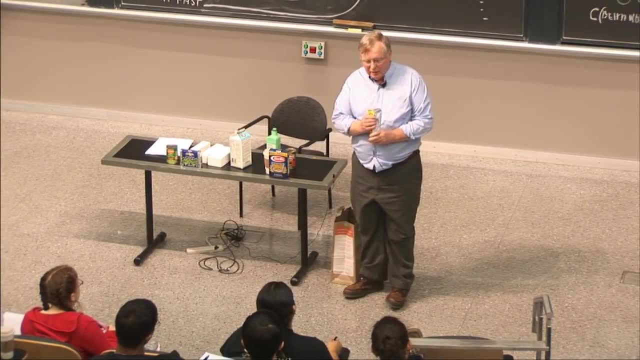 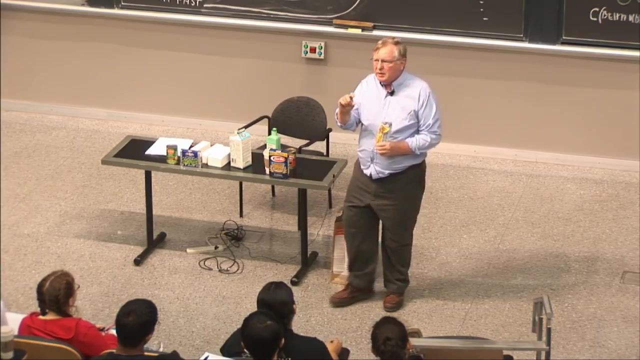 It wouldn't know that if you put them on the bottom of the bag, they'll get crushed. And it wouldn't know that if they get crushed, the customer will get angry because people don't like to eat crushed potato chips. So that's what I mean when I say the knowledge of these. 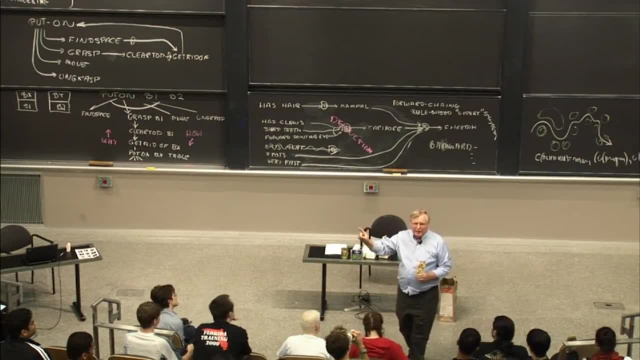 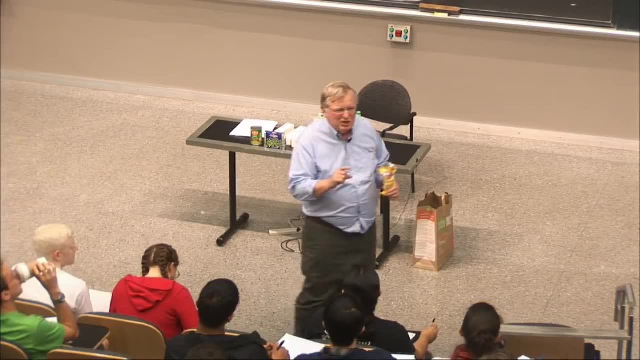 things tends to be a veneer. So the MISEN program during D-Business is a program that does that. For example, if you're driving to a shop in the ass and you get some test results for your test, there's a test result. 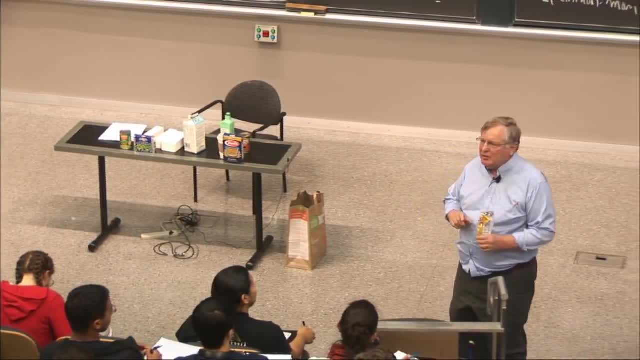 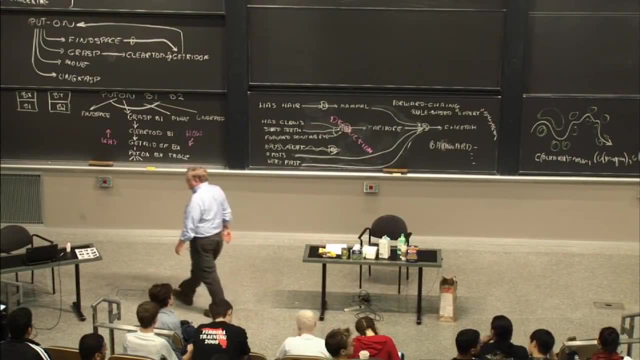 that says that you might be on the wrong way, that you might be on the wrong path. So the medical examiner is going to say: how is the test result? How is it going? How is it going? How is the test result going? 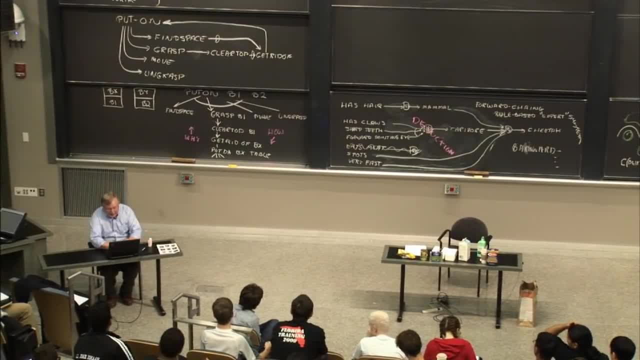 And the test result is going to tell you, And that test results is going to be a health test. You can find that on the equipment and on the book, but it doesn't necessarily predict a health, Because there are certain indications, there are certain 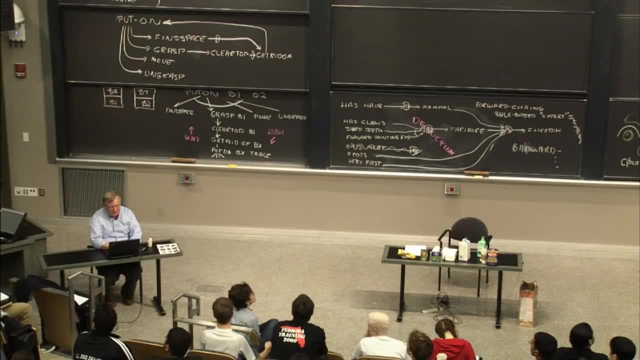 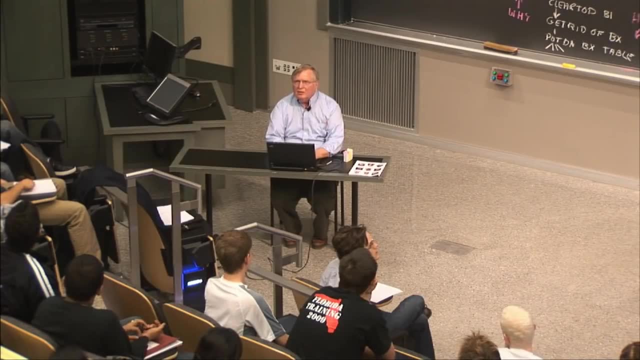 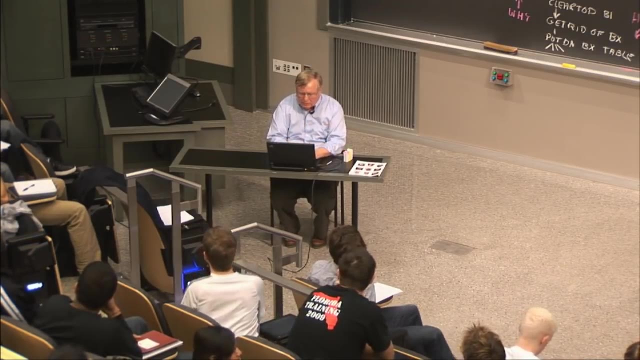 situations in which rules could be said to play a role in our ordinary understanding of things. Would you like to see a demonstration What I'm going to show you when Eclipse boots up? well, before I make any promises, let me see if I'm actually. 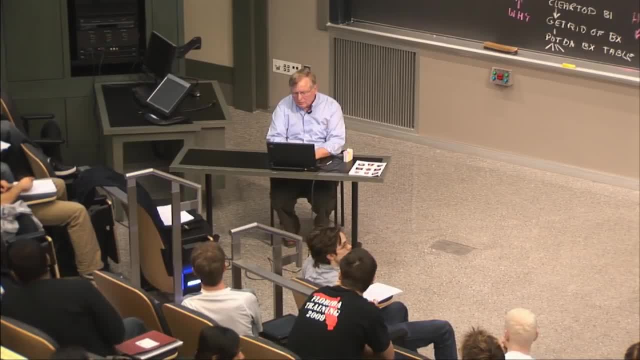 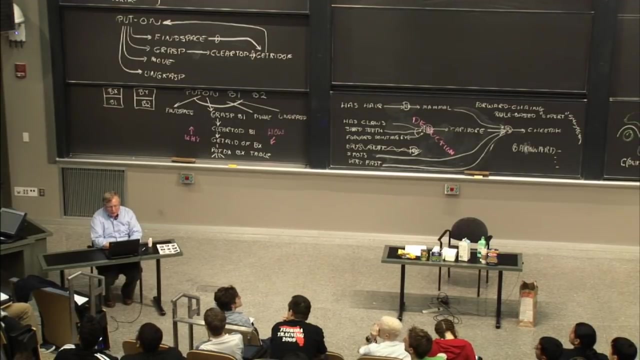 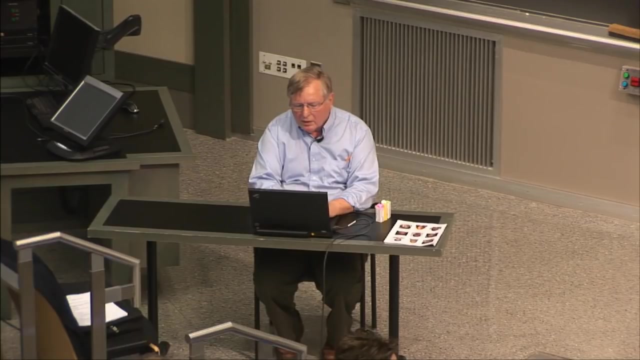 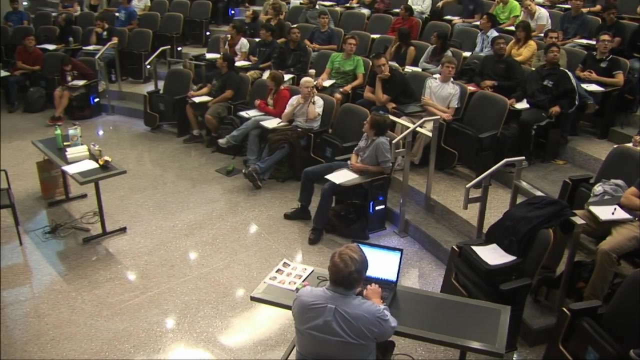 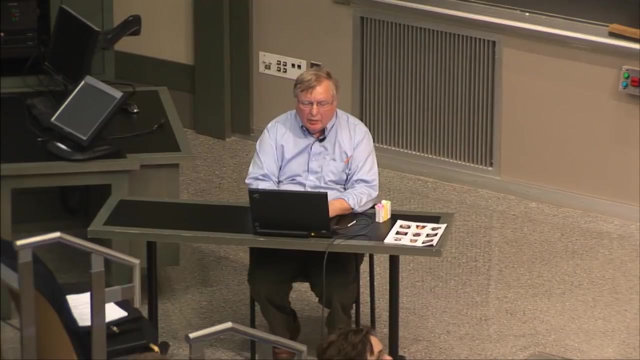 connected to the web. MIT good, MIT guest. yeah, that's me sounds good. OK, I just tested the system And I've seen that it is actually connected to the web. Now I'm going to adjust some systems options here. 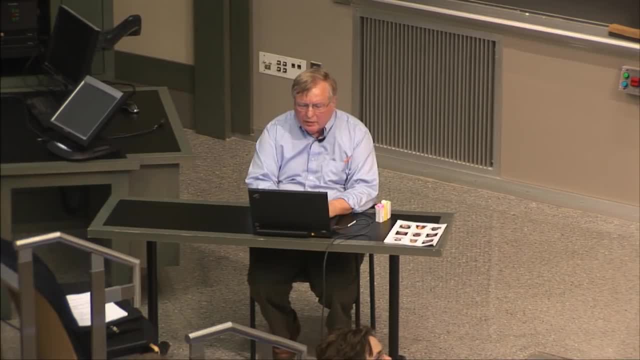 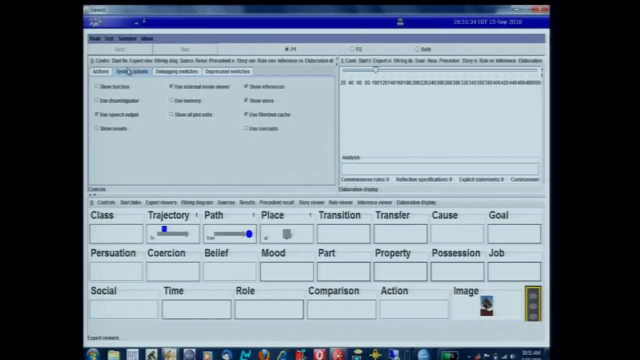 We'll get rid of the text box And we'll get rid of this or change its scale a little bit, And then what I'm going to do is I'm going to read a little synopsis of the Macbeth plot. Now, you're MIT students, I'm sure you're all classically. 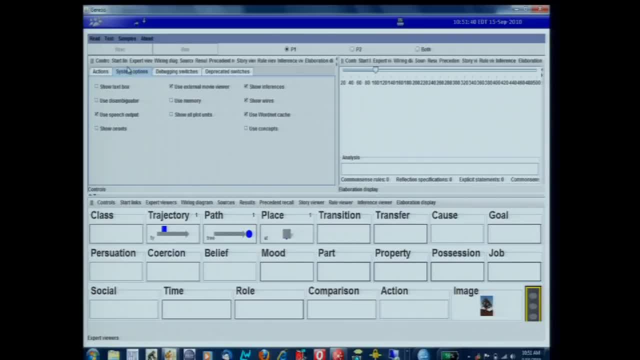 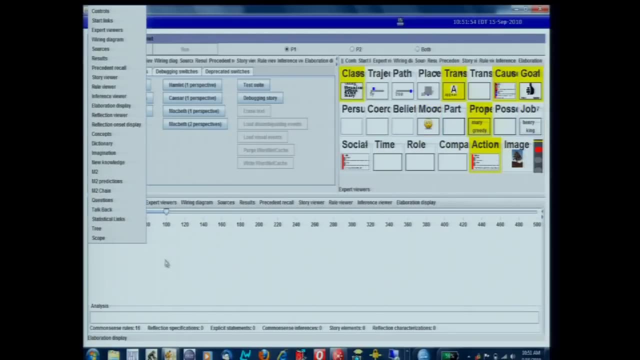 educated and very familiar with Shakespearean plots, So I'm going to read one. I'm going to read a version of a Macbeth plot And it's going to go along like this: It's basically reading a rule base so far, And pretty soon it's going to get beyond the rule base and 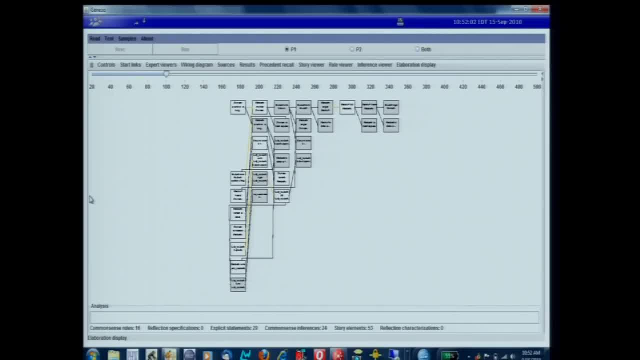 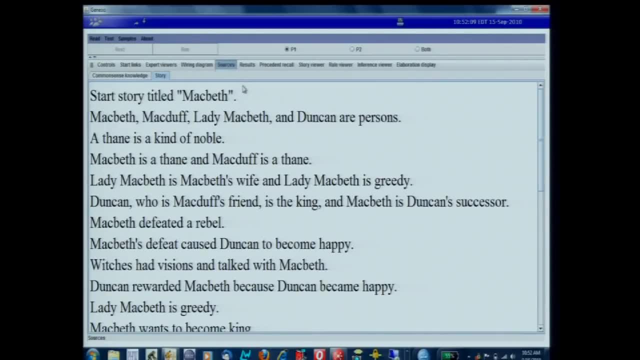 start reading the Macbeth story. And there it is. It's read the Macbeth story. Let me show you what the Macbeth story looks like as it's actually retained by the system. That's it. You can read that. OK, you ran out of time because the machine's already. 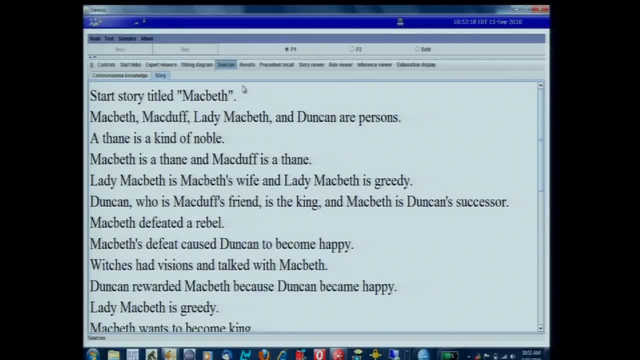 finished. It takes about five seconds to read the story. Now, as you look at this little synopsis of Macbeth, there are a couple of things to note. For one thing, it says that Duncan is murdered. Duncan, I hope this doesn't bother you. 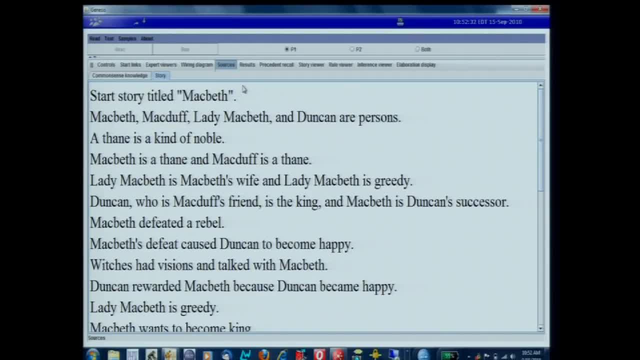 Duncan is murdered by Macbeth, But at no time does it say that Duncan is dead. But you know Duncan's dead because he was murdered. So you can see that he's dead And that's it. That's it. If murdered, then dead. 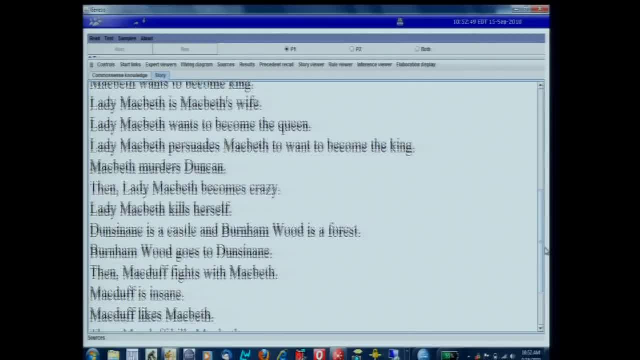 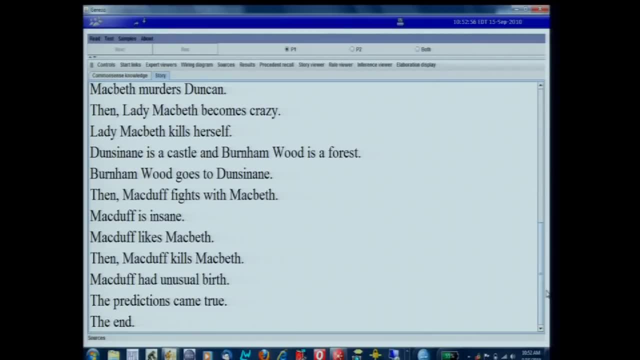 So if you look a little further down, what you see is that Macduff kills Macbeth, fourth line up from the bottom. Why did Macduff kill Macbeth? It doesn't say why in the story, but you have no trouble figuring out. 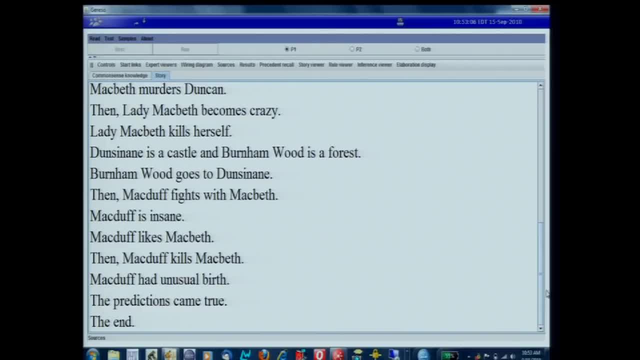 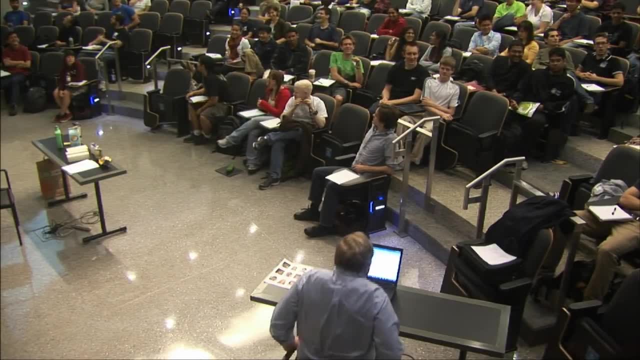 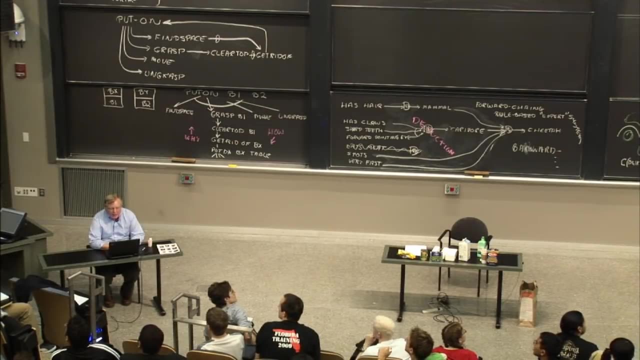 that it's because he got angry. And when you get angry you don't necessarily kill somebody, but it's possible. So now that you see what's in the story, let me take you back to this display. It's what we call an elaboration graph. 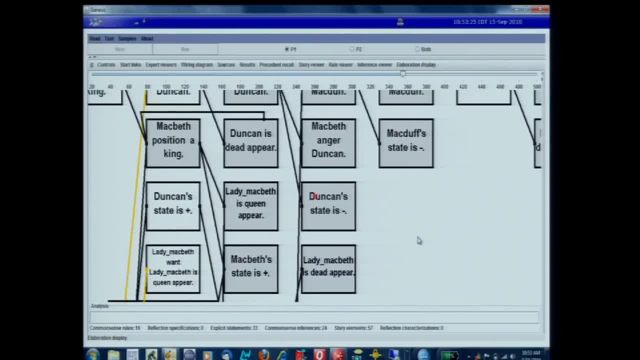 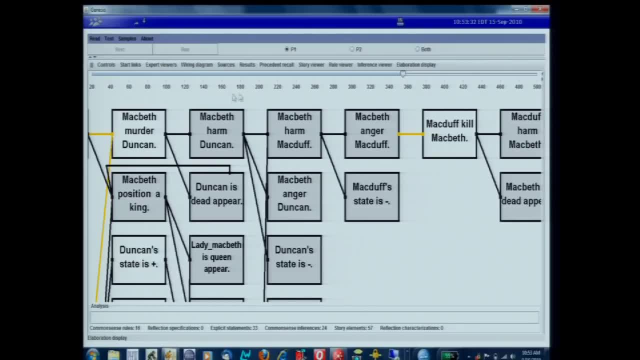 And when I blow it up you can see that there's some familiar-looking things in there. For example, up here in the left-hand corner, Macbeth murders Duncan, right over there And over here Macduff kills Macbeth. 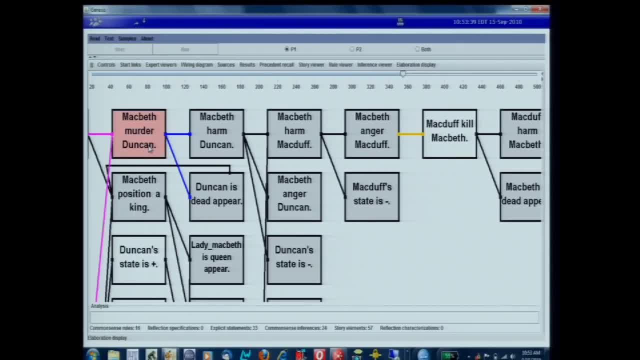 And if you look at what is a consequence of that, it looks like there must be a rule that says: if you murder somebody, you harm them, And if you murder somebody then they're dead. And one reason why you might kill somebody. is because they angered you. And if you go the other way, one consequence of killing somebody is that you harm them and that they get and they die too. And if you harm somebody, they get angry and their state goes negative.